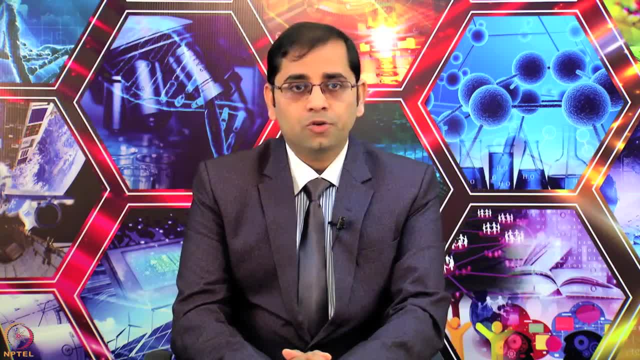 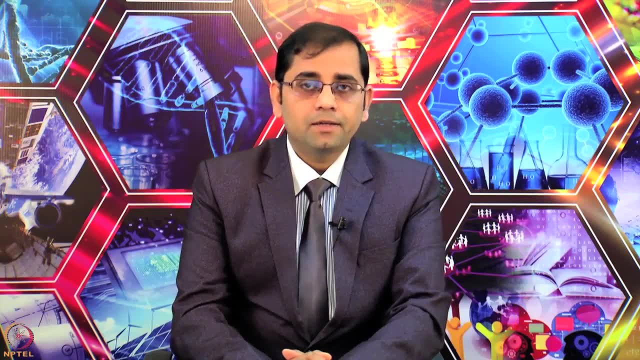 National Cancer Institute- NCI- National Institutes of Health in USA. Dr Rodriguez's research has focused on understanding mechanisms of cancer and age-related diseases, including development of molecular-based technologies. in basic translational and clinical sciences, Dr Henry Rodriguez has led to the development of NCI's clinical proteomics and genomics. 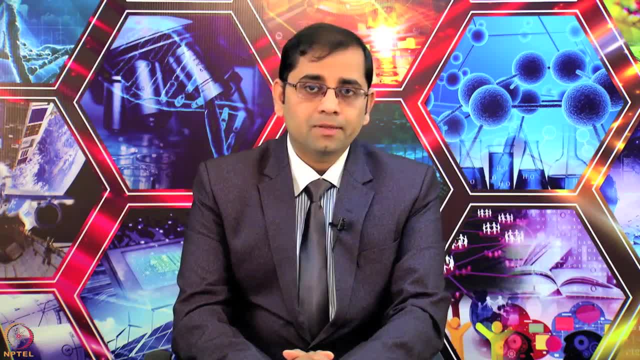 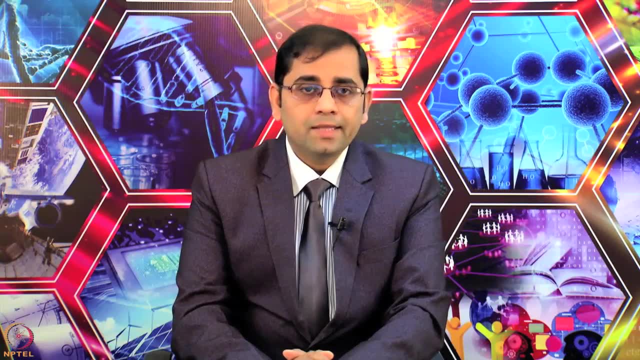 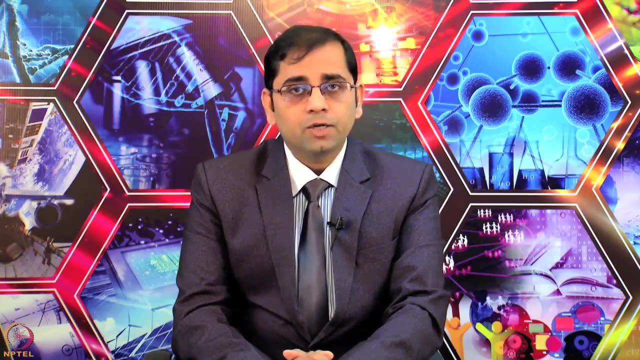 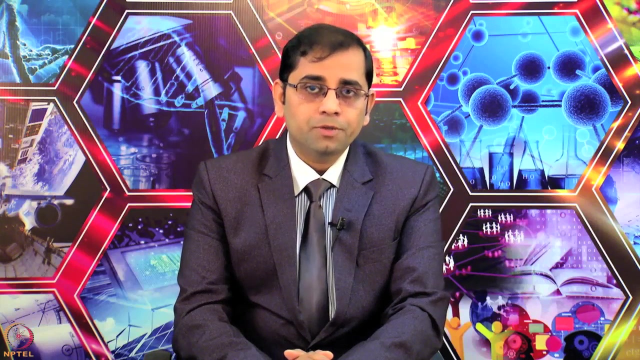 research program, which today includes the world's largest public repository of proteogenomic sequence data and targeted fit for purpose assays. His efforts have led to the formation of two cancer moonshine initiatives: The international cancer proteogenomic consortium, ICPC, and the 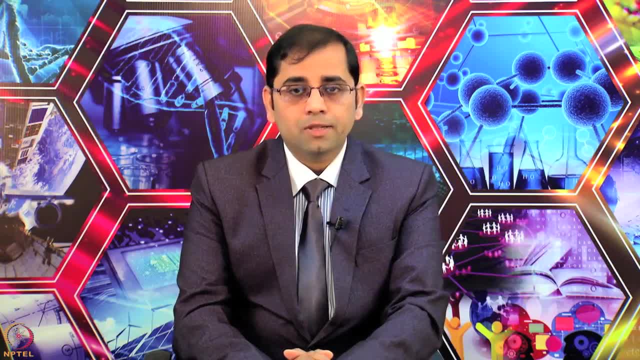 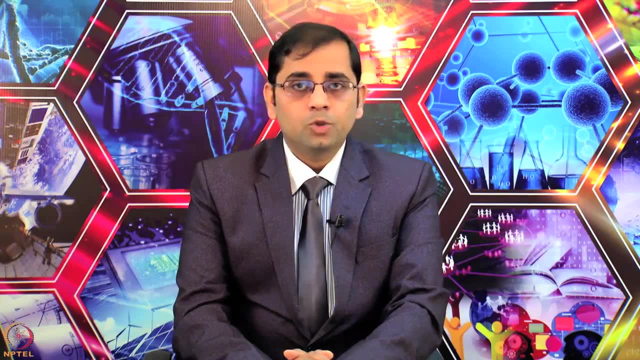 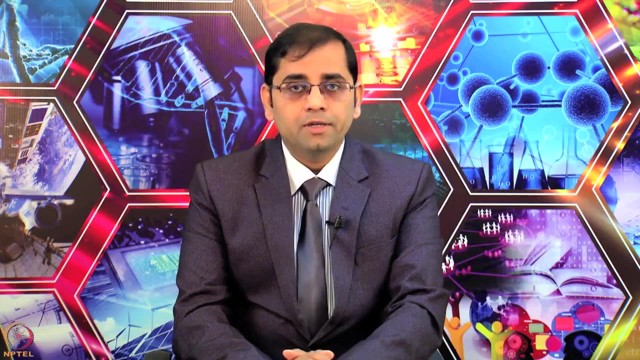 applied proteogenomics organizational learning online consortium. Dr Rodriguez's work showcased Organizational Learning and Outcomes Apollo Network, which he developed and co-developed. Dr Rodriguez has been very supportive to also include India as a part of ICPC initiative and India has now become the 12th country to join this consortium to look at the cancer. 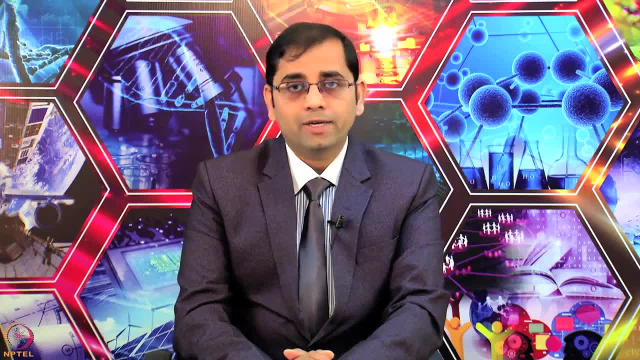 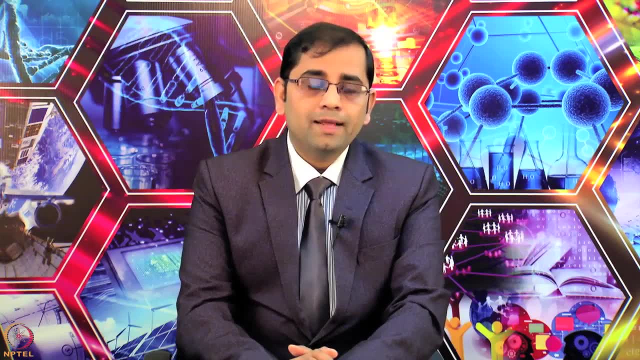 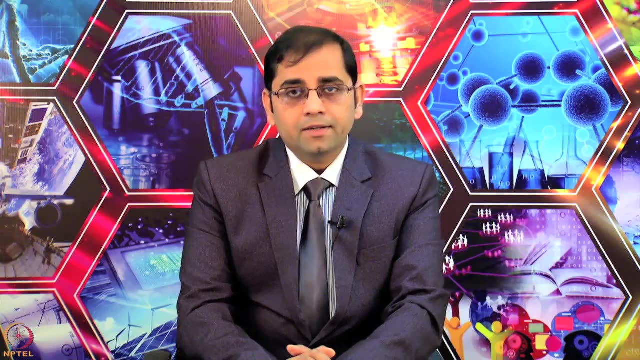 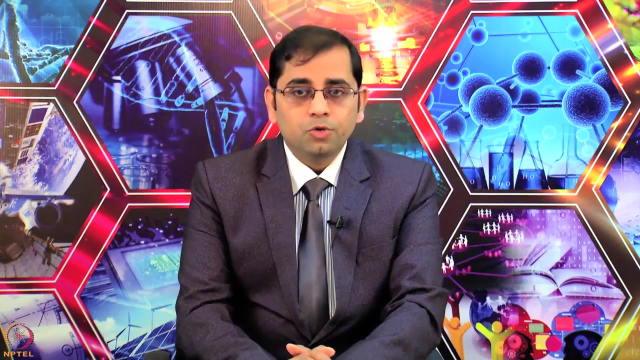 proteogenomics: research for cervical, breast and oral cancer. Dr Henry Rodriguez will give an overview talk of Clinical Proteomic Tumor Analysis Consortium, CPTAC, which is one of the efforts from NCI to accelerate the understanding of molecular basis of cancer through the applications of large scale genome proteome or proteogenomic. 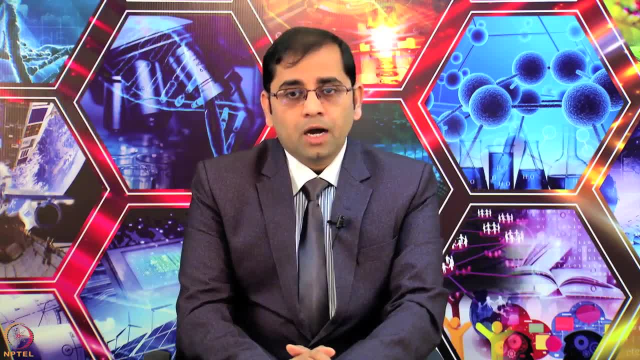 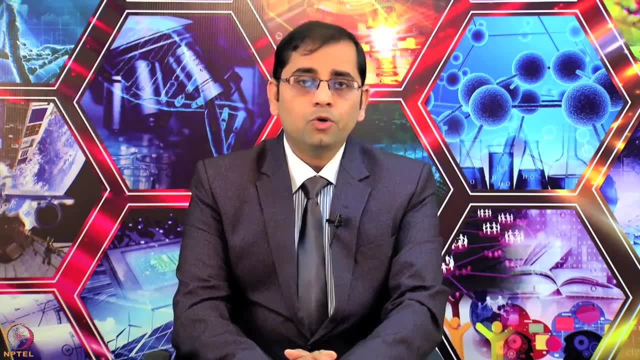 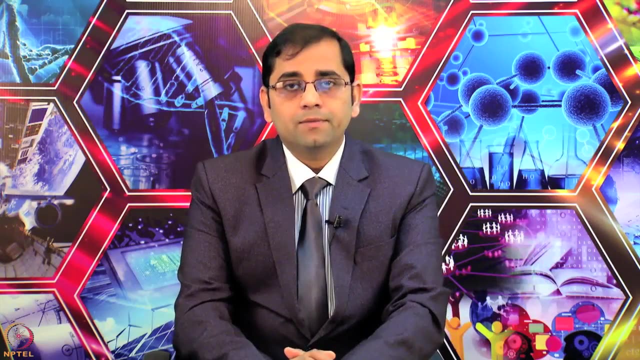 analysis. He will also brief about how NCI is working and taking the translational cancer research to the next step. Dr Rodriguez will talk to us about how genomics and proteomics together in the area of proteogenomics, could make much more meaningful impact. 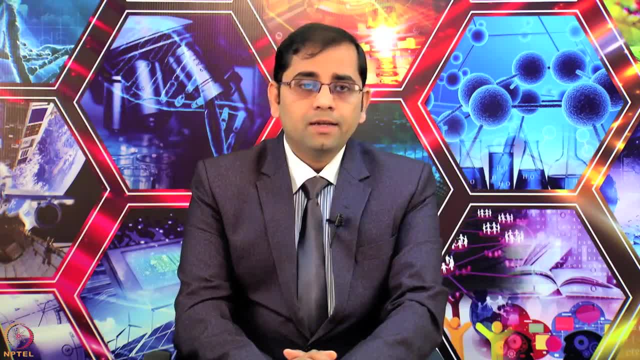 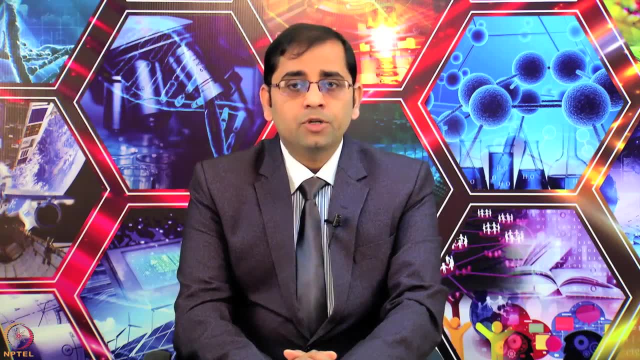 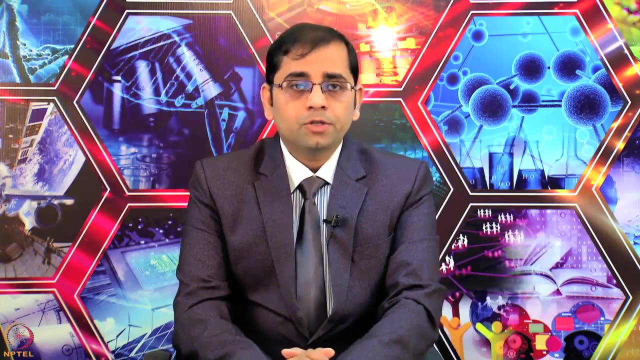 The importance of proteogenomics and how the robust field can reveal answer to different biological questions will be addressed. He will then bring various facts that laboratories worldwide should follow a standardized workflow to obtain repeatable results. Thank you, Dr Rodriguez will also talk about how proteogenomics is providing new prospects in recent projects. 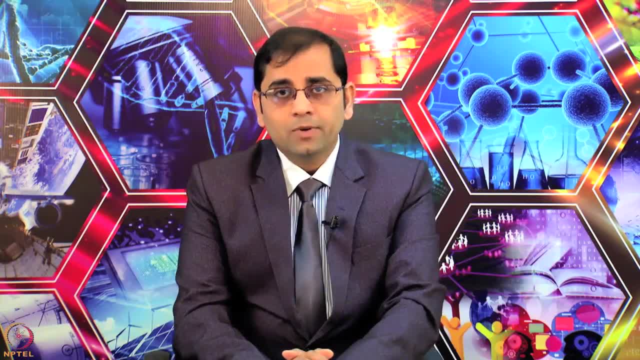 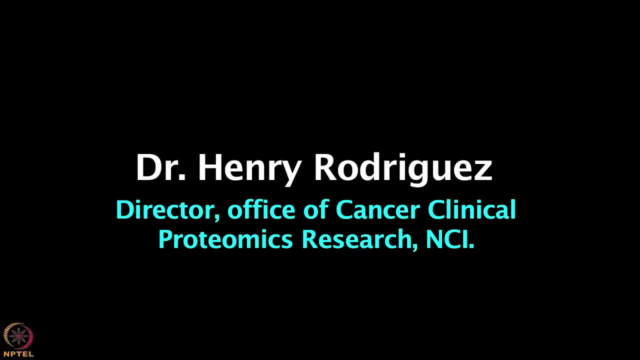 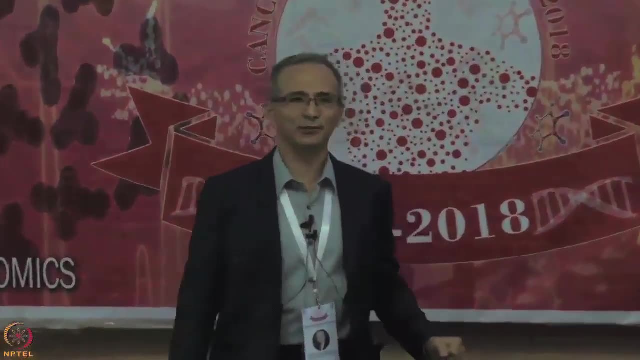 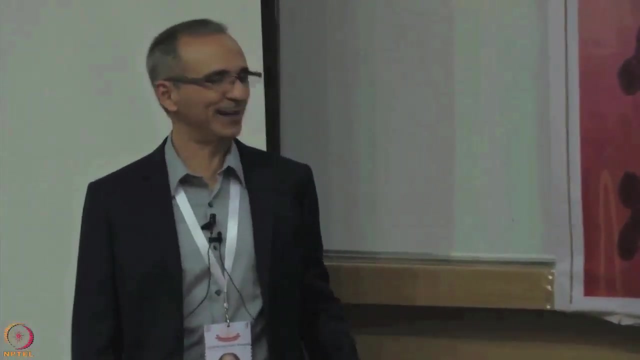 of CPTAC, like ovarian cancer. So let us welcome our distinguished colleague, Dr Henry Rodriguez, for his lecture. So welcome everyone. So my name is Henry Rodriguez. I am the Director for the National Cancer Institute's Office of Clinical Proteomics Research and I have to admit it has been extremely exciting and 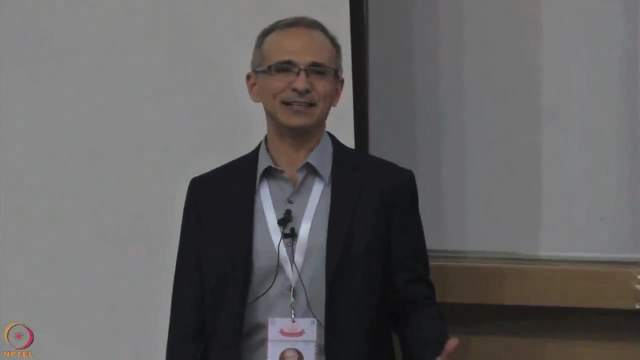 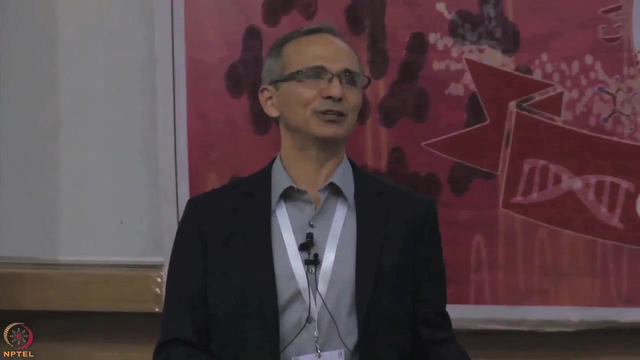 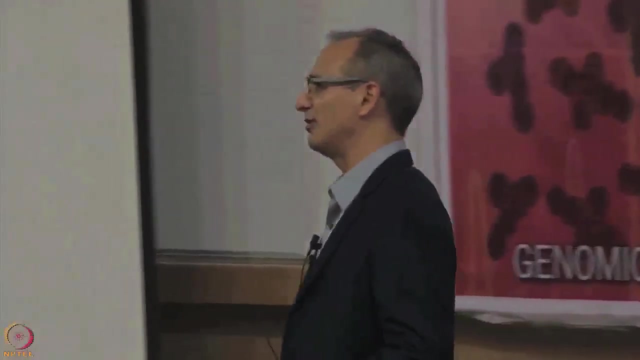 flattering, watching over the past several days, this idea of looking at the proteomics based information and trying to now blend it more and more with the rich history that has come out over the past 15 years in the genomics landscape. So what I thought that I would do is to give you sort of an overview of what we have been. 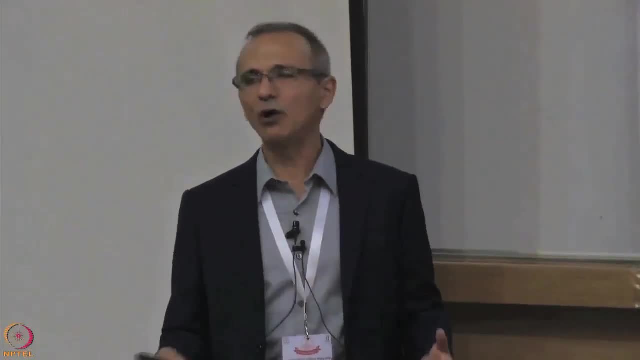 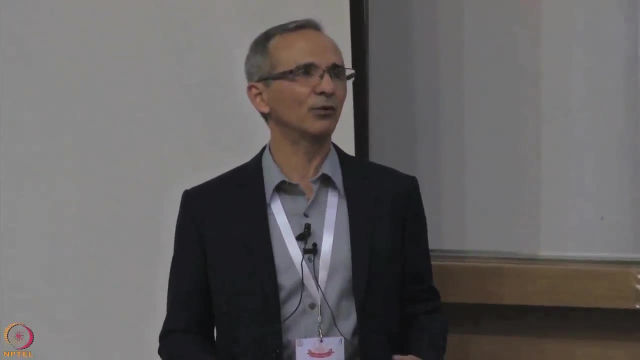 doing now at the National Cancer Institute really for about 12 years, where we see it going in the future For about another 10 years, and at the same time kind of talk about how we have taken what we have developed in the US through this program called CPTAC and now we have sort 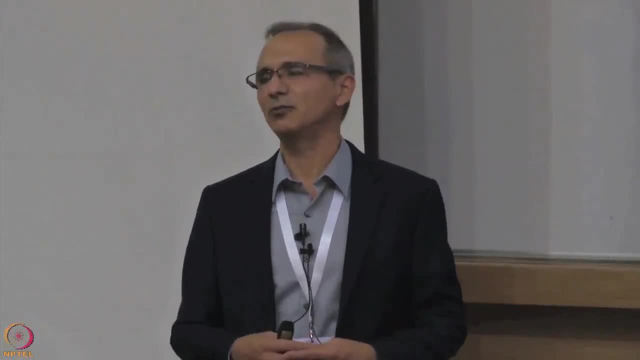 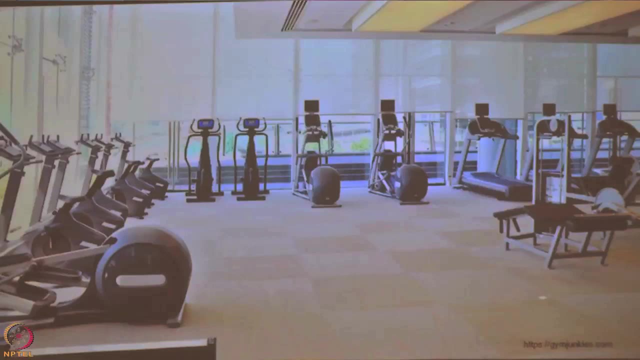 of expanded it, and it is really nice to see how India has become the latest partner within this international effort. So let me do this. the first slide that I am going to do is sort of a cartoon, because it was this one presentation that I saw two days ago and people were quite nice and they 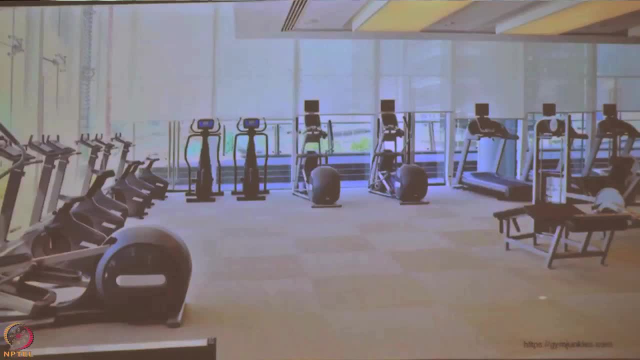 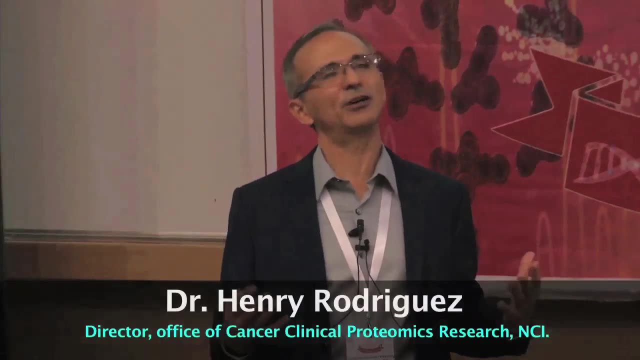 were very scientific And they explained to you genotype. they explained to you the genes. then they talked about phenotype. but here is my simplistic perspective of trying to understand a genotype and how it rolls up ultimately to a phenotype, which is what you want to get your hands on. 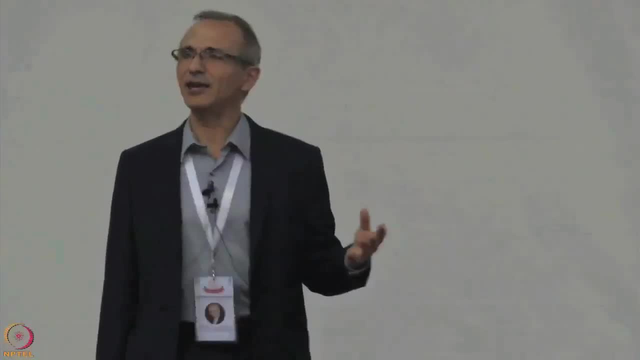 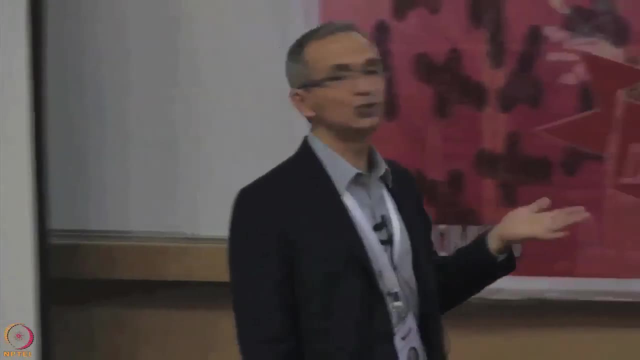 So imagine if you are at the gym. So in a way, if you want to look at what genotype is which is going to be representative of your genomes, this in way could actually be your genome, which is your genotype, which kind of tries to represent. it is your blueprint. 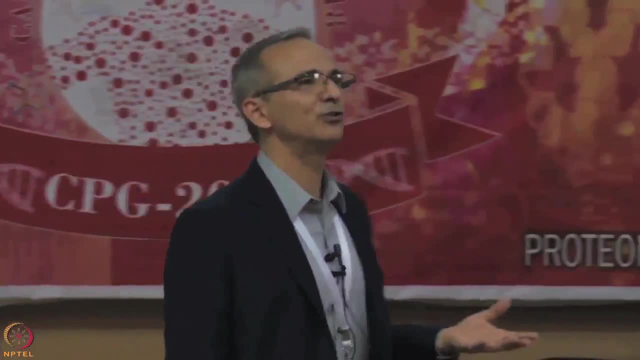 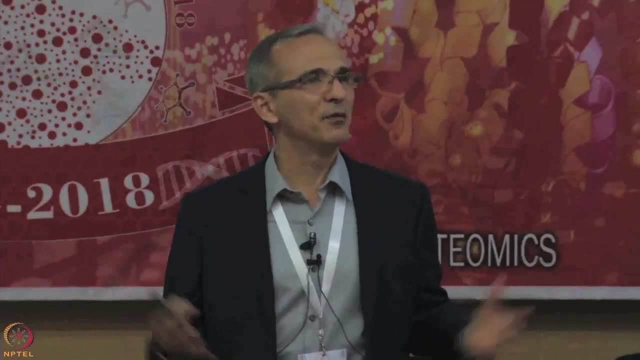 Right, And obviously, when you have a blueprint, what you are trying to do is to say: this is what I could potentially could become. that is your genotype. all the potential is there, but, as people know, we all aspire to do certain things, and sometimes those things actually. 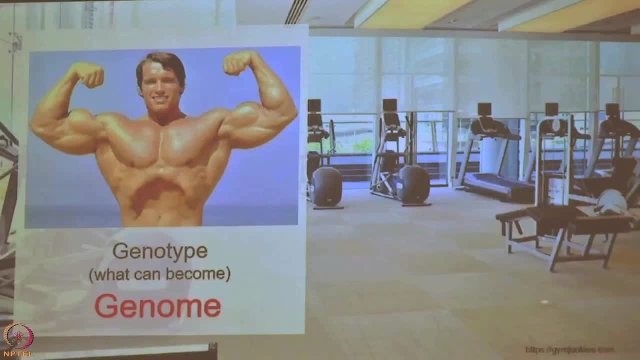 do not come to fruition. So the reality is your genotype, which is what you wish to become, as in this individual which is Arnold Schwarzenegger, the phenotype which is actually your functional space and you, and you can kind of look at it as your proteome. 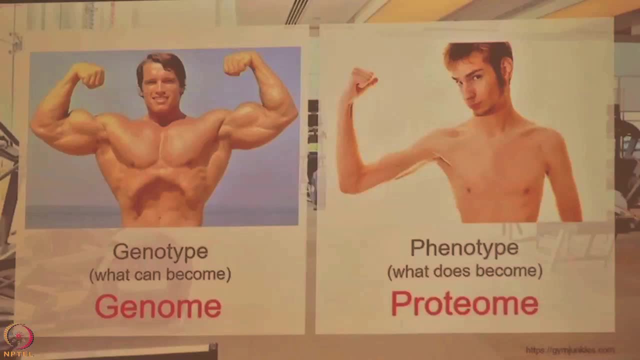 This could actually become your phenotype, So not always do you get what you want to put in a good way. however, though, that is actually ok, Because I think, ultimately, to understand the different states between the genotype and the phenotype, it becomes really important to begin to blend these worlds together. 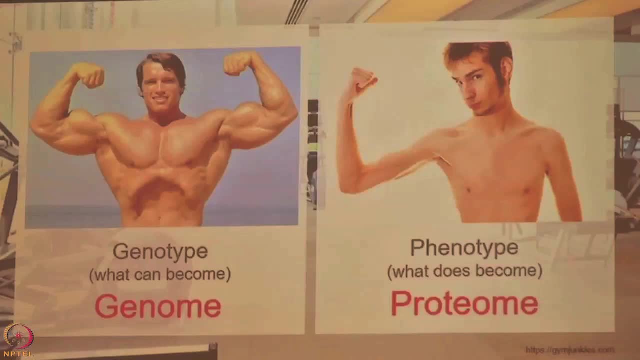 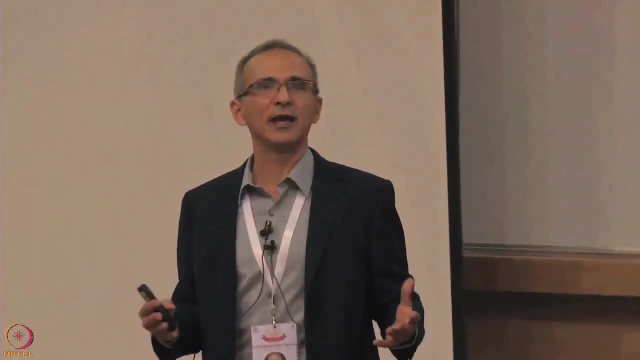 Quite frankly, I think if you study only the genome and then you ignore the proteome, or quite, if you look at the proteome, completely ignore the genome, you are going to be missing a tremendous amount of biology, And I hope in the next 40 minutes I could give you an example on how. now we have seen that. 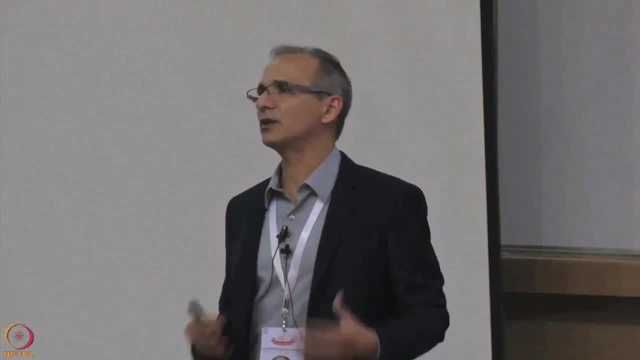 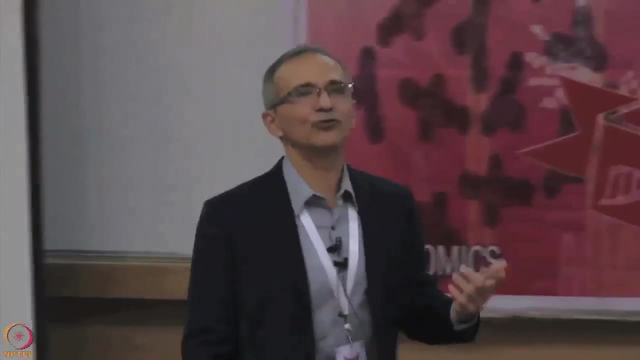 In the space of oncology that that is the case. So more and more, as technologies are becoming very mature, we are starting to blend these worlds together. So this is the history sort of the genome that I see it from the perspective of the 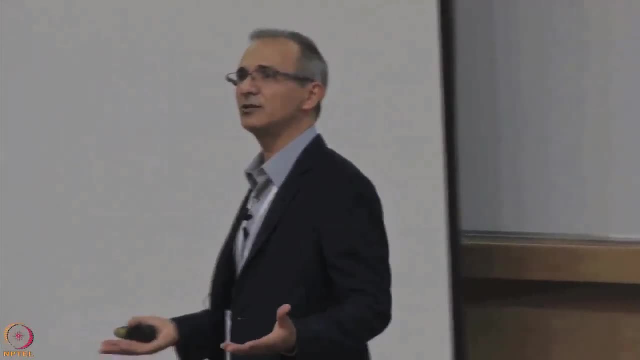 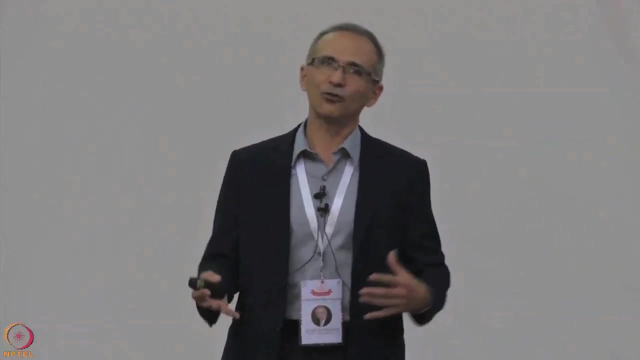 National Cancer Institute. So I actually got recruited to NCI just about 12 years ago and one of the things that I kind of liked about it is that I love organizations that enjoy taking risk. So for very conservative organization they kind of did take a risk politically because 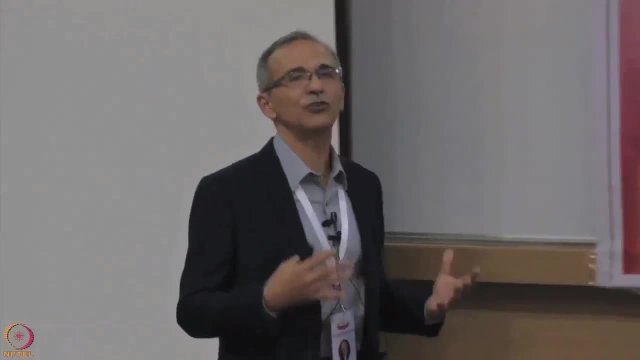 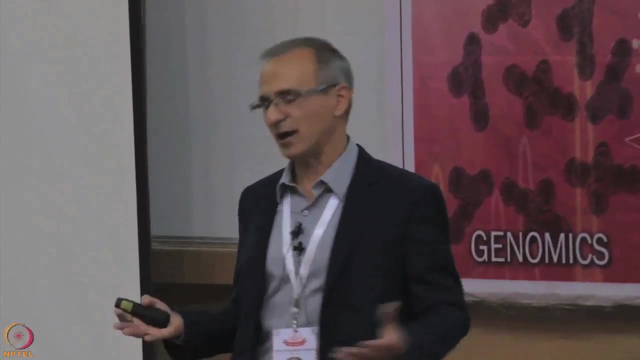 it did cost a lot of finances in the space of, in the space of omics based research, and if anyone talks about genomics, a lot of people will talk about the Cancer Genome Atlas. So the Cancer Genome Atlas actually gets officially launched in 2006.. 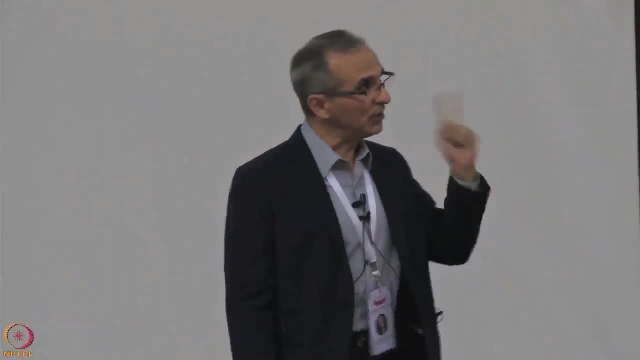 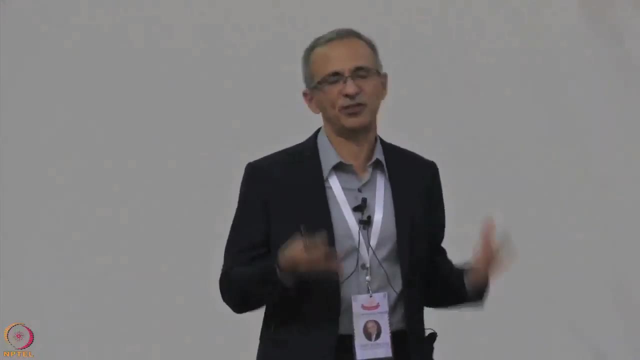 So the dates now become very important here, and TCGA in a span of 10 years. of course, they had a lot of capital to do this, but in a span of 10 years they did an amazing thing. They basically catalogued about 34 different cancer types. 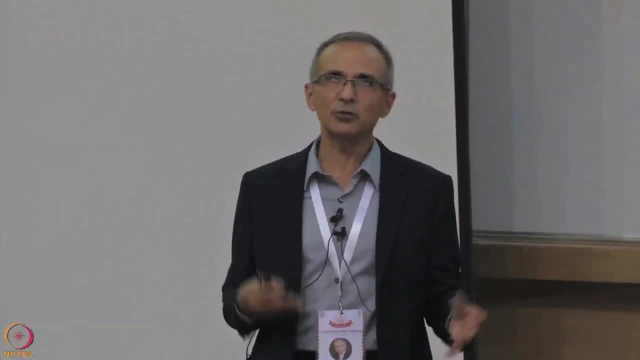 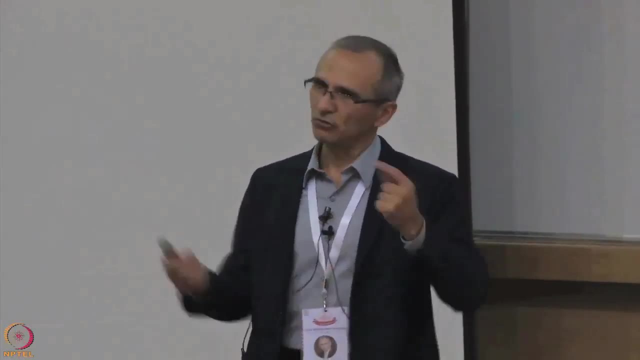 These are all solid tumors and they actually went through about just a little bit over 14,000 individuals to achieve that goal and all the information they placed it in the public domain. So that is good. Here is the part that a lot of people do not know about the history of NCI. actually, when 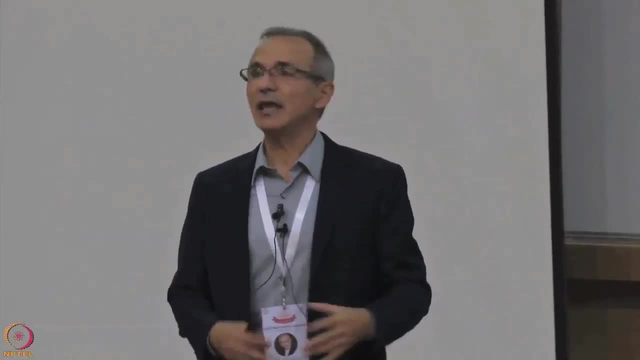 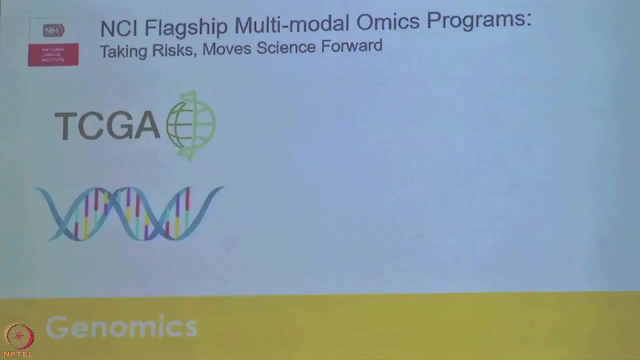 they were actually trying to come up with this idea. well, do we look at the genomics? they all along did not want to do genomics in isolation. They actually did want to go after the proteomics space and in that, and actually what they ended up doing was 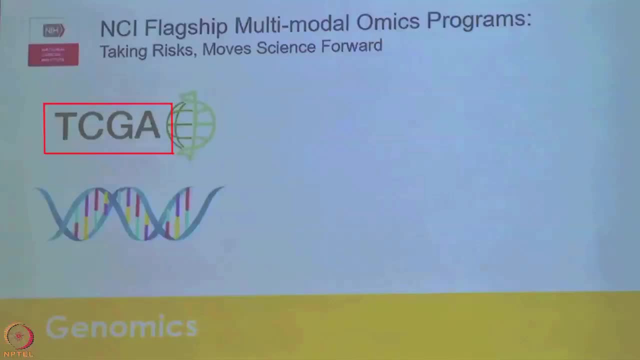 So at the same time that they launched the Cancer Genome Atlas, which was mandated to go after biology, they launched a proteomic based effort. Now, a lot of people knew about it, but that program at the time, which is now today kind of known as, is referred to as CPTAP. 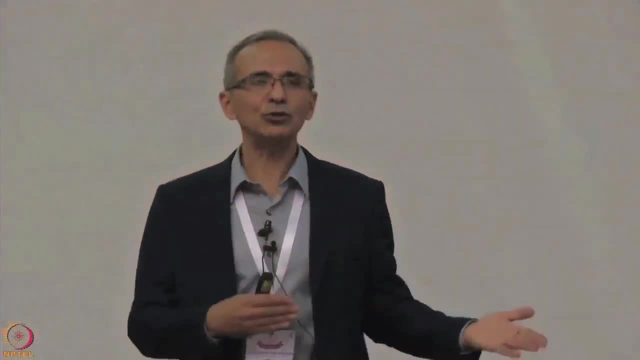 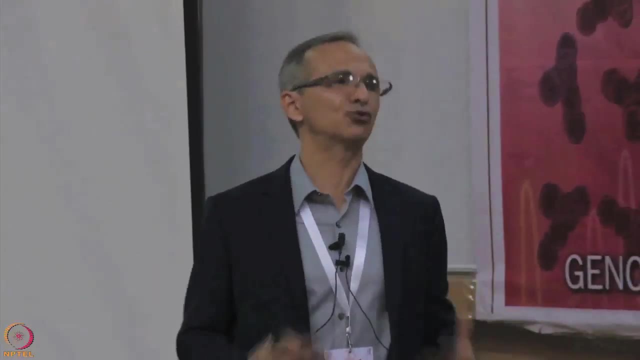 Now the reason they want to do it was quite simplistic. or in the early 2000s the first draft of the human genome project gets released. again, it is a draft, but that really raised the interest of a lot of oncologists in the US, especially our cancer center directors. 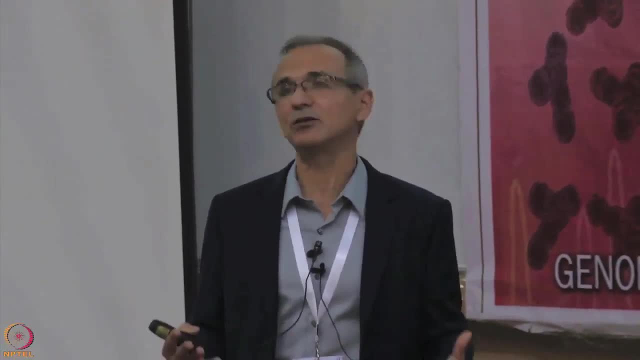 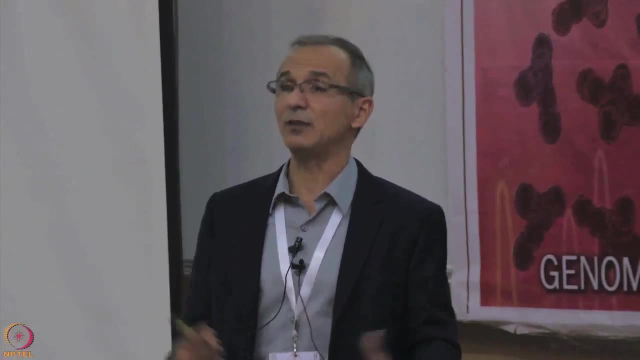 And they basically did these series Okay Of workshops and one of the things that came out of these workshops: they said we need to now begin to explore omic based technologies in cataloging different cancer types, and they made it very clear We want to go after genomics and proteomics. now, why proteomics? well, the first one. you 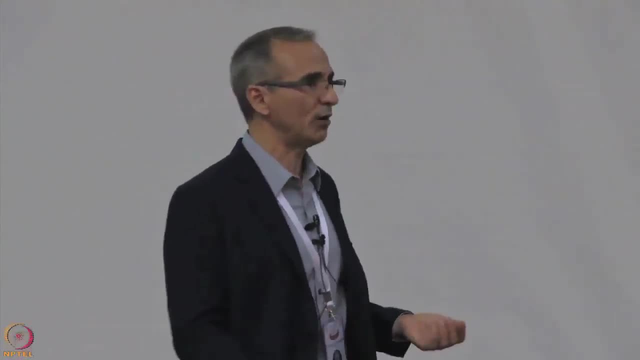 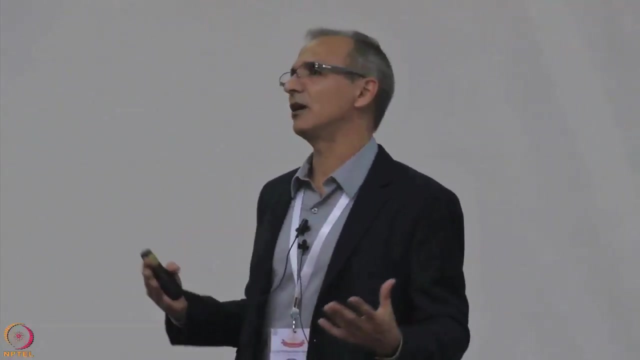 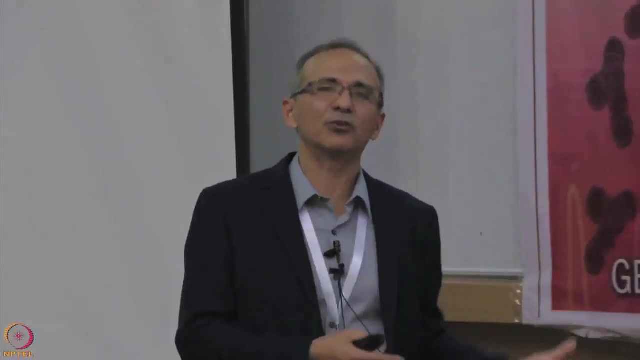 kind of would actually understand- which is what was talked about in the days prior- was you need to get an understanding of the underlying biology of a disease? and if you talk about biology, trying to understand the different pathways and not just taking your RNA-seq data and computationally predicting, from a bioinformatics perspective, what the abundance? 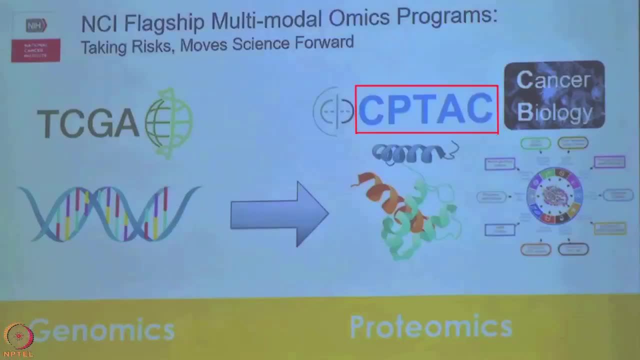 are proteins or, more specifically, what those modifications would be. it is never a one to one correlation, So they knew they had to understand the underlying biology before any of the biology could even move potentially towards patient care. The other reason was is exactly what I said: patient care if you ignore the space of IO. 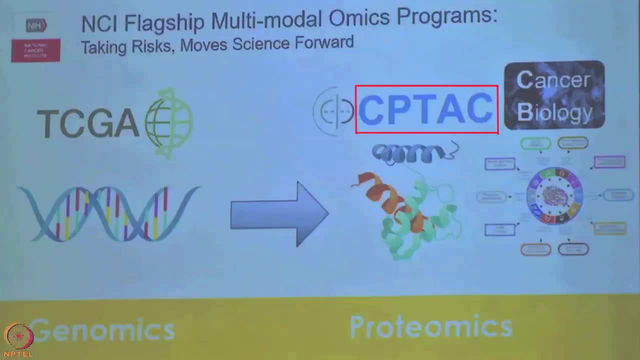 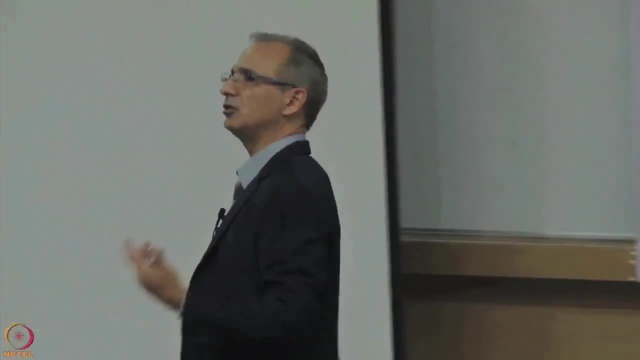 which is a immuno-oncology. the vast majority of all our patients are still being treated with compounds. These compounds that are typically chemo based, and those compounds actually do not target- in fact, the vast majority of them do not target- DNA. there is very few that play this idea. 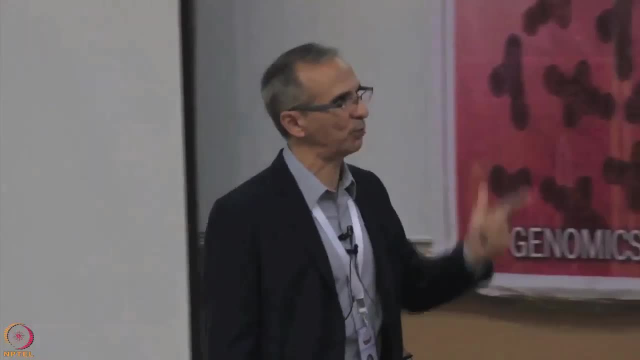 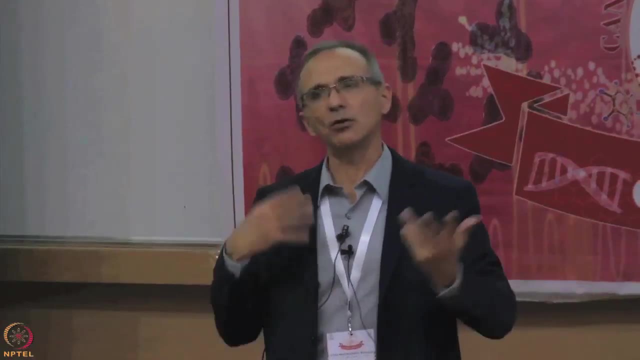 of intercalating the DNA. the vast majority will always go after a protein. So they need to understand, not just hey, my target binds here, but again trying to understand off target sites and all the wiring of the biology and all the off-roads that you could. 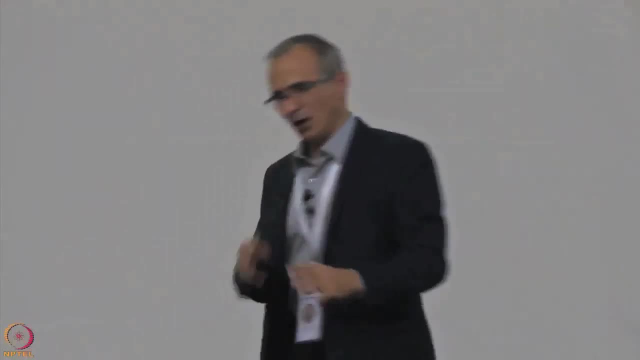 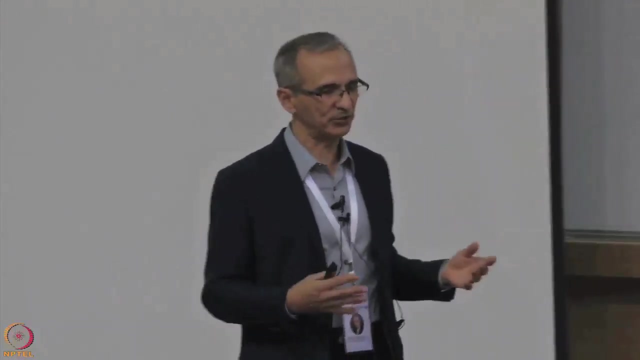 get. But here is now what happens around 2003 using the instrument of a mass spectrometer. So this is what happens. So a mass spectrometer, a publication gets released into the public and that actually looks at early stage ovarian cancer. 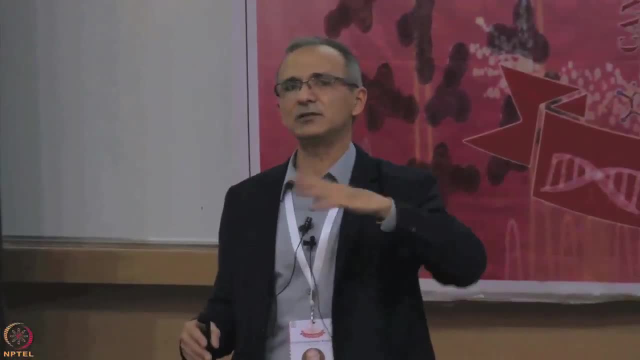 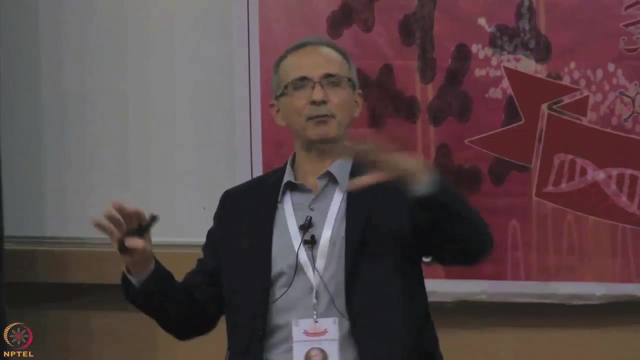 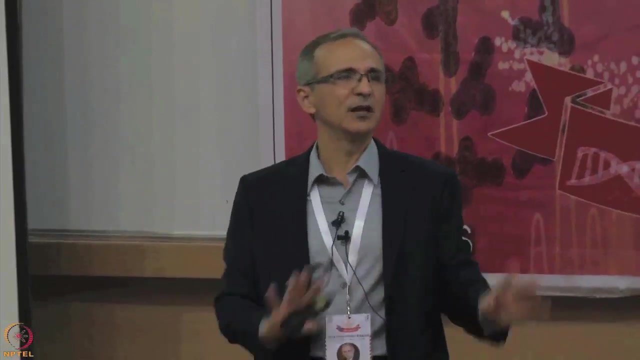 They actually did not identify the proteins that they were measuring. they basically looked at these pattern recognitions and, based upon that, they basically argue that simply looking at proteins by a pattern, ignoring the genomics information, we are able to identify early stage ovarian cancer. and I think they talked about like 90 percent specificity with a 99. 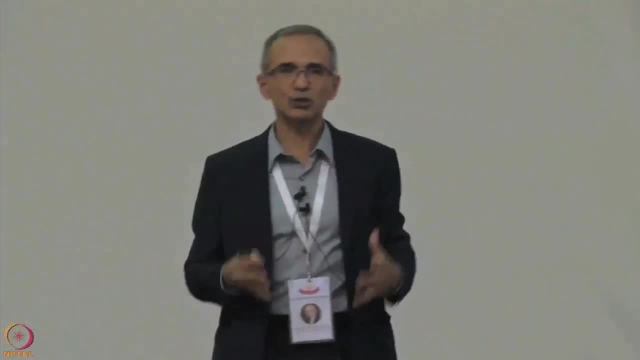 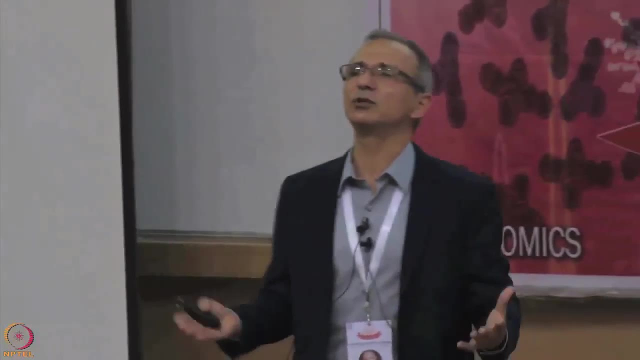 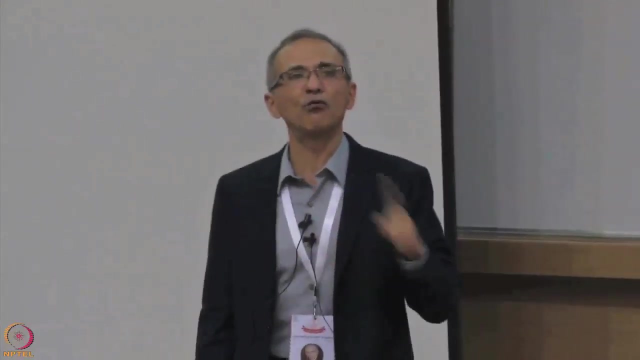 percent of specificity built in, Which is incredible if you think about it, because not even that existed within the DNA diagnostic space. Well, it turned out it was too good to be true. there were errors at all levels of this. So what the NCI decided to do was, when it came to proteomics, they did not move forward. 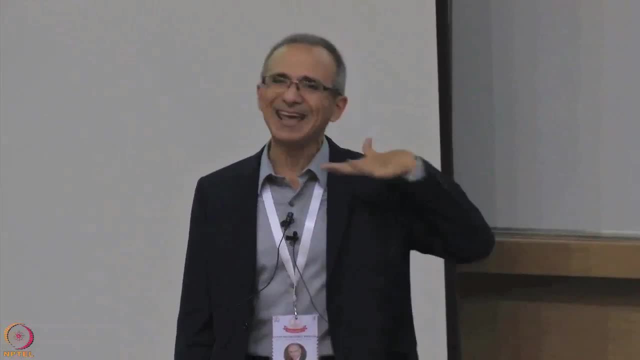 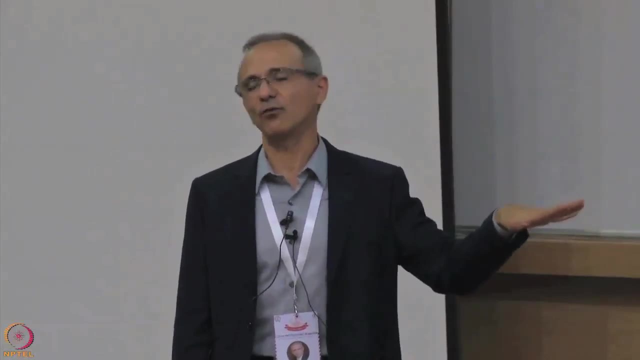 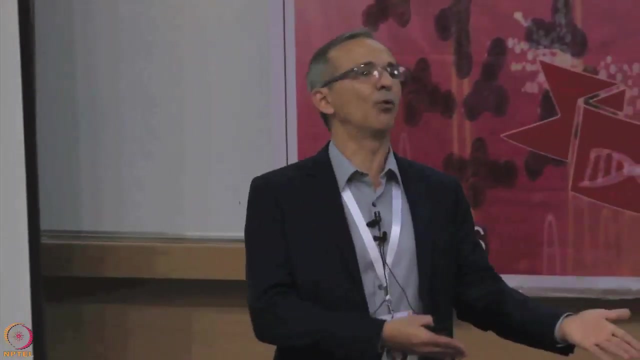 in 2006 when they created this to go after biology, that was taken off the table. So they basically wanted to go after the analytics and determine: can you standardize these powerful next generation methodologies, predominantly a mass spectrometer? And if you can, then you would come back to our board, you would give us the confidence. 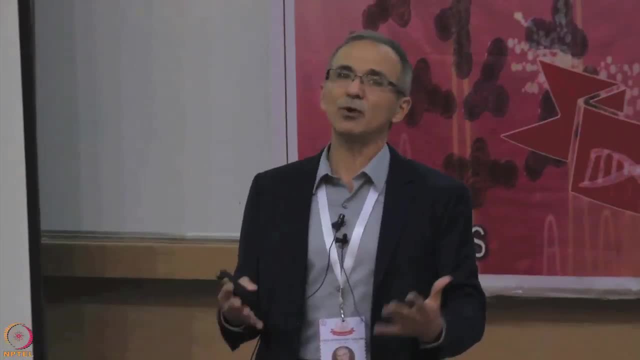 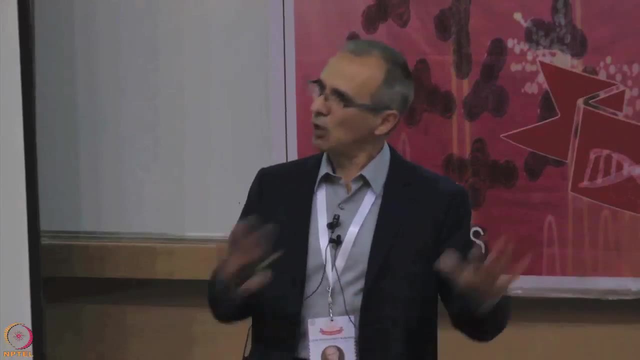 that we could trust the measurements, in other words, what you are measuring. it is going to be representative of the biology you are trying to go after. it is not going to be attributed to an artifact, attributed to way the sample is collected or the way you are processing. 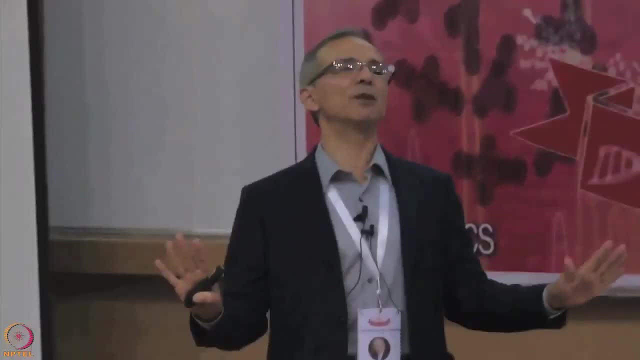 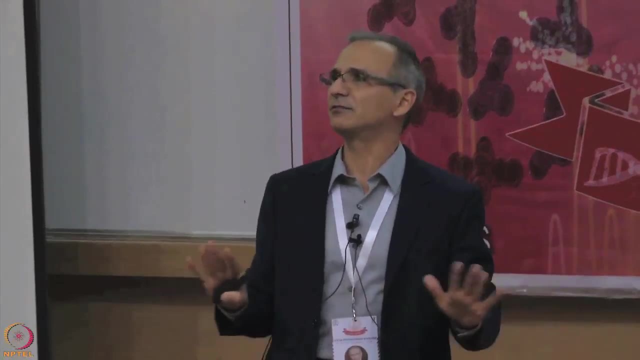 your sample, Because that is very important. everybody is going to measure something, but you got to ask yourself: is what you are measuring going to be representative of the biology of a disease state, or is it an artifact? Because if it is an artifact, it will not go towards the data. 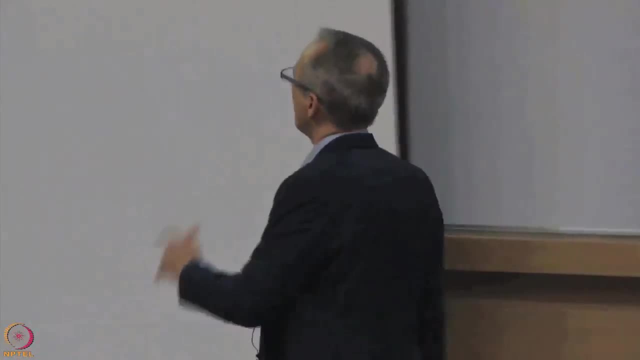 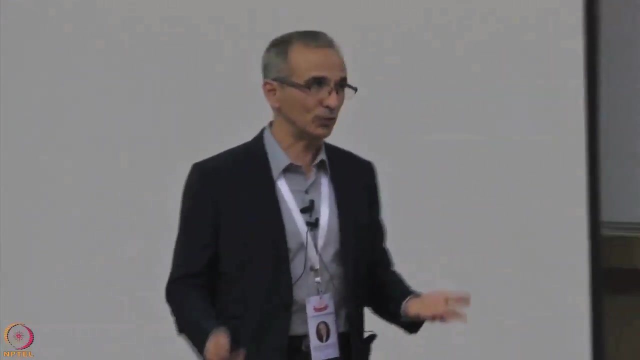 So that is what the NCI decided to do. It will go towards patient care most likely, and then, if you could do that, you could go after biology. So for the very first 5 years we had to try to standardize as much as we can. 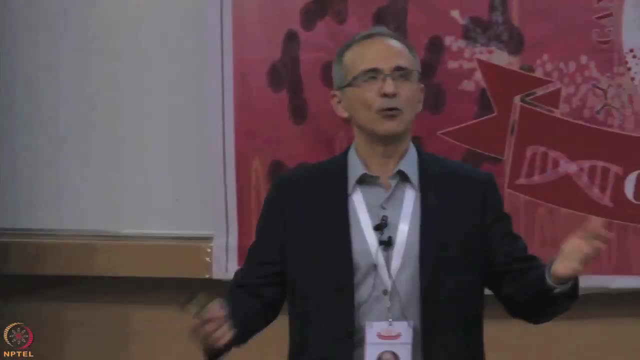 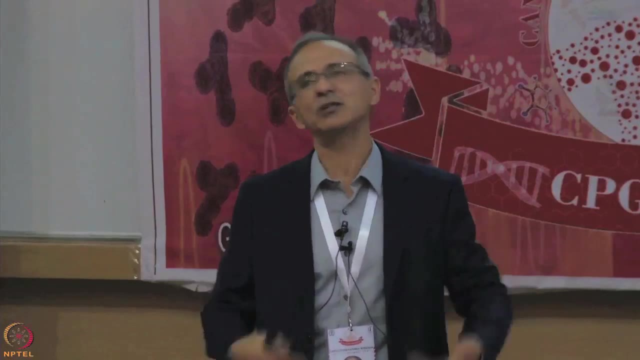 I am not going to go through all the science, but here is what we ended up doing. We basically carved the space of proteomics, exactly like you do in genomics and genomics you first do a comprehensive characterization. once you identify what you want, then you basically: 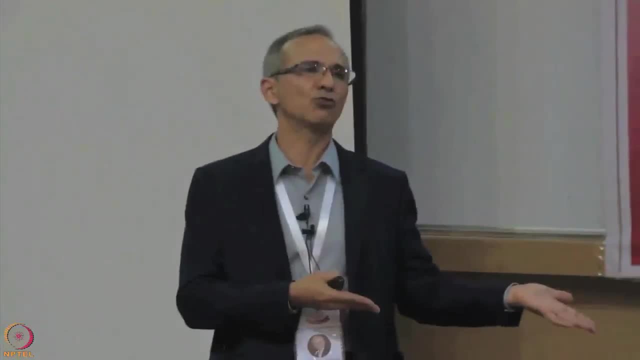 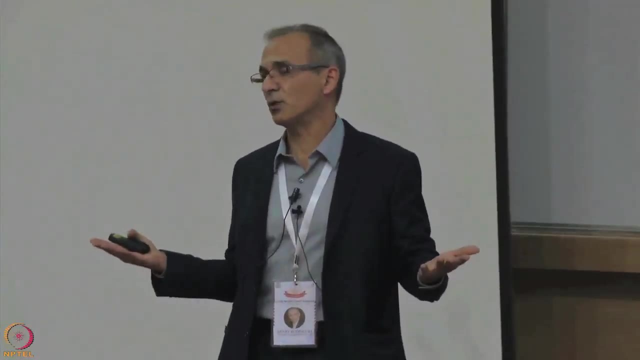 develop targeted panels. So targeted panels that today it is actually drives a lot of our patient care, especially within the clinical trial space. So when it came to proteomics, we decided to take a very similar based approach. If you do a deep dive, that is basically what a lot of people refer to a shotgun. I am not. 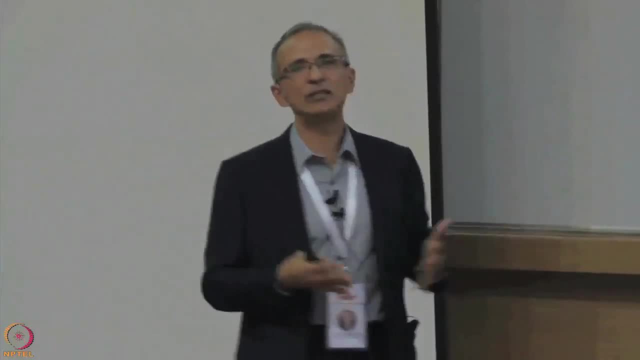 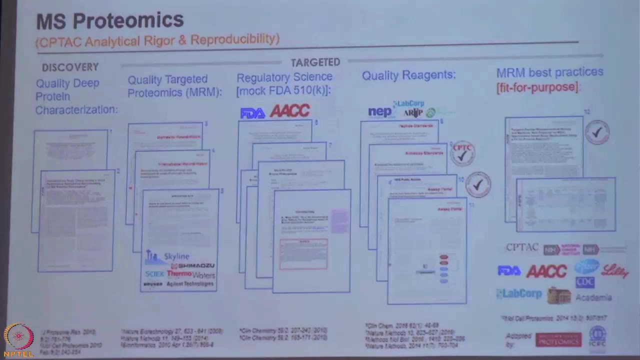 a fan of that terminology. So basically I tend to call it very deep, comprehensive coverage. You are trying to measure as many things as you can, and there we basically showed: if you distributed a standard operating procedure amongst multiple laboratories, guess what you get very good concordance type CVs, typically less than 15 percent and sometimes even less. 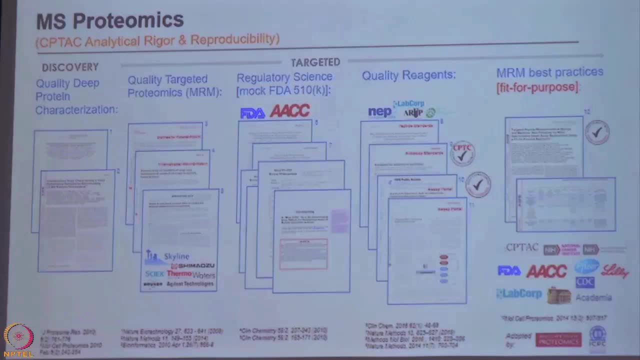 than 10 percent, which is very good. So that is the general space of targeted mass spectrometry, because once you identify the large landscape, you do not want to do this comprehensive based approach all the time. It is very high cost, it is low throughput and it requires a lot of sample. 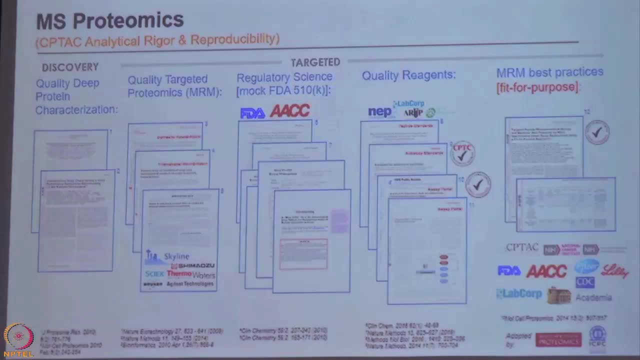 So you want to get something that is going to be very locked down, and for lockdown, you typically want to target based assay. So in that space, we basically at the time looked at what is now referred to as multiple reaction monitoring, and they have different ways of phrasing this, never invented it. this. 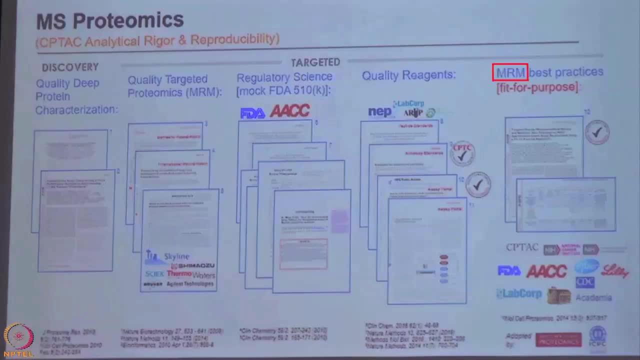 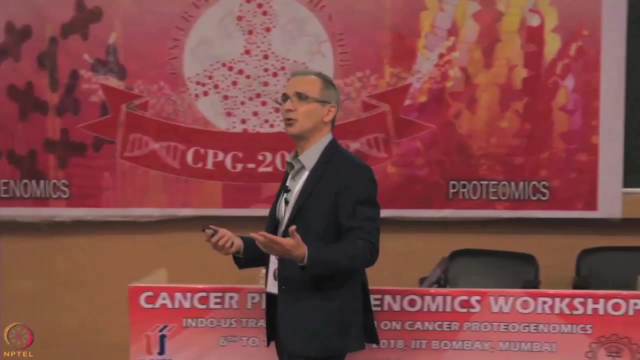 existed in clinical labs for 30 years. they basically use it for measurement of small molecules. So you typically want to ask the question: if you roll it up to a peptide, can you use it in that space and is it reproducible? and, more importantly, can you transfer the technology? 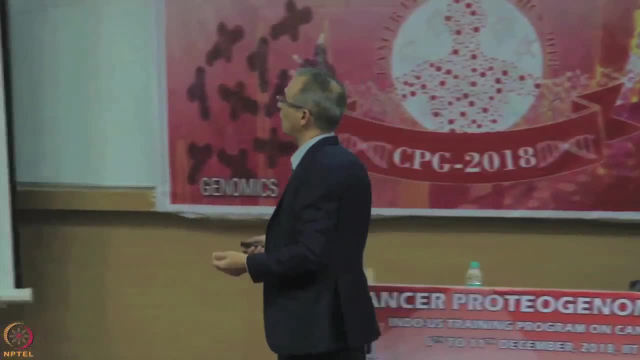 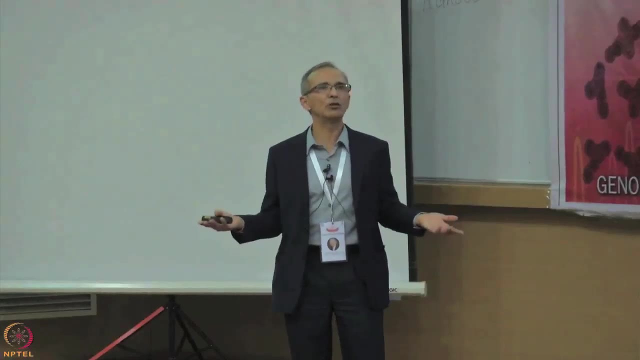 across laboratories and get very good type measurements. So what we ended up doing? we basically looked at multiple reaction monitoring. we did a series of round robin studies. One involved eight laboratories in the US. we got very good results. Another one that we did, an international study: labs on the east coast, west coast, the US and 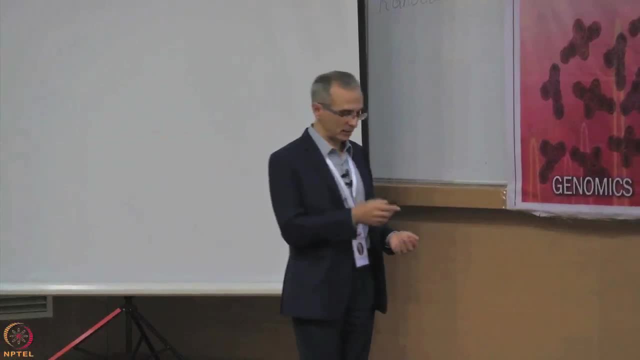 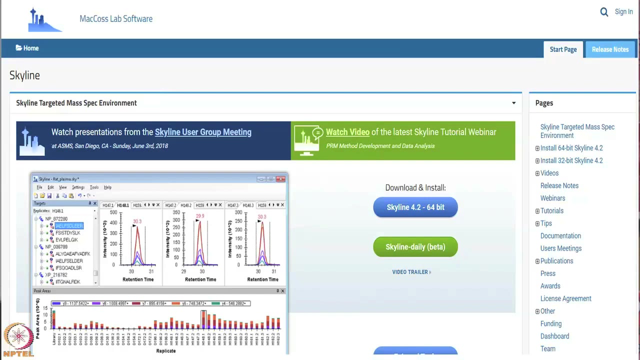 we had a lab in Asia. Again, very good results that we obtained from that, Thank you. People was talking about skyline a couple of days ago, So skyline is actually a little product that came from one of our laboratories when we were actually creating this program. 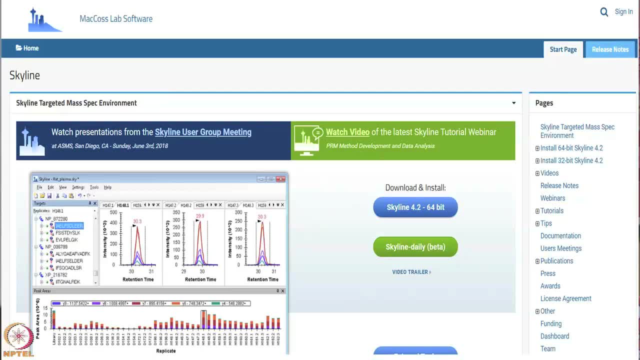 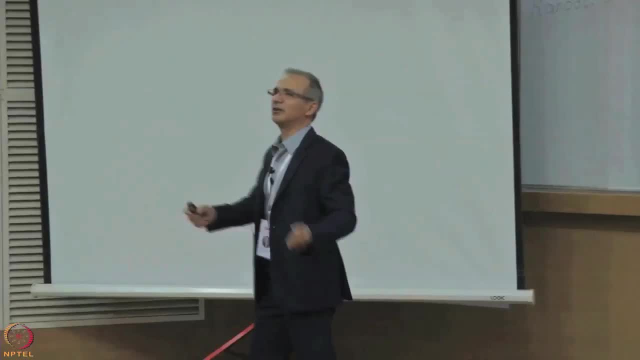 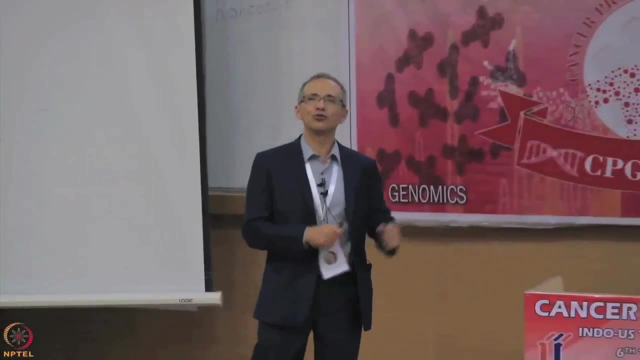 It is a great little tool and it shows you how, from basic science, you could get a computational product that is now is being used broadly by the research community. The other thing we started to ask is: well, what if? what if you could take your technology and you could potentially move it a little bit further towards regulatory approval? because 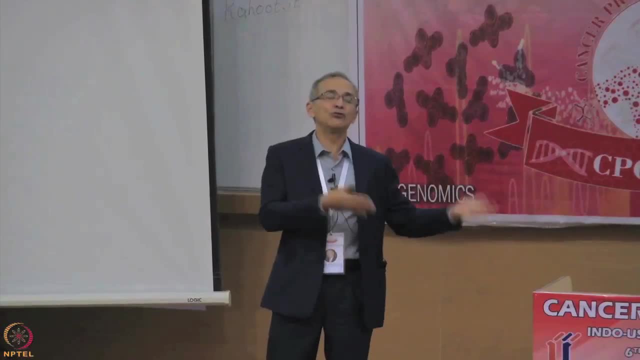 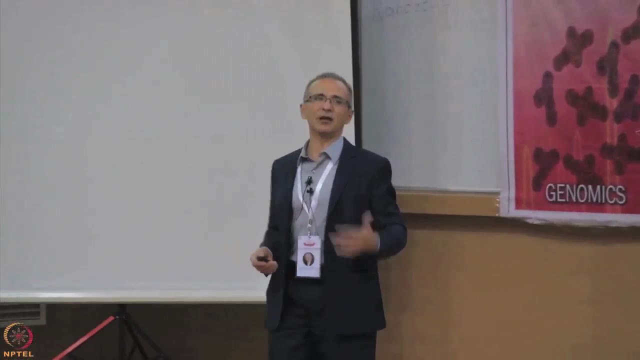 ultimately that is the goal. You want to put it in a clinical laboratory and hopefully use the information to go back towards patient care. In the US that is the food and drug administration. So typically to get a device cleared as an IVD MIA you need to go through the FDA and 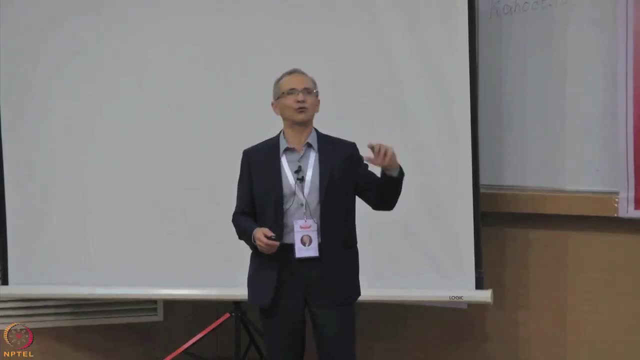 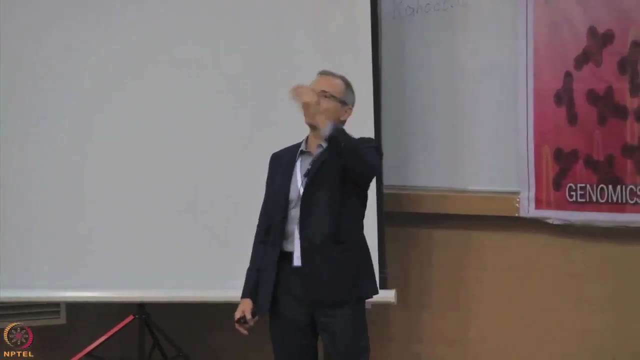 there is two stages behind it. A very first one is what we refer to as a 510 document. What happened in the past was typically a manufacturer will submit it, it gets all marked up by the food and drug administration and then they give it back to the submitter. but 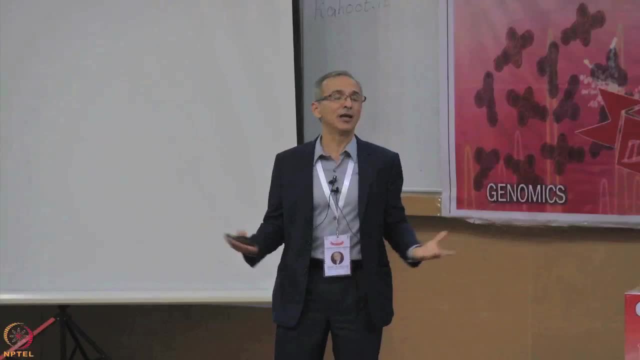 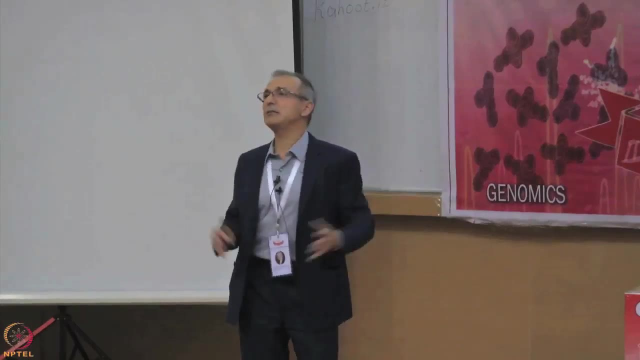 the submitter never wants to release it. We were very interested In releasing all that information to the public, So what we ended up doing was we held a workshop with the regulatory agency and we basically made up all the data, but we did not make up the analytical workflows. 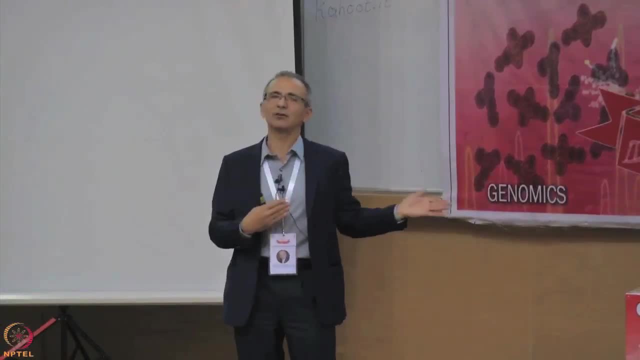 The beauty of that was it allowed us then to submit all our data to the regulatory agency as an official filing. They marked it up like they would for any device manufacturer, but because we submitted it and we made up the data, then we were able to take the document and we published it in. 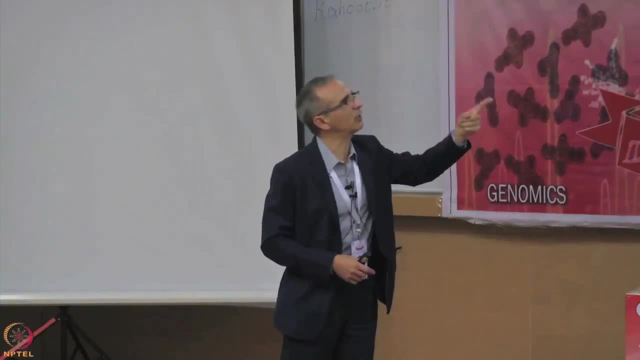 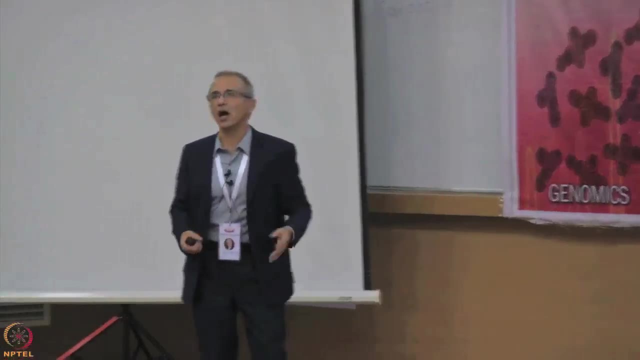 the public domain. We actually got it published in a clinical chemistry lab. Okay, Because we partnered with the American Association for Clinical Chemistry in the United States. The other stuff we realized early on: a lot of the commercial grade reagents that are out there in the community were not to the standards we felt they should have been. 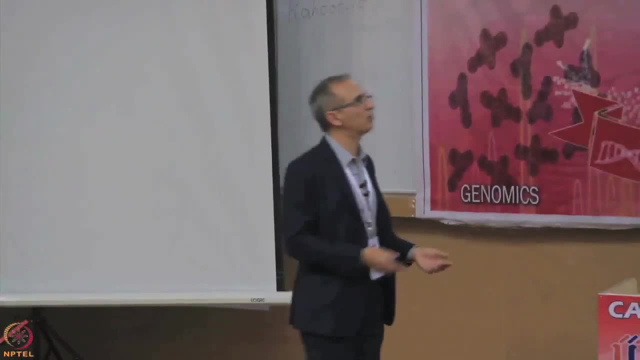 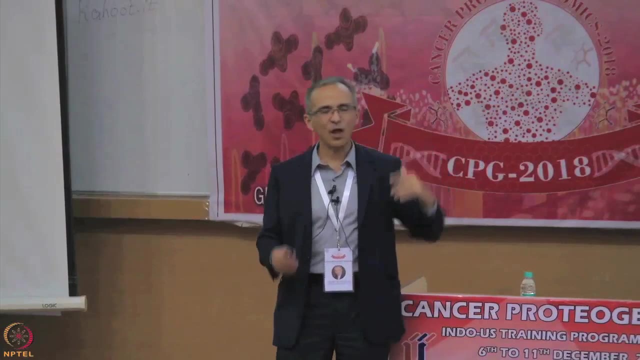 So we have worked with the commercial sector, trying to raise the sort of quality of the products that they released. And then the other one was a lot of people talk about. I have developed a targeted based assay. I will be honest, after a while a lot of us did not know what that even meant. 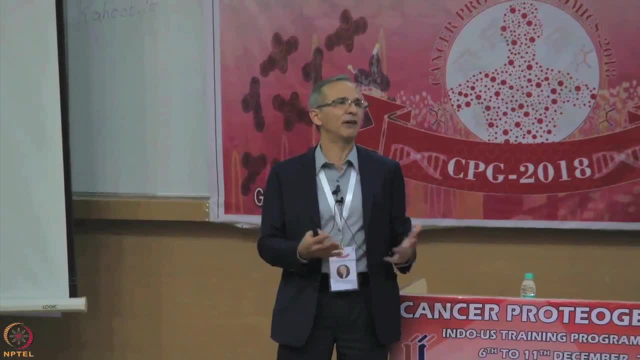 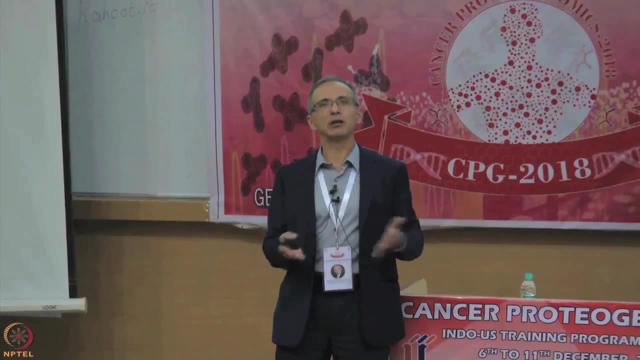 Because people develop assays and you find out. what they mean is that they have other. they have either developed a theoretical assay or they develop the assay running it in buffer. The last I checked: if you draw blood or a tissue from a patient, it is not theoretical. 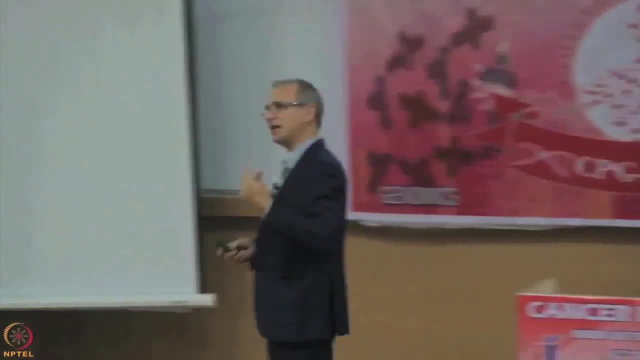 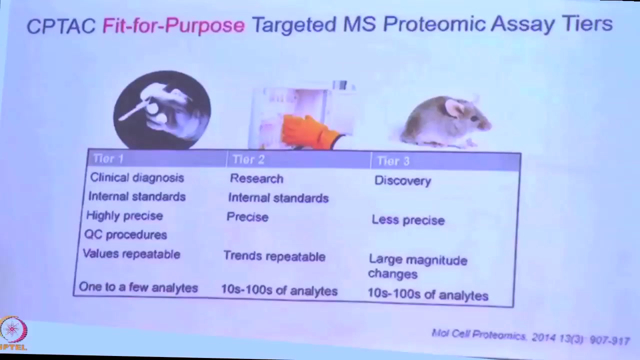 and there is no buffer flowing in that system. So we wanted to develop a clinical based way of thinking about it. So basically it is a fit for purpose based criteria, And we actually did that and, what is quite nice about it, in a very simplistic manner. 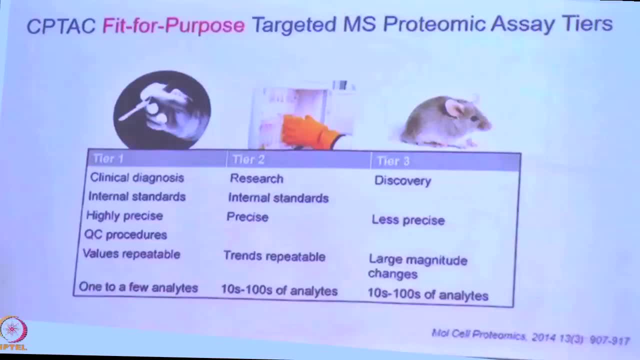 you could kind of see it as the following: We developed tiers: tier 1,, tier 2, tier 3.. Tier 1 is basically a standard assay. Tier 2 is basically a standard assay. Tier 3 is basically a standard assay. 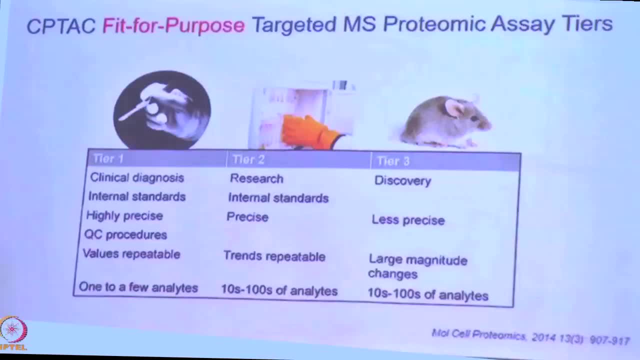 Tier 3 is basically a clinical grade assay. We do not do that within our program. Tier 3. there is less analytical rigor involved in that when you have to submit these sorts of criterias. But tier 2 is a nice little sweet spot, that everything within the CPTEC program we actually 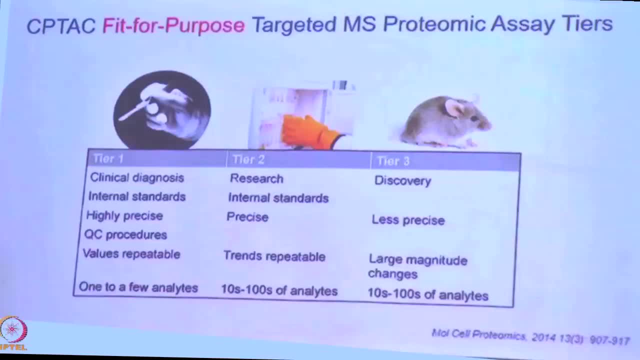 adhere. What is quite nice is that this ultimately now got picked up by the molecular cellular proteomics as a journal and also by the international community. So anytime you know, submit to this journal and you say that you have developed a targeted based assay. 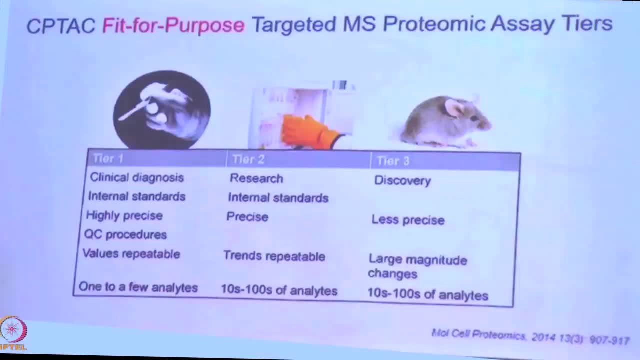 You will have to adhere and describe your assay based on one of these analytical tiers. So with this in now, with this is a 5 year window. At this point we go back to the board of NCI. We could- we actually demonstrated that we are able to get very good analytical understanding. 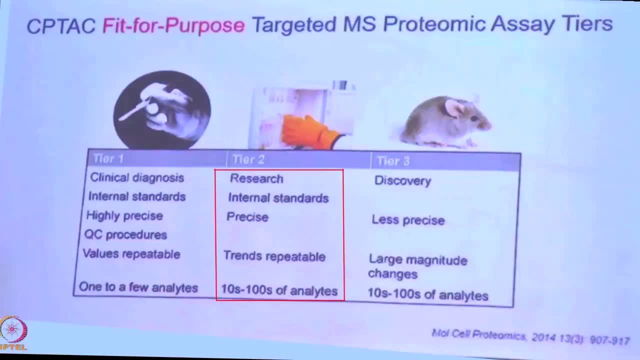 of these technology, predominantly mass spectrometry, And now we get approved to move it to the next stage. and that next stage was interesting. We wanted to explore as a pilot, to create a model, So we have a very good analytical understanding of these technologies, predominantly mass spectrometry. And now we get approved to move it to the next stage, And that next stage was interesting. We wanted to explore as a pilot, to create a model, So we have a very good analytical understanding of these technologies. approximately mass spectrometry. Why did we want to go after biology? The biology we wanted to go afterwards, specifically the cancer genome atlas, because that started biology 5 years before us, were 5 years behind And the way we basically phrase it to the board was: we want the exact tumor that just went from a patient to the cancer genome atlas and was comprehensively characterized and 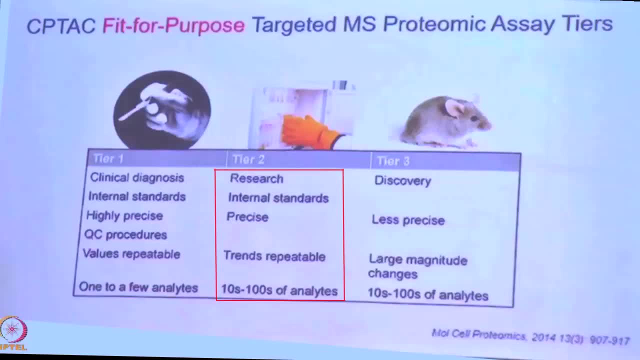 will take it, And then we are going to put a comprehensive proteomic characterization right above it, And, ultimately, what we are trying to find out is: are you able to identify a biologic pathogen? and then? so that is where we are going to participate in it. 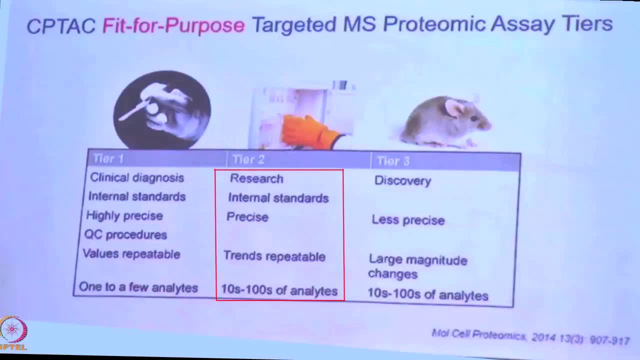 Here. most of these concepts ago actually exist and they did not exist. but think about back then. they do exist- additional biology that is either difficult to obtain or simply not feasible through genomics. So think about it because if what you come out of that sort of a finding is, I could confirm. 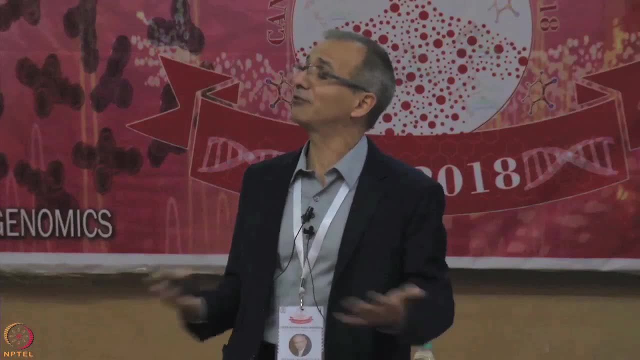 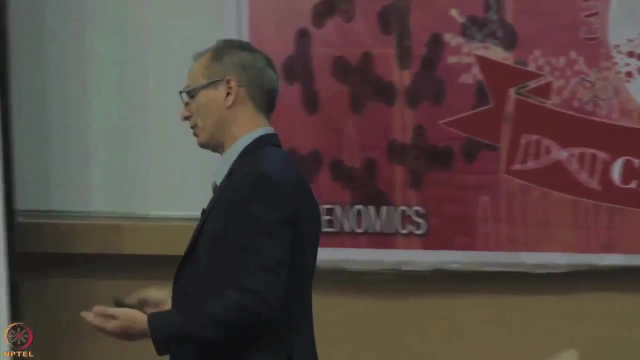 what my genomic colleagues just found. it is going to be very difficult to convince people. proteomic has a role, because proteomics cost more and it is lower throughput and does require a higher amount of sample input. So that was the goal. can you find additional biology, pure and simple? 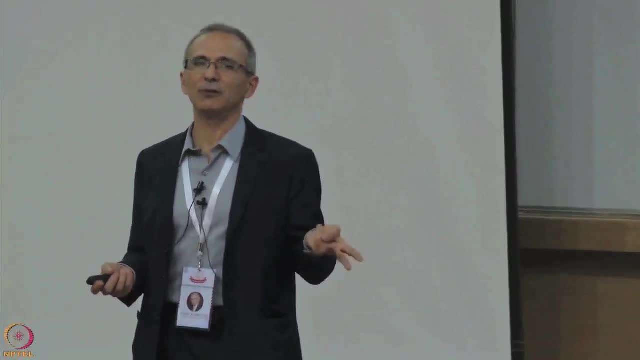 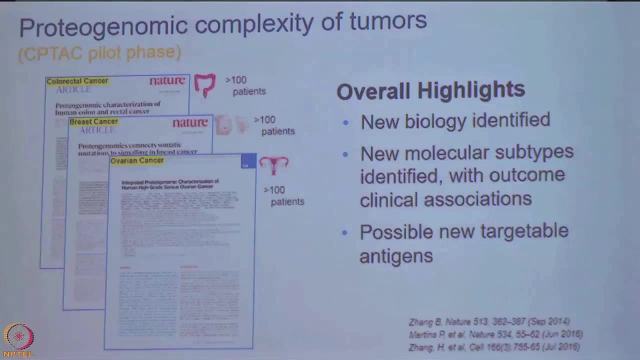 So here is kind of what we ended up doing. We went after three cancer types of TCGA. We went after colorectal cancer, ovarian cancer and breast cancer- On average about 100 individuals for each one of our studies. Suffice to say, here is the overall highlights. in every one of these we found new biology. 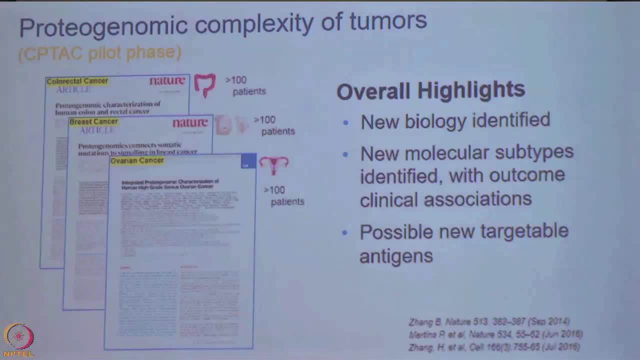 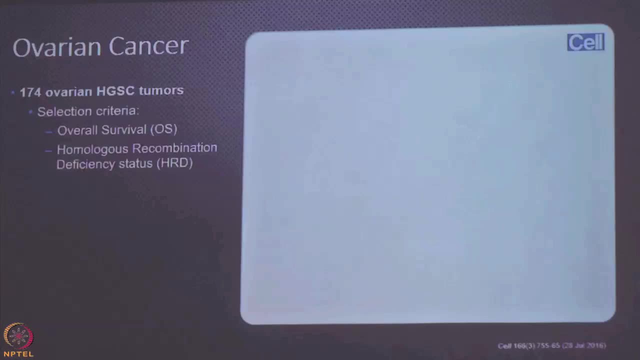 Now here is sort of a little example of what I mean by a finding, additional biology. If you look at the ovarian study, this is just one little slide that comes out of that paper. So in the cancer genome atlas we actually catalog just shy of 500 patients to come out. 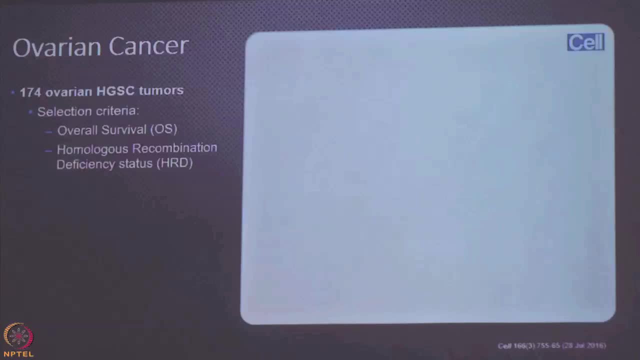 and come up with this with the observations that we did for ovarian cancer, and in that they did a whole series of analytical, different ways of looking at the data sets. So what our investigators had an interest in is, if you look at the proteomics landscape, 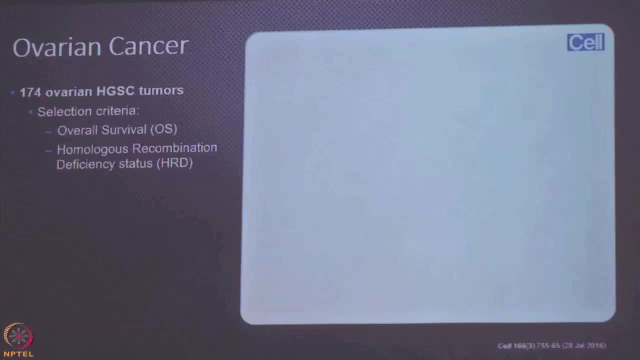 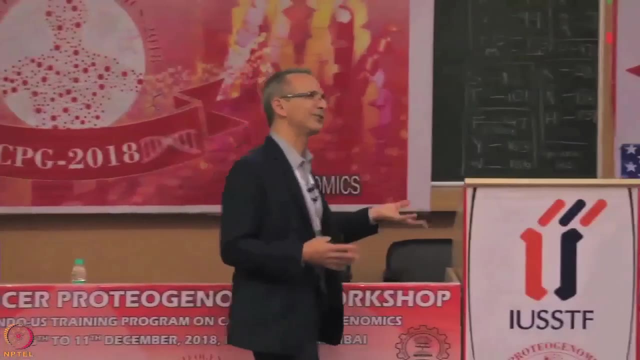 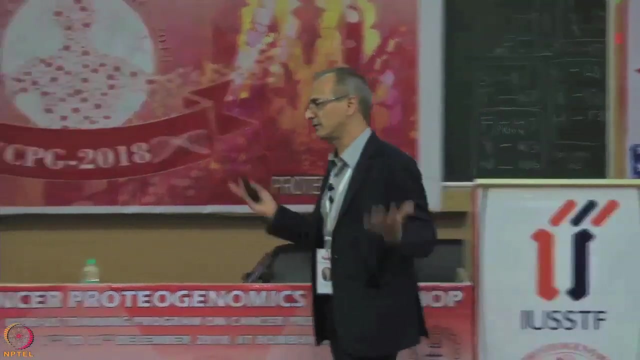 are able to tease out two features that is associated with ovarian cancer. One is going to be overall survival. typically, you wanted to find out if you could separate short versus long term, less than three, more than five years, and at the same time they were. So we found that in homologous recombination, deficiency or brokenness is commonly referred. 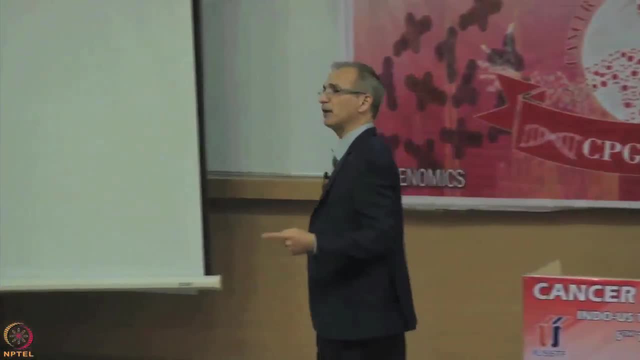 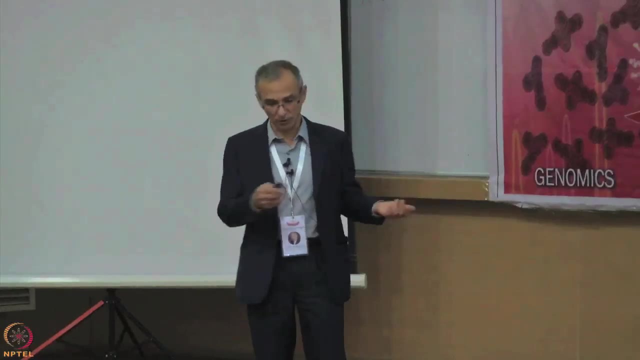 to as. So what they ended up doing was the following: out of the 500, we took approximately shy of 200 of those samples and we distributed to two laboratories. they were blinded to what the samples were, and they perform a whole series of bioinformatics on the information. 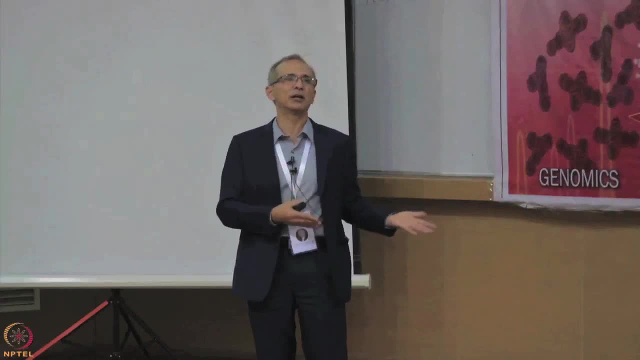 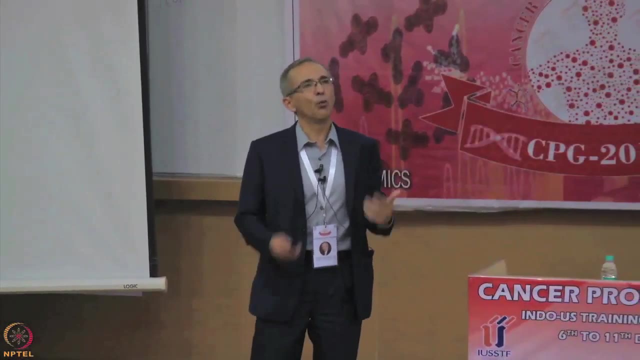 One of the things they did was a consensus clustering, kind of analogous to what is done at the RNA-seq level. and the question is: if you look at the information at the protein landscape, So if you look at the protein abundance, what do you get is going to be different, or we? 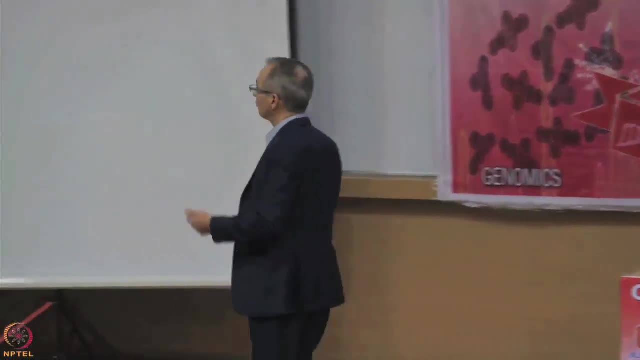 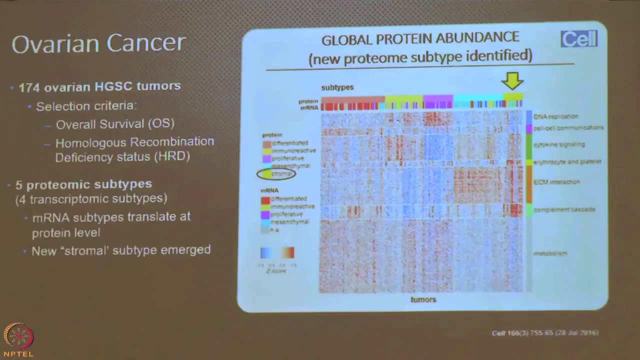 simply confirm what you did at the transcriptomic level. So here is what they found out: Not only do you confirm, but you are also to infer additional biology. So out of the four initial subtypes that you get at the transcriptomic level, they nicely 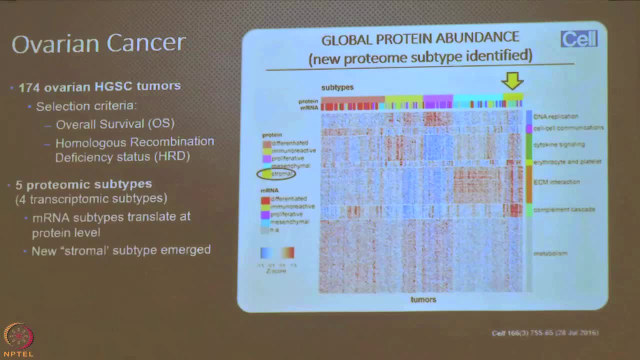 roll up to the protein level. but in addition to that, they identified a additional subtype that is identified here. This one they simply referred to as stromal, because a lot of these proteins tend to be associated with things like angiogenesis. But again, the key of this study that they had an interest in when they got these samples- 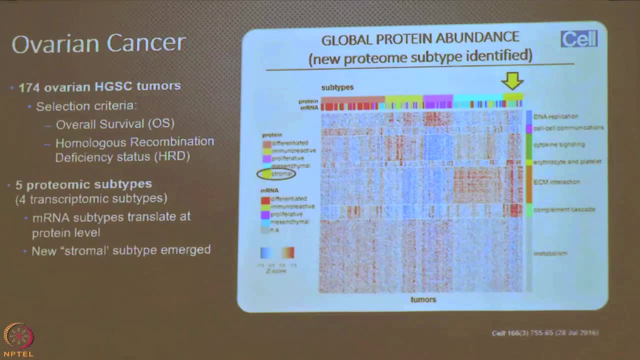 they wanted to identify. can the protein information at abundance level separate out for me either overall survival or HRD status? and it actually it turned out the answer was no. So protein abundance in itself in this type of an analysis could not separate overall survival or HRD status. 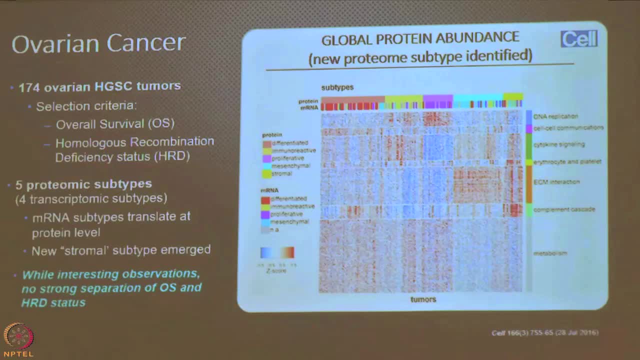 But that actually was not bad. and here is why: Because the same type of analysis was performed by TCGA, either in their flagship study or an additional study down the road that TCGA did, and they also cannot identify those two criterias. Now here is why it gets interesting. 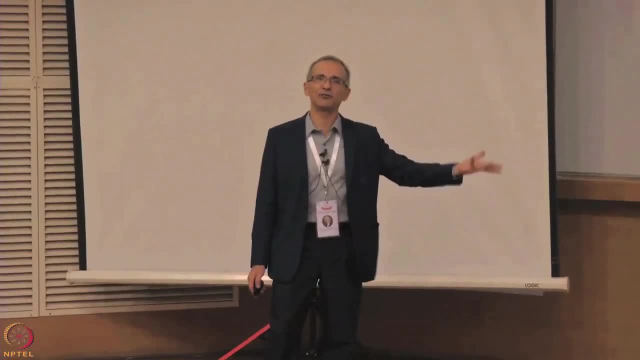 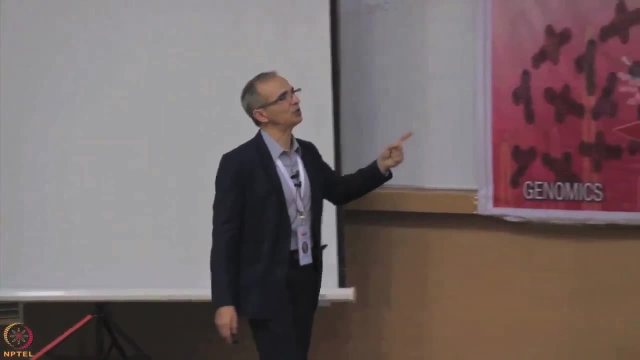 So these investigators? they had an advantage: they had genomics based data from TCGA and we had protein information. they also had modified proteins. at the same time, And as opposed to be asking these questions and trying to analyze the information from a gene based level way of thinking, they wanted to roll up the information into biological 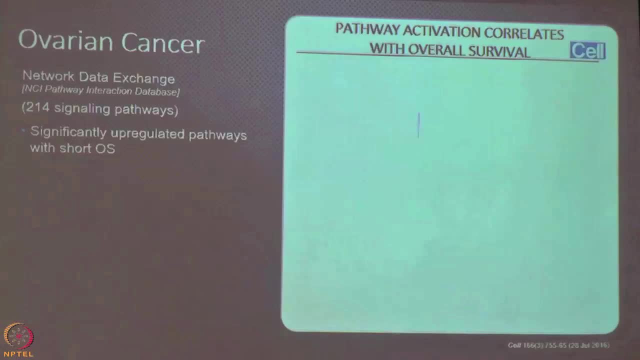 pathways. So what they ended up doing was they took all the data and then they plugged it into the NCI pathway interaction database and they identified just over 200 signaling pathways. Now, just focusing on the feature of overall survival. they asked a simple question: can? 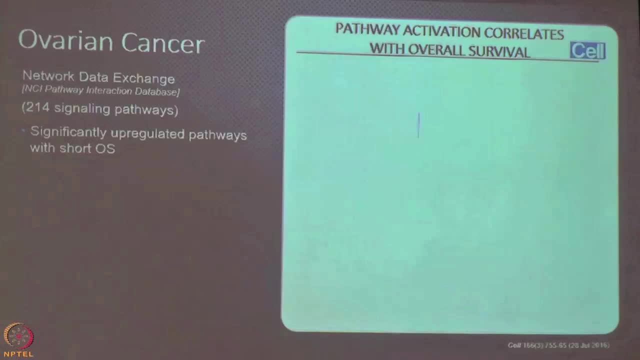 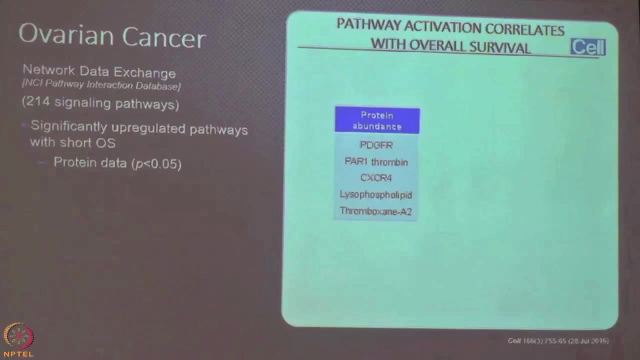 I use the information now looking at cellular pathways and try to separate short versus long term survival. So here is what they get. Looking at protein abundance, Well, It turns out 5 pathways all sudden rise up to the top from those just over 200.. 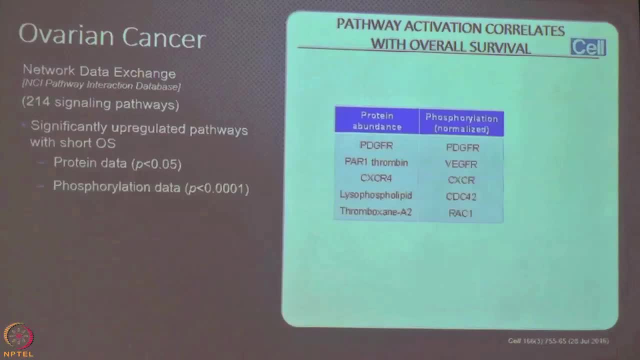 If you normalize against abundance and now look at phosphorylation, an additional 5 pathways became apparent. There is a nice crosstalk between one of these growth factor receptor pathways, but because we also had TCGA data from the same tumor, we also analyzed it at the RNA-seq level. 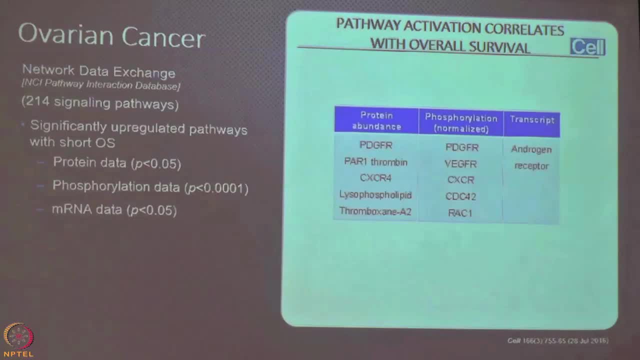 A different pathway came up. now you can begin to see what started happening to our program. In other words, if you were to perform an experiment, either looking at only protein abundance- and you are done, or you want to look at phosphorylation and nothing else, or 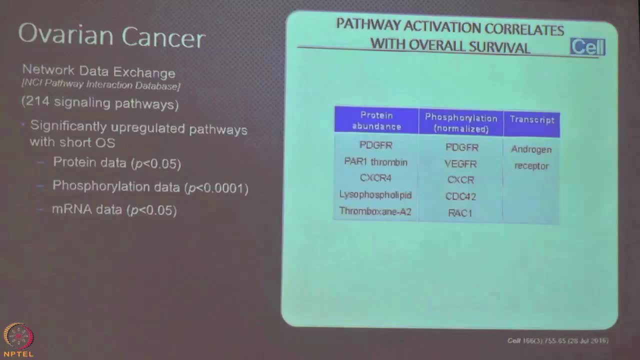 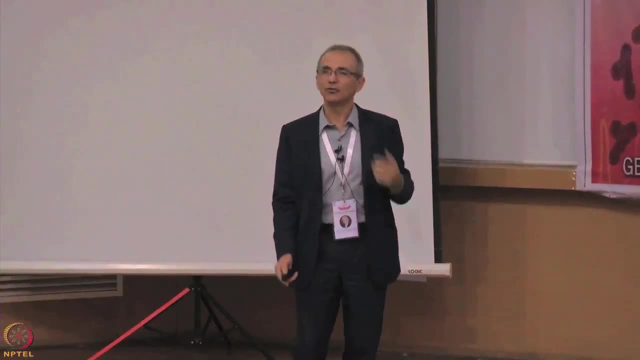 you just want to look at genomics, most likely you are going to be looking at an incomplete picture of the underlying biology for this study that we were involved in. So that became sort of a very turning point for us. So at the end of the day, what we learned from this was: if you have the opportunity, 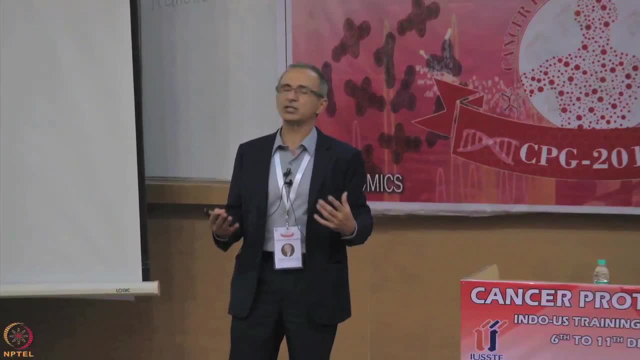 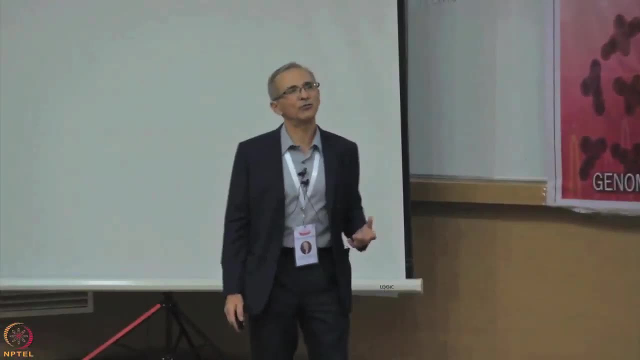 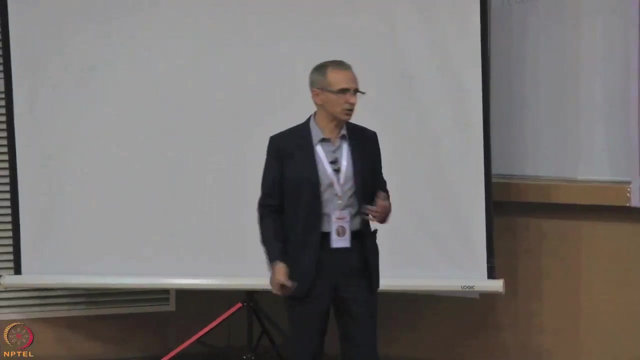 as these technologies are now mature and you can begin to actually perform comprehensive genomics with proteomics at the same time. most likely, blending these worlds together is going to give you a better understanding, not only of the underlying biology of the disease, but we hope. we hope that the biology could potentially translate towards patient. 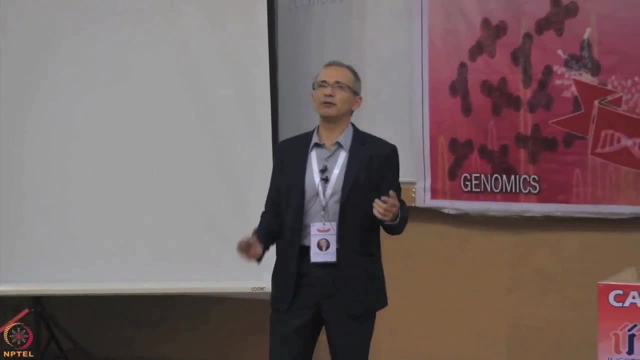 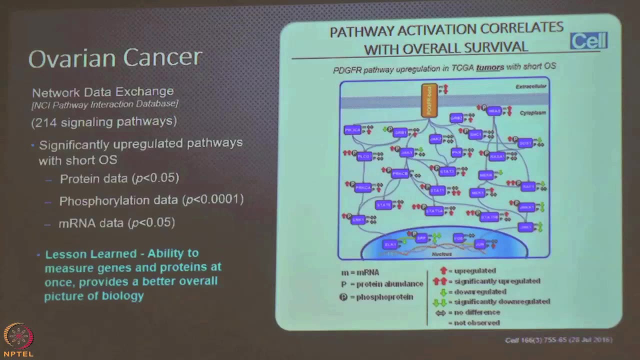 care Now, in addition, also to be developing very detailed pathway based maps, as are shown here. you can also begin to tease out those funky features that people like to look at. So, for example: So this looks at the what is it for? the growth factor receptor pathway, a very commonly 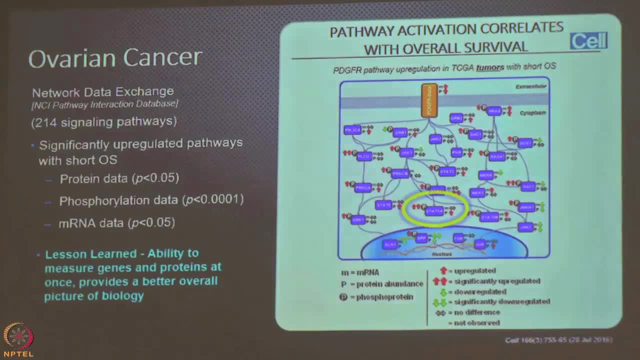 looked at, transcription factor turns out to be STAT5A and actually by rolling both informations together, if it is not that obvious here, basically what we showed was at the transcriptomic level, looking at overall survival, not much change at the protein abundance level. it kind of resembled at that point what you found at the transcriptomic, maybe a slight. 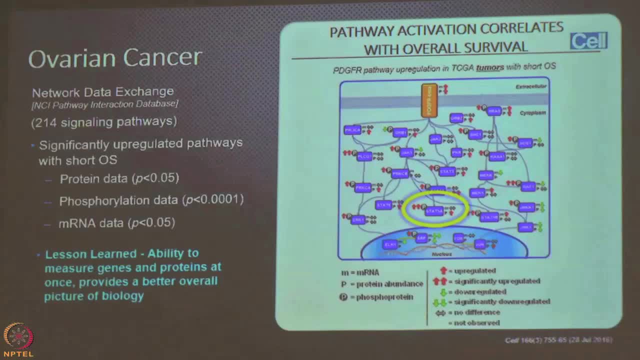 little bump and nothing really that is going to be significant. but really you saw a huge increase at the level of Of Of phosphorylation. So again three cancer types that we did all similar observations. So here is now what starts to happen, and I have seen this question being asked also. 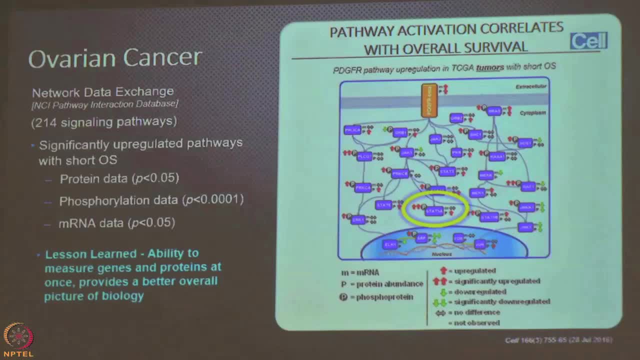 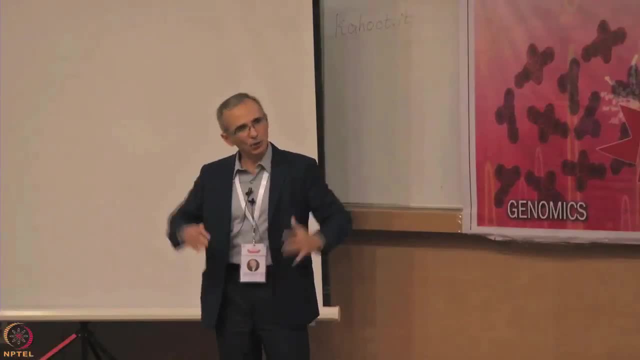 in the past couple of days. So now we have standardization: first five years. the next five years, which we just wrapped up, focus on trying to tease out biology, and we had to go back to our board And what people kept on asking is the same thing that people were asking for the past. 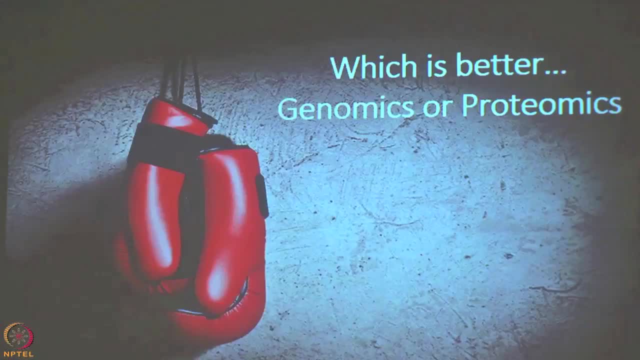 two days. and that is the following: Wow. So which one is going to be better? Should I only do genomics or should I only do proteomics? Should I do proteomics and completely alone, genomics? Which one is better between the two? 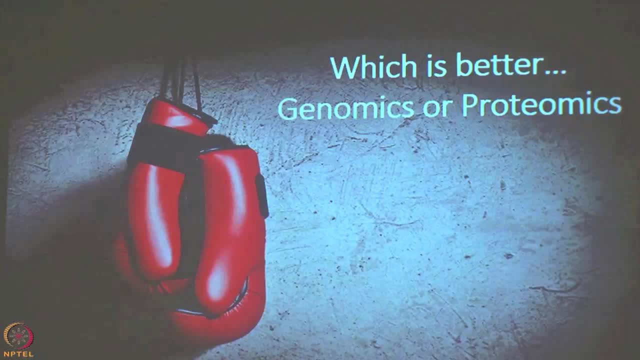 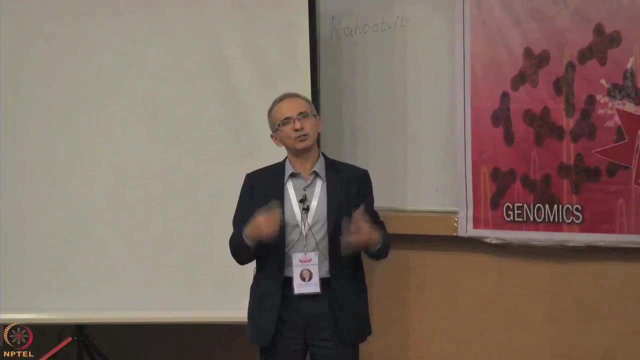 So the way that I kind of viewed it was: just take yourself back to a book of biochemistry. The first thing you learn is that everything has to relate to one another, and if you could get a good comprehensive systems perspective view of the biology, hopefully it is going. 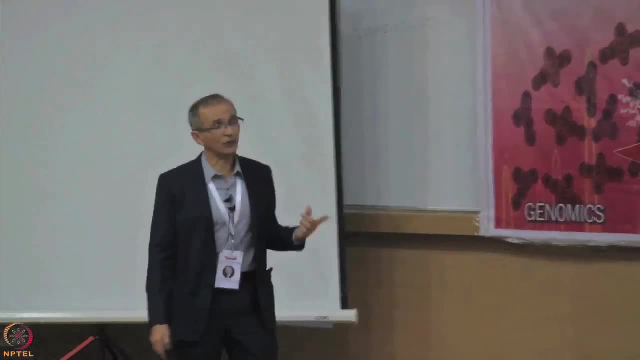 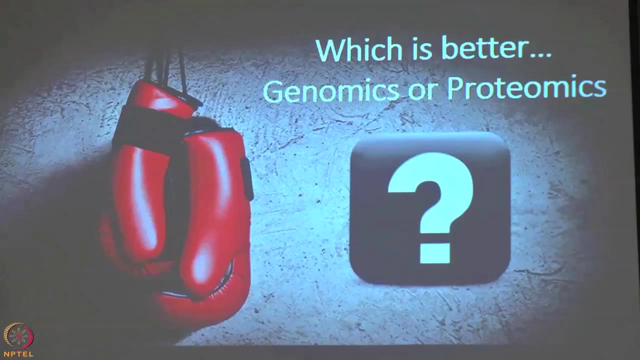 to be more representative of the disease state itself. So for us the answer became no, I seriously doubt, I seriously doubt. So if you do not understand any of the biology of what you are going after, why do you want to go after one of these omics now, when the technologies have become quite mature? 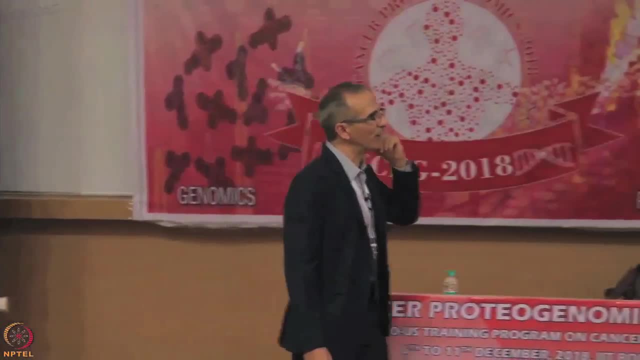 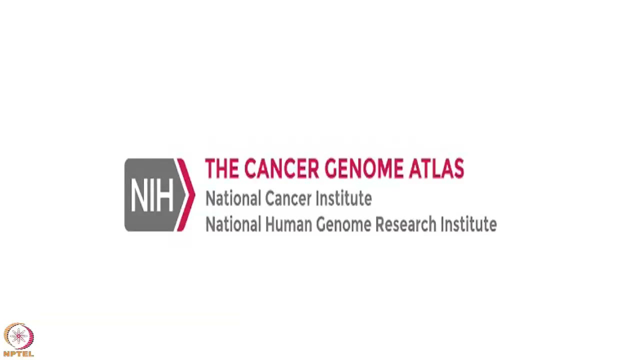 And here is why, which is what is the same argument that I made to the board about four years ago. If you look at the cancer genome atlas- again, the cancer genome atlas- I am a huge fan of this program, simply for what it was able to achieve in a 10 year window. 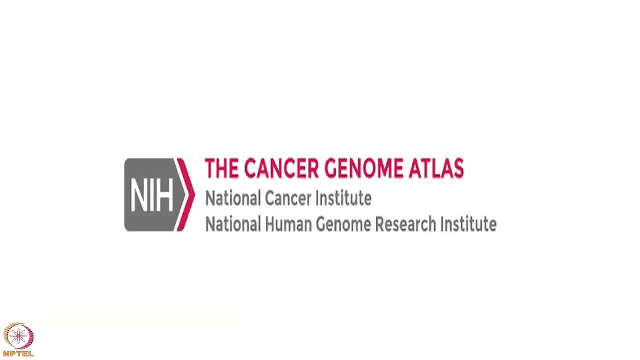 They went after 34 cancer types, just over 14,000 individuals, and in the process they found a lot of interesting biology. Again, you cannot put clinical context behind this, because the samples are never collected with a clinical question in mind, But nevertheless a very good resource that has been given to the public at large. 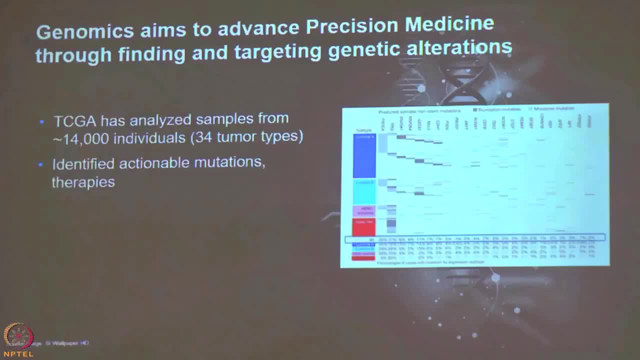 But in that they also identified a whole series of actionable mutations that now some of our small molecules. it is actually driving a lot of our precision oncology trials, So that is the good news. Now you could actually look at the other side of your story, which is what we are learning. 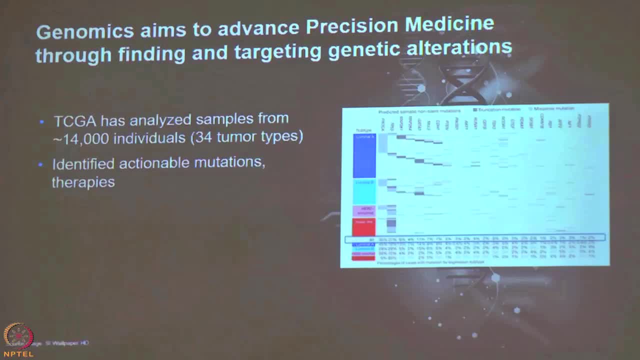 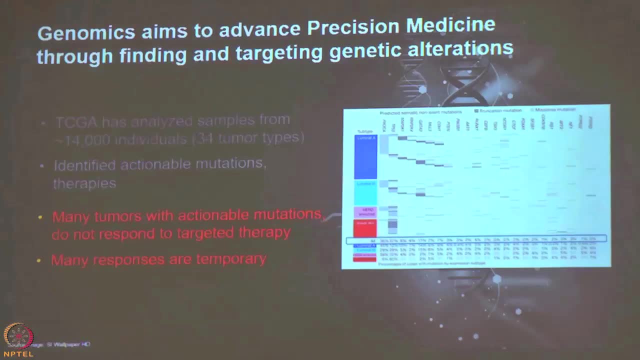 now, four years down the road And running a lot of these very precision oncology trials, What we are learning is that a lot of these tumors, that they had these actionable mutations, that we develop all these GMP facilities to develop these small molecules, those individuals. 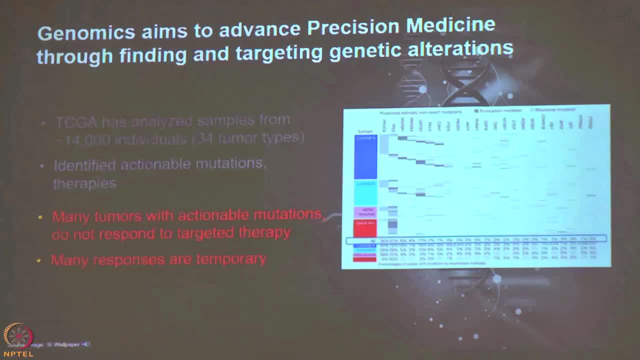 actually are really not responding long term to the therapy that they are being administered. If they do respond, it is short term and a lot of them actually develop toxicity. they got to take it from one treatment arm and then quickly move them into another. Why? 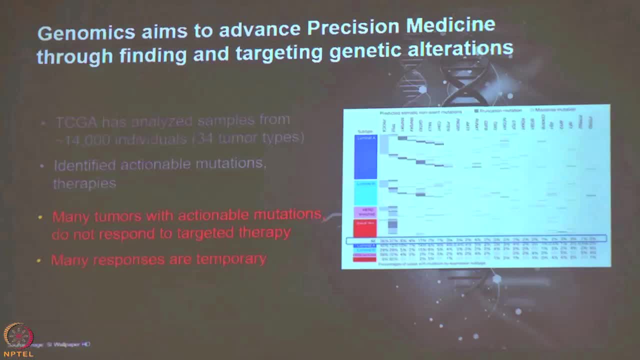 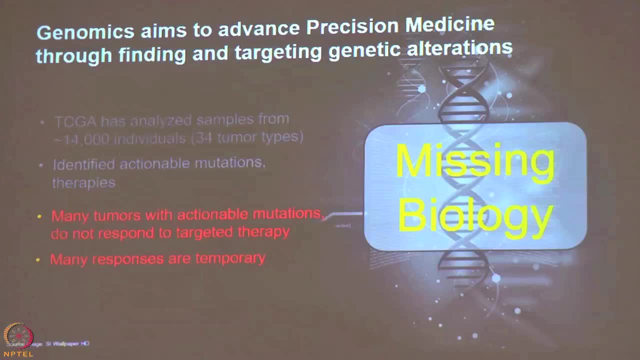 We have no idea why that is the bottom line. So, for me, what that tells me is that there is still a tremendous amount of missing biology. strictly focusing on a one omic based approach, Now you could actually flip the coin. just look at what is going on within the therapeutic 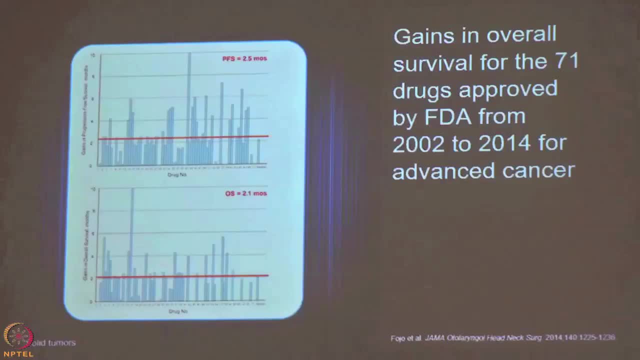 perspective. So this is a nice little paper that people could look it up. it is by a colleague named Tito Fo who used to be at the NCI and now moved to New York City, But he did basically this little analysis where he looked at solid tumors and what Tito 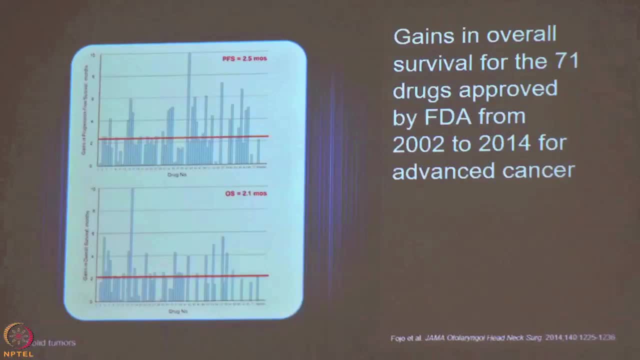 did was actually quite savvy. He went in the public domain. he said: look, if you look at the first main precision oncology drug that came out, which is Gleevec, along with Herceptin in the early 2000s, and what transpires over the past 15 years, there is just there is about over 70 of these drugs. 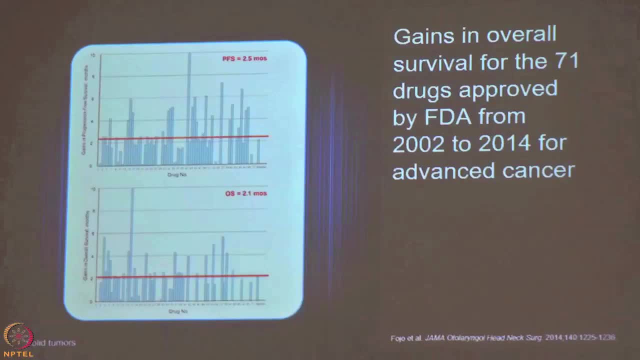 now, And if you look at the drugs, for all the different cancer types that they are, that they are being used either as a single or in combination. on average, just on average, what is the two main criteria that people look at? either overall survival or progression free survival. 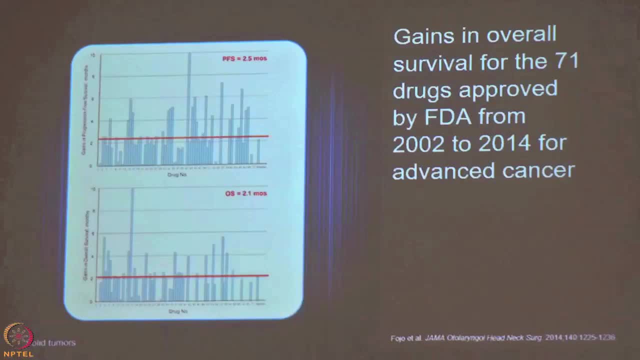 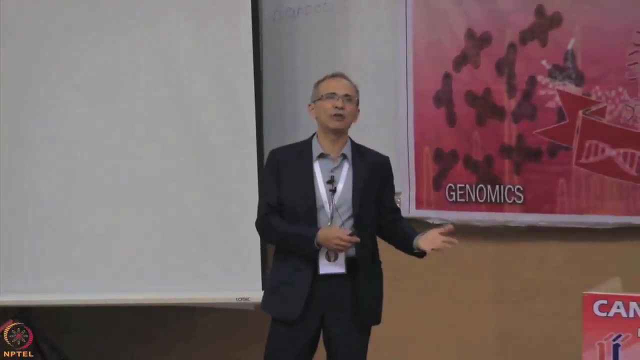 Now you excluded from this study, obviously, the exceptional responders, And what you found out is, for all these therapies, on average, for both of these two different metrics, it is typically no more than three months. So this played a big role the way that CPTAC now evolved in its current round. 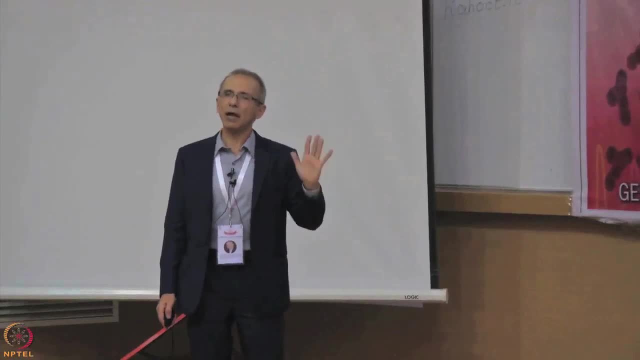 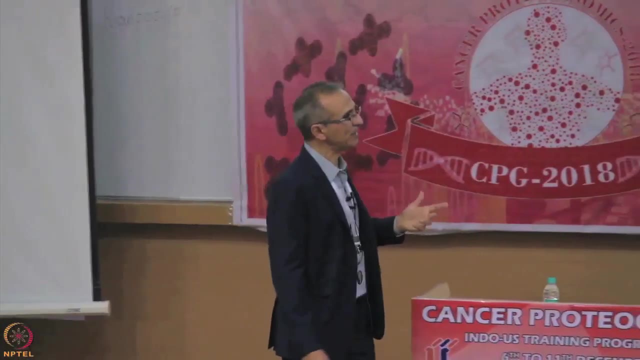 We still go after biology, like we did when the prior program, but now we are slowly trying to move into that translational space. So this is CPTAC today. So CPTAC is still held responsible to characterize deep, comprehensive therapy. 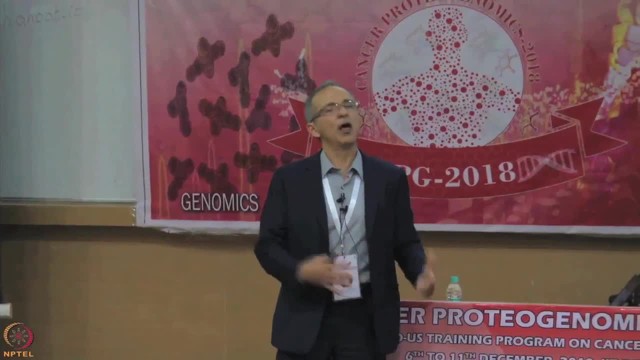 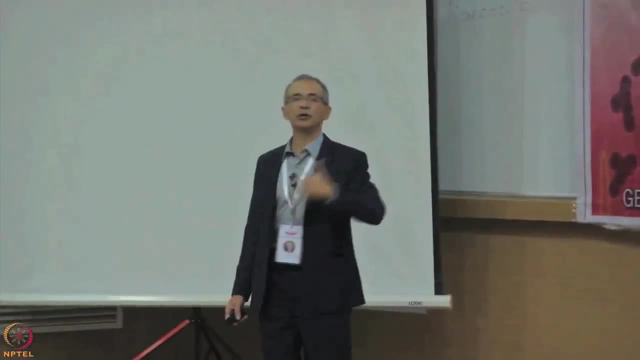 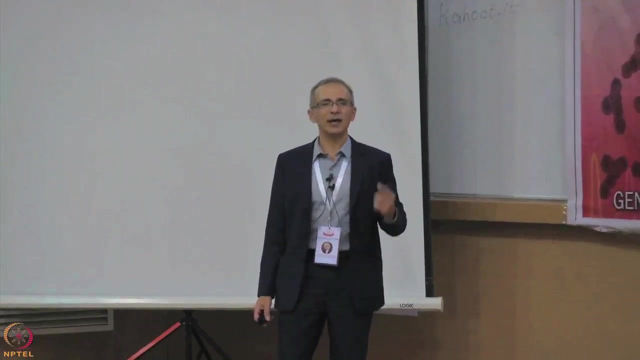 So this is CPTAC today. So this is a deep, comprehensive genomic characterization, along with proteomic characterization for five additional cancer types And all the information we put in the public domain because we see it as pre-competitive. At the same time, for the very first time, the National Cancer Institute has now partnered. 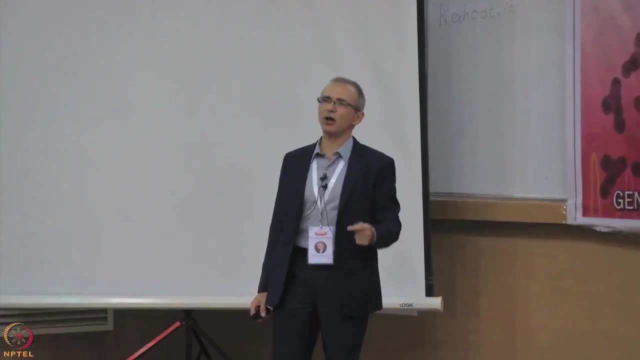 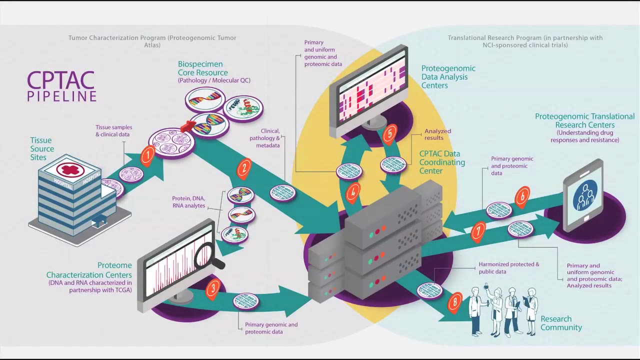 a proteomics laboratory with an ongoing precision oncology, typically genomically driven, NCI sponsored clinical trial. Now what is interesting there is that the information is not going to go back to a tumor board to figure out exactly what treatment arm or what therapy to administer to a patient. 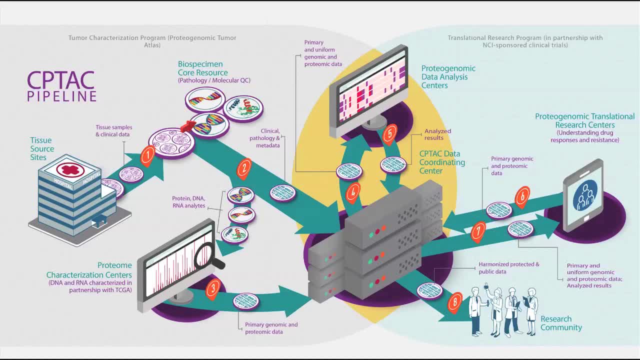 On the other hand, the information is basically going to be used in a reverse engineering manner, So, based on the study itself, you will be able to get samples from these trials, which are very well controlled. So the amount of clinical inference you are able to pull out of it is tremendous, and you 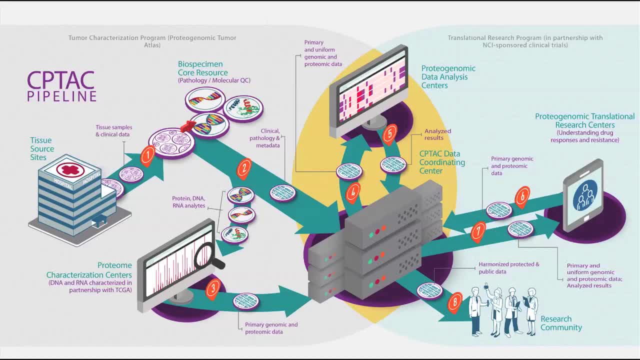 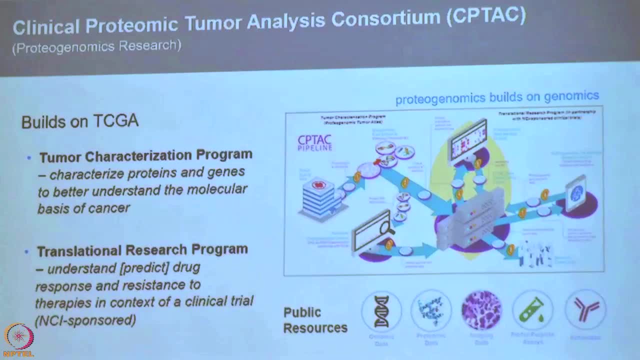 will get pre, during and post And hopefully what we hope to learn from that program is: if the individual did not respond to the way we think they should have responded, Based on the genomic information, can we identify the biology to the root cause of that by looking 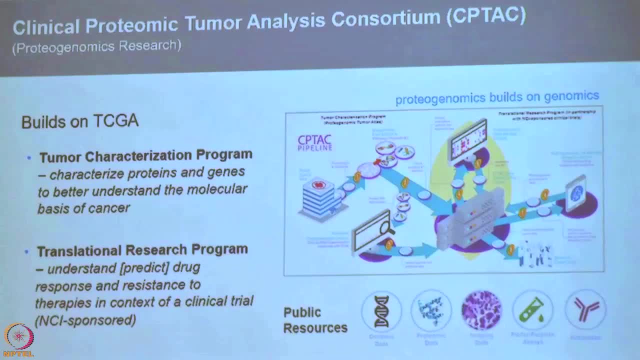 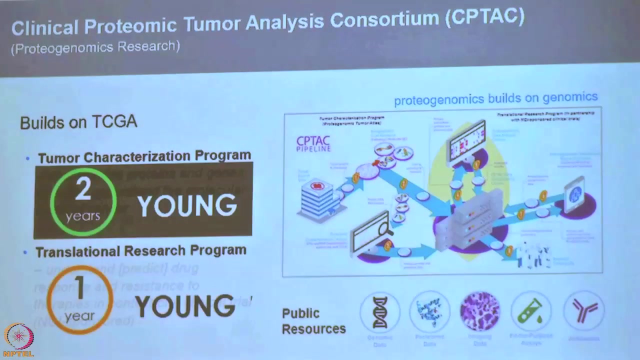 at the protein landscape of those subjects And if that turns out to be very revealing. my goal is that in the next iteration we want to combine those two worlds, fuse them together and actually go directly now to our tumor boards. Now, in terms of how old is the current CPTEC program? actually, it is not that old. 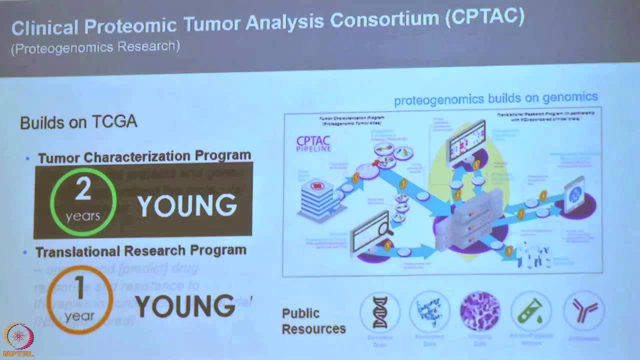 So, in terms of the comprehensive characterization, that is now two years old as a program, or young as I like to say, because I have reached my middle age crisis, So I do not like to use the word old anymore and the one of the translational now is one. 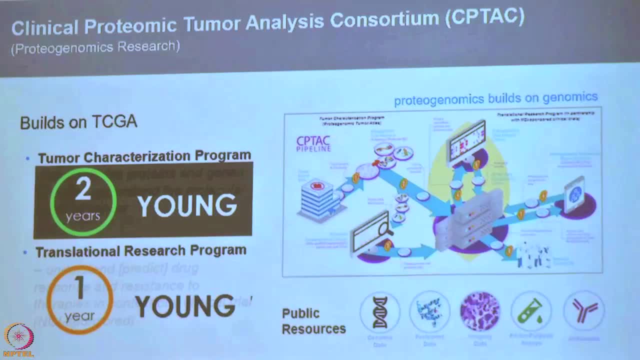 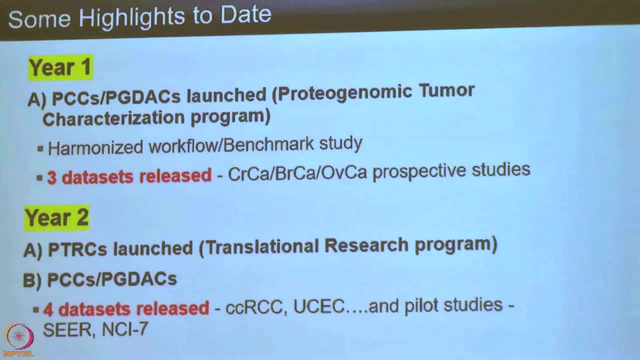 year young. So what have we done over the past two years? because that is really a two year window that the program spin around. So here is what we ended up doing. these programs are very complex. the reality is, you just cannot get something off the ground and expect it to work. you have to build your infrastructure. 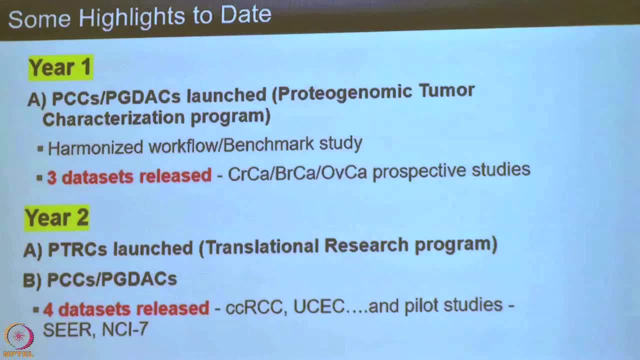 So the first one that we launched was the characterization component. the first thing we realized is that 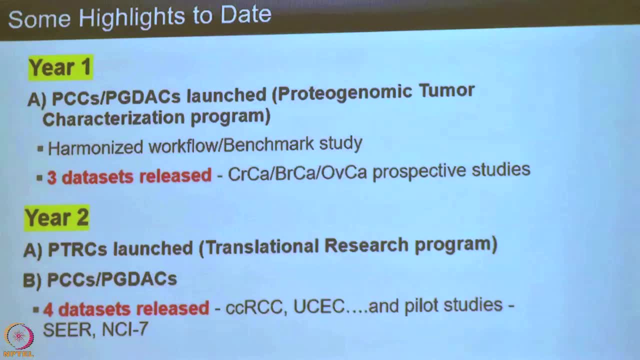 being main of what we call data production facilities or sites, and we tried then to try to standardize the best we can or harmonize the analytical workflows of the way that they would be producing those data sets. So that became very important for us and that pretty much took about a 12 month cycle. 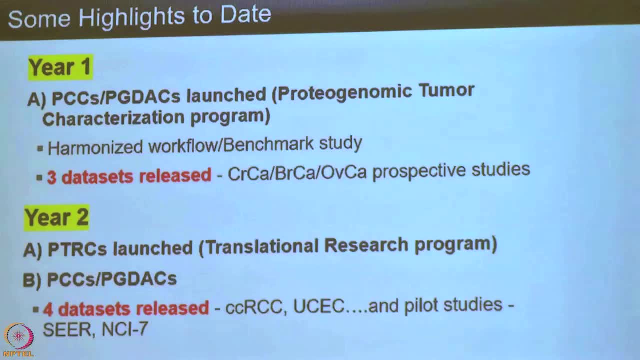 for us. at the same time, they also released an additional three data sets to the public, which is sort of a continuance of the last program, but these are now freshly collected samples that have been optimized for both comprehensive genomic characterization and- And that has to be- for colorectal cancer, breast cancer and ovarian cancer. 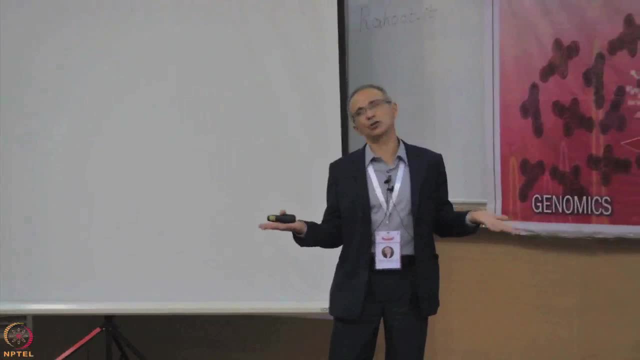 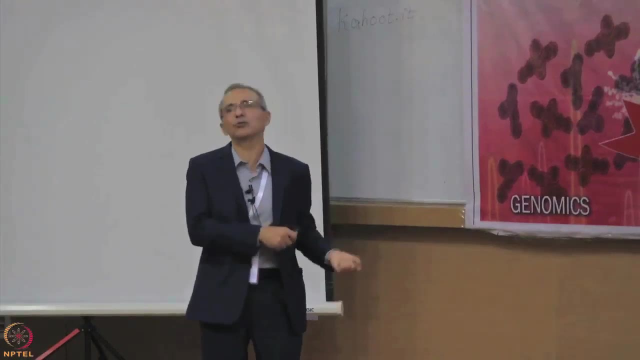 In the second year of our program we officially launched our translational arms as our partnerships with our clinical trials, And at the same time we also then continued in terms of that brute force characterization arm and we released an additional four data sets to the public. 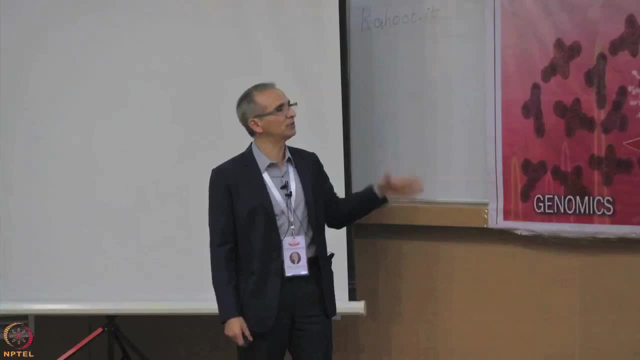 One, well, two of them actually, well, in fact, all of them occurred in the fall of this calendar year. colorectal cancer were released, endometrial cancer were released. Then we also released two additional pilot studies, one focusing on 30 year old samples to try and understand the stability of these bank materials, and the other one was sort. 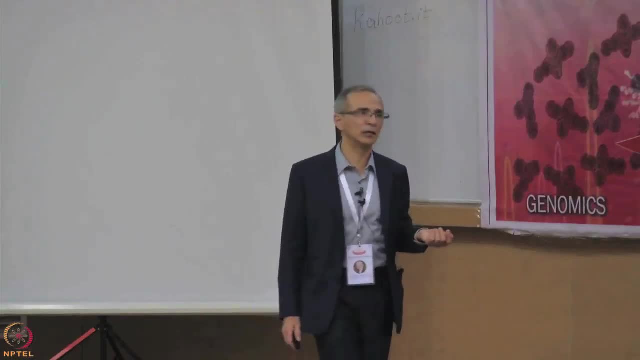 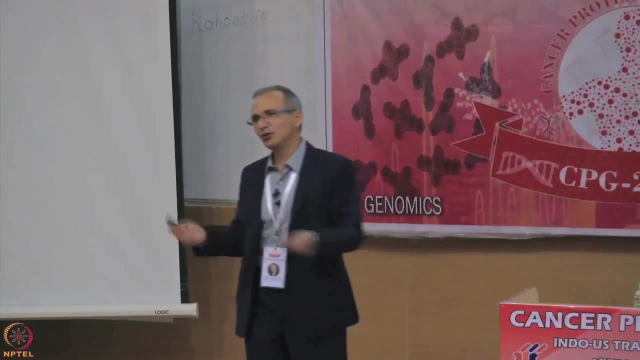 of a cell line study And we hope to release another one in the in the next several weeks. Now I talk about a lot. we give all this information to the public. The other question I get all the time is ok, so you give all this stuff to the public- is: 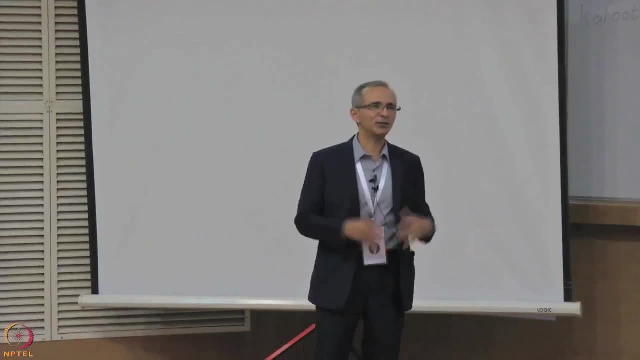 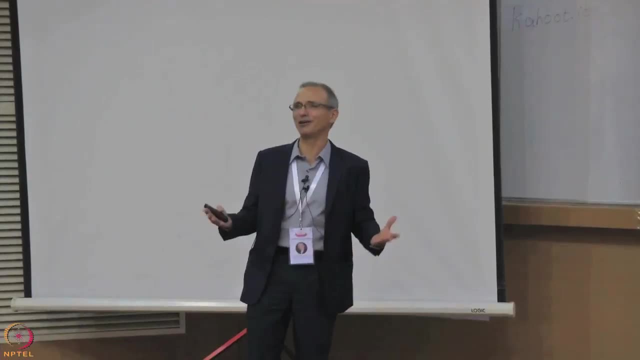 it being used. It is like developing a business, right? if you guys develop a business and if nobody comes to your store And actually uses your products, your store typically won't stay in business too long. So I am always paranoid, you know, are people going to use these materials? 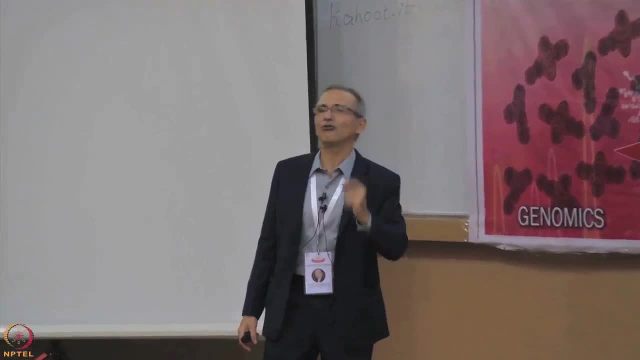 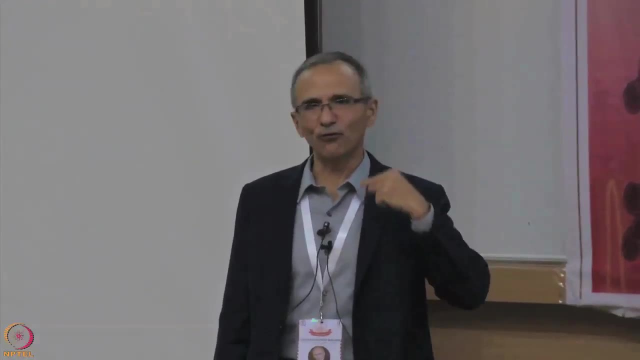 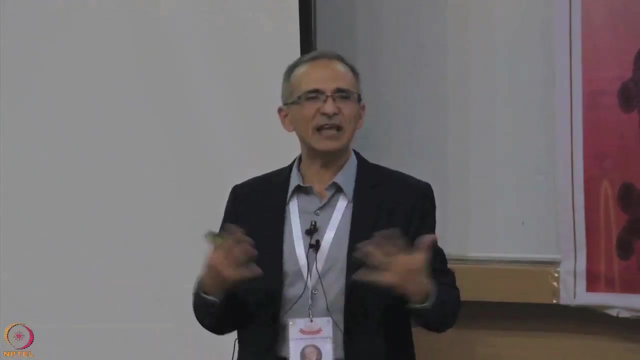 I would argue giving away your data and everything you find in a pre-competitive manner is truly advantageous, not for your own program but at the same time for the globe as a whole, For three basic reasons. one: if you give away the raw material- just data, sets, reagents, your 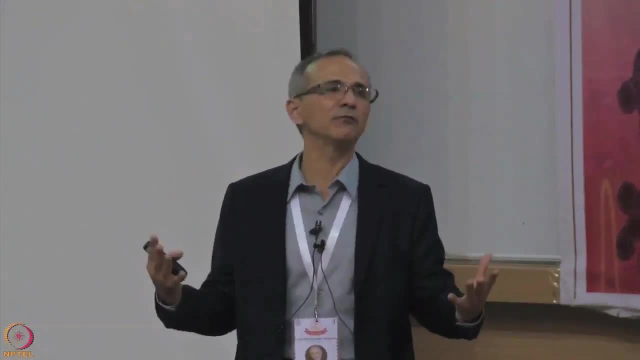 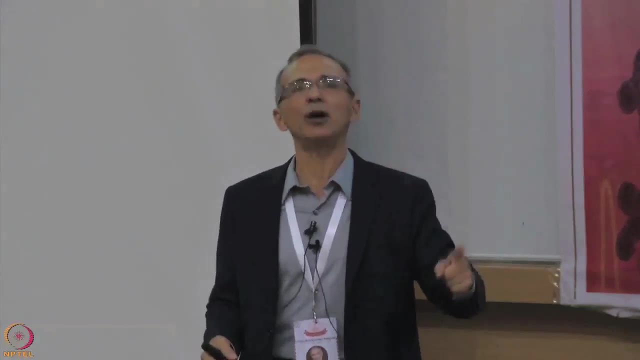 standard operating procedures. It stimulates outside individuals that do not have wet laboratories, that are computational scientists that could reanalyze your data sets and hopefully develop new hypothesis to pursue science in a way that you could not figure that out a couple of years in the past. 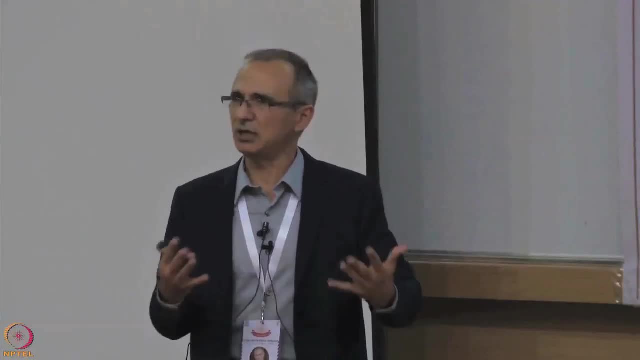 Secondly, if you could take your raw ingredients, work with industry to develop kits, you could further disseminate that to the public. And thirdly, you hope that some of these kits or the reagents, you could put them in a way together that actually could be used in a clinical setting. 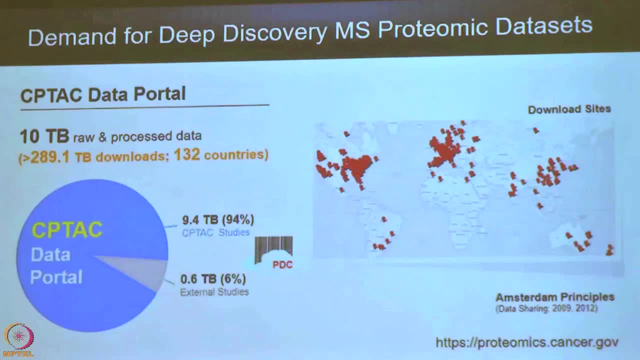 So let me give you an example of all three of them. So, in terms of our data, do people use the data sets of CPTAC? It turns out it does. it is very simple to get analytic metrics on it. So our program has about 10 terabytes worth of raw and processed data files available. 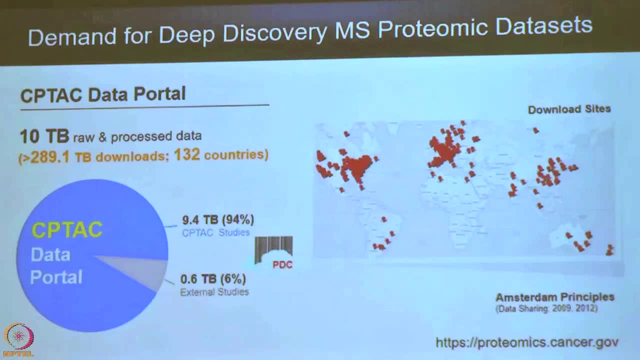 to the public. as of today, We know that our data is being downloaded all over the world, specifically just over 130 countries, And actually of the small little 10 terabytes worth of raw files that those downloads have now exceeded, So we will almost have reached 300 terabytes worth equivalent of our data sets. 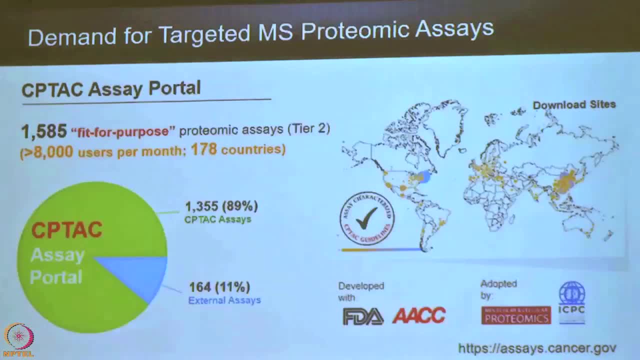 In terms of the other components that I talked about, we also give away assays for those targeted based assays that we develop. So we have a portal. we give away all the parameters behind the assays that we develop. We currently have just over 1500 of these fit for purpose based assays. 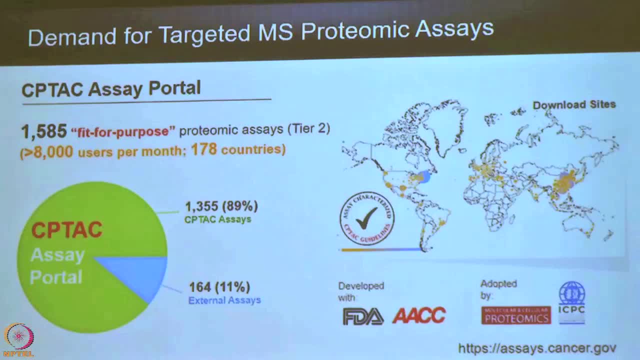 Do people go to our website? Yes, it turns out. on a monthly basis, over 8000 people are now going to our website and they are grabbing whatever information they want. They are actually conducting studies in their own laboratories and actually those download sites come from almost 180 countries. 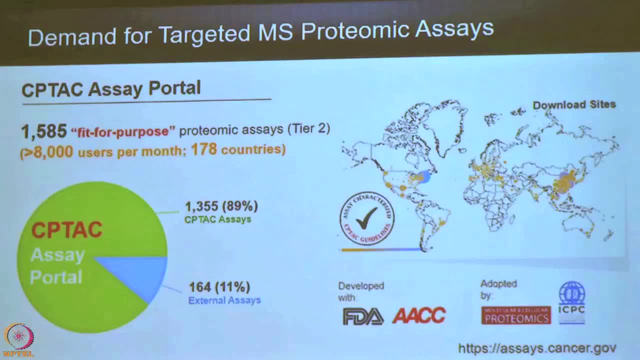 The vast majority of the assays actually do come from CPTAC, but as we develop these analytical criteria for the public, we are starting to allow outside investigators to deposit their own assays within our own portal. Now, some of these assays do require a higher level of sensitivity, if you want to measure. 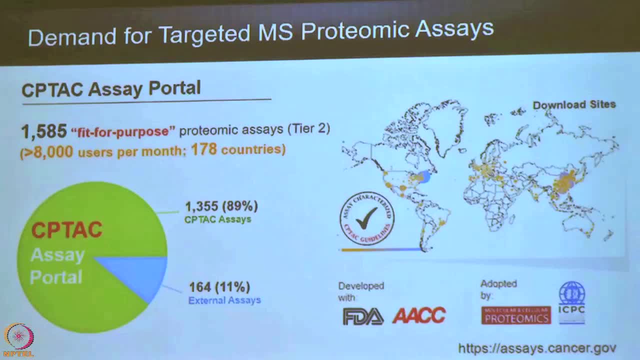 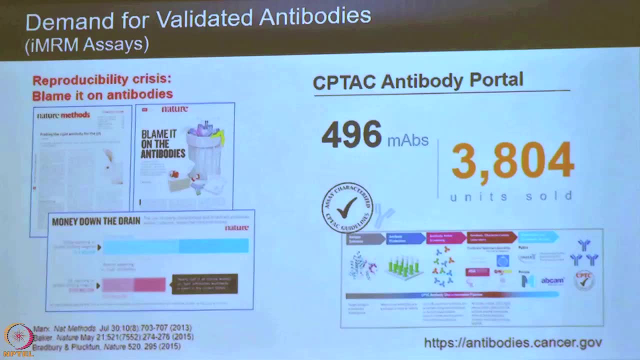 endogenous levels in individuals. So for that we do develop reagents. those are antibodies. So in antibodies, So in antibodies. So we have almost 500 monoclonal antibodies that we have developed and fully characterized. we give away all the characterization in the public and we give it away through different 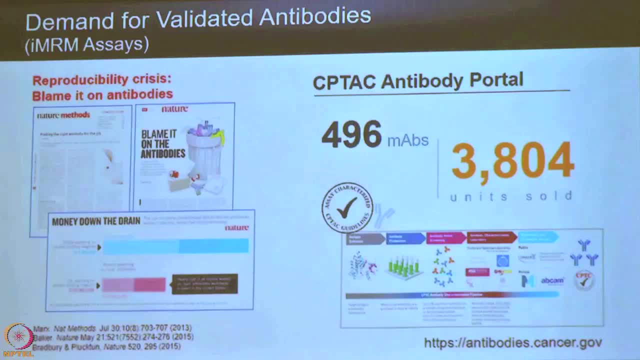 distribution arms One week. one distribution arm is at very low cost through the academic model and the other one is through industry and we have been able to sell these units. So we have now sold almost what 4000 units of our antibodies, which is really good for. 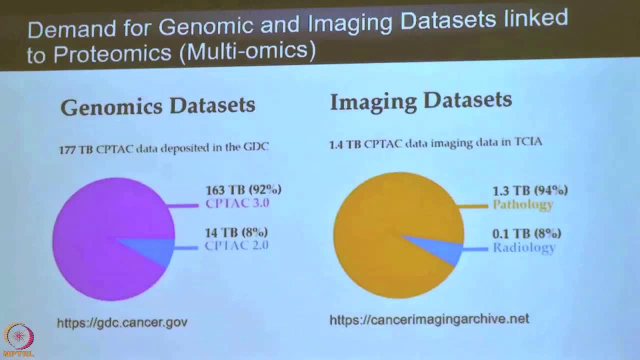 this little small program out of the National Cancer Institute. And of course we just do not do proteomics, We do genomics and isolation, we do genomics and we do imaging. So all the imaging that comes from the histopathology lab or from the radiology lab, we give it away. 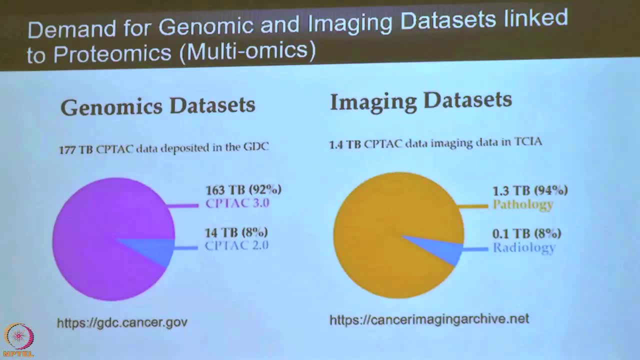 into the public domain. So it is not just proteomics. we do genomics, transcriptomics, proteomics and imaging- everything. we put it in the public. Now, another great example is this recent study. In fact, I ended up getting this paper from the director of my institute about a couple. 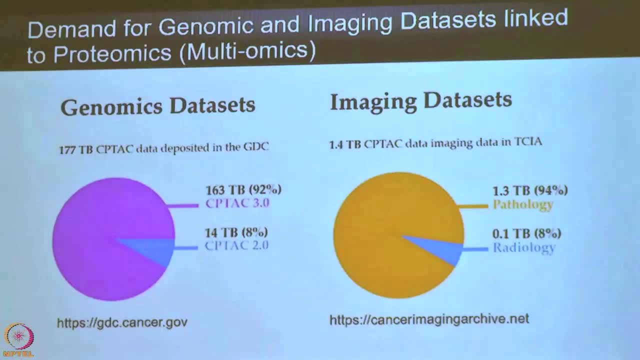 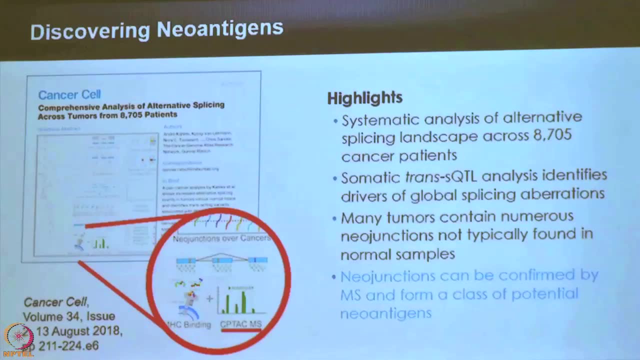 of weeks ago and his comment was: have you seen this? it was flattering that somebody else saw it and not me, And here is why It is a neat little study. So our program really was not looking at neoantigen. neoantigen is like this hot little. 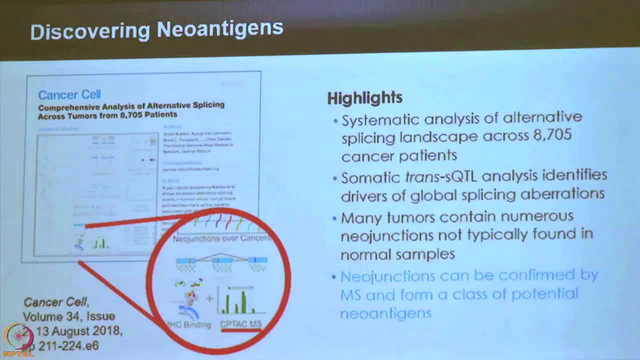 terminology that people use now, basically looking at mutated components. But at the end of the day, this study comes out in cancer cell in a late summer and what they looked at was neoantigens. but they looked at publicly accessible data sets, it turns out. 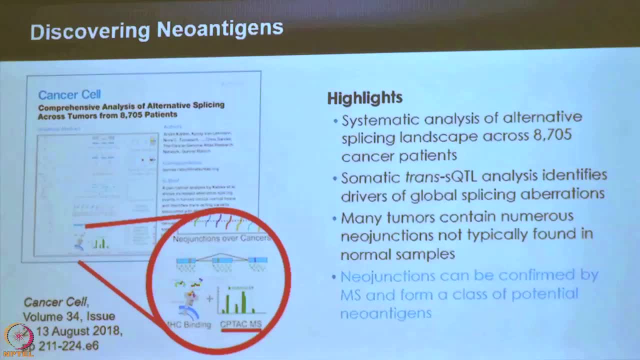 Obviously, the one that typically people will think about is the cancer genome atlas, but the part that I liked about it was is that on the front cover, if you look at the image that they had, The data sets that they pulled out to conduct their analysis actually comes from the US. 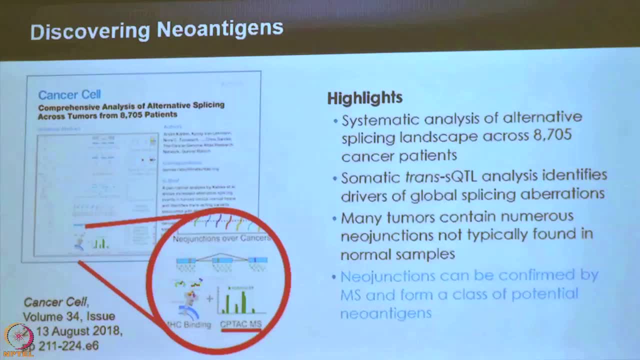 based CPTAC program. why? only because we place it in the public domain. So there is a great example on how giving up the information we never explored- neoantigens within our data sets. another investigator group is able to do it for us, and again it. 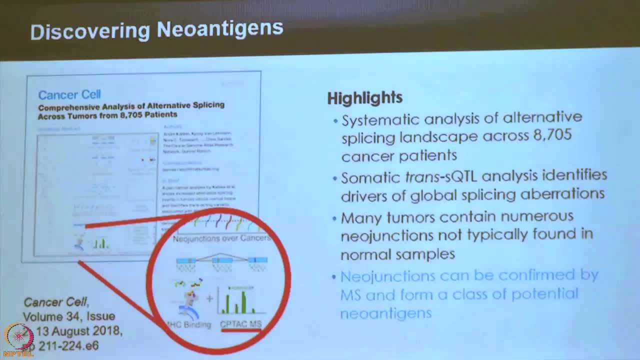 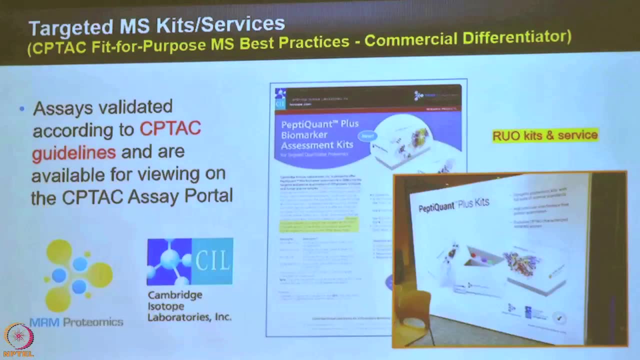 further stimulates the science world. Now, these are raw ingredients. what if you work with industry to develop small kits? So one of our colleagues is in Canada, MRM proteomics. So MRM proteomics develops kits and these are targeted based assays and one of the thing 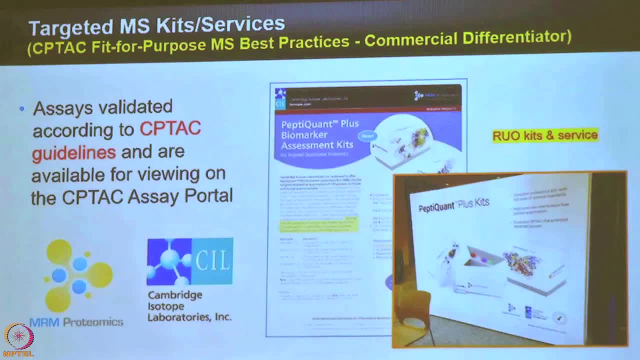 they wanted to know was: how do they differentiate themselves from other manufacturers? Our comment was: you might want to look at our analytical criterias and, if you are able to adhere to them, we will host your assays on our own portal. further drives traffic towards your company and at the same time, you put out a kit that has a higher level of standardization. 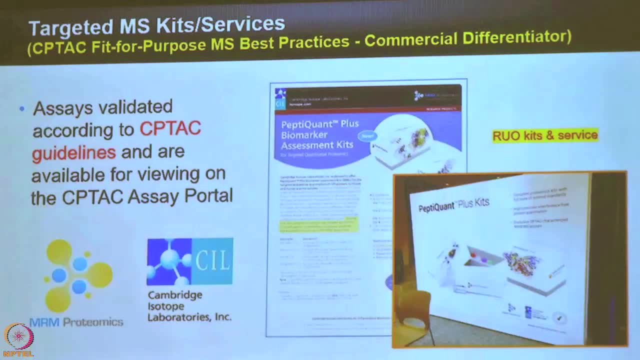 than typically what is out there within the research landscape, and that is exactly what they did. So when they now put out kits that they actually run it as an in-house service or the, you could actually purchase your kits and run it within your core facility. 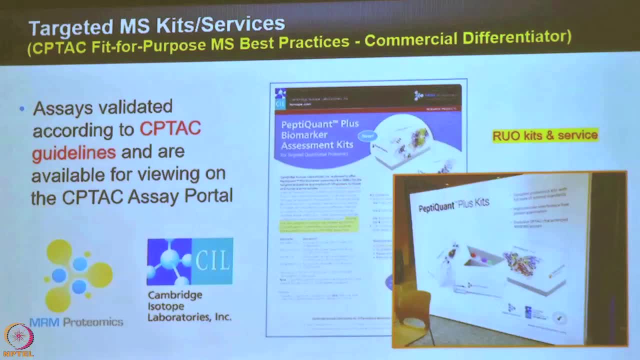 These are all research use only. right there, it will basically tell you that they adhere to the CPTAC guidelines for their analytical kits themselves. Now, this is still the research space. what about the translational space? and develop these targeted based assays? here is a great little study that actually came out, a couple. 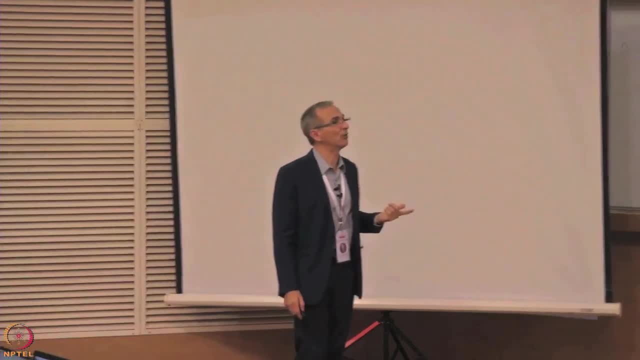 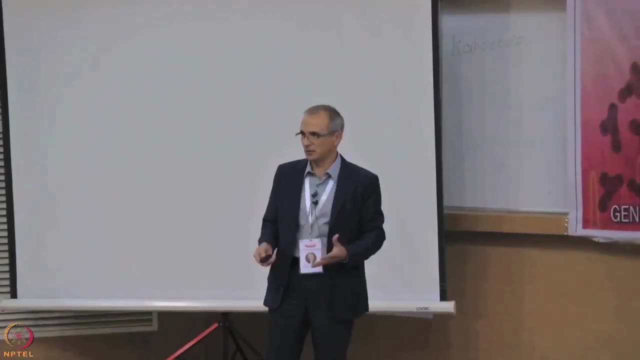 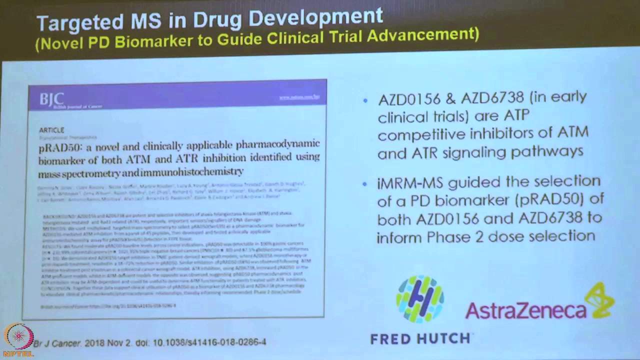 of weeks ago, and this is a partnership from one of our laboratories on the west coast That actually partnered with AstraZeneca, and here is a great example how proteomics helps the therapeutic side of the landscape. So in this one they were looking at is two compounds. DEs are basically tyrosine kinase. 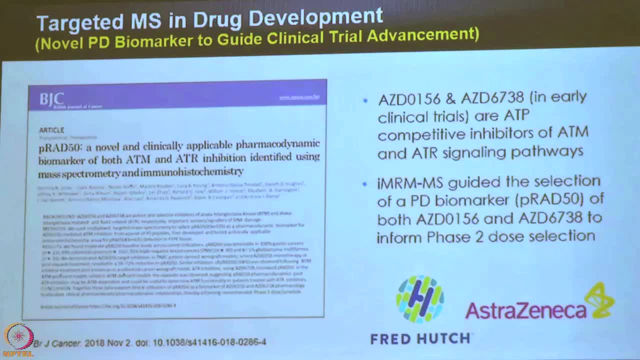 inhibitors and they are going after two pathways, ataxias that are. that has a lot of affiliation with DNA damage response. But basically this investigator, Amanda Polovich, at the HUD she developed a targeted based assays that looks at the DNA damage response. That was a huge success. 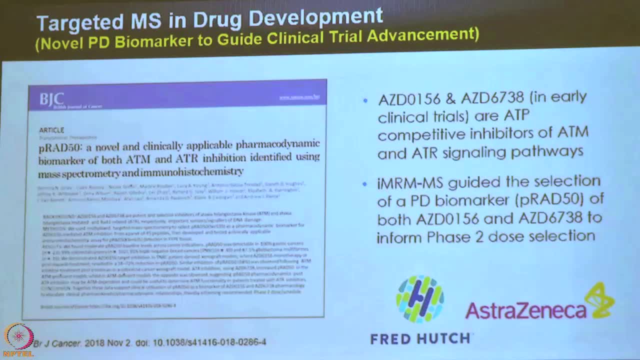 That was a huge advantage for AstraZeneca and in the partnership, what they ended up doing was they actually then identified a marker, and this is a pharmacodynamic marker. That PD marker actually helped AstraZeneca move these two compounds from a phase one. 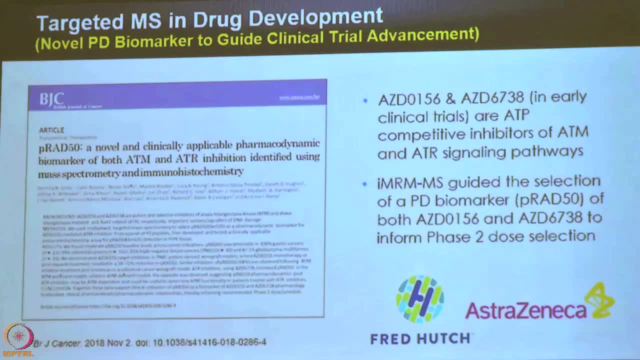 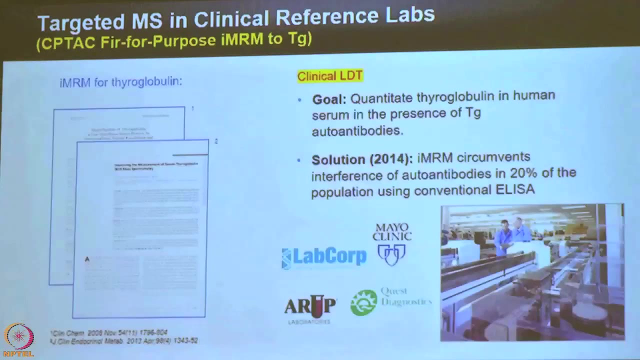 study, using now this PD marker and they are able to translate it into a phase two And it is being used to actually determine the dose that actually is going to be administered to these individuals. Now, this is still the translational space When you get it in a clinical environment. we have actually played in that space. 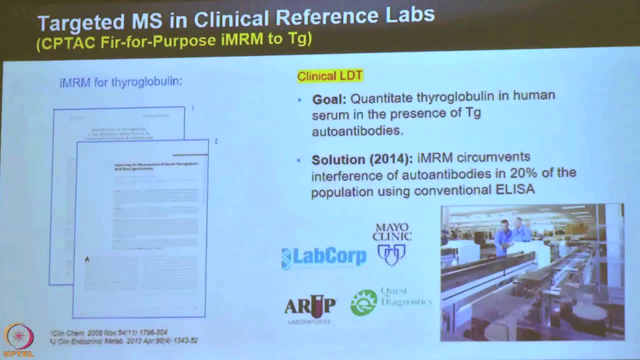 Here is one example. Now here is one where a lot of people try to find new biomarkers. but again, that is very complicated because you are trying to figure out new biology and, believe me, new biology towards patient care takes many years. but that is ok because biology is complicated. 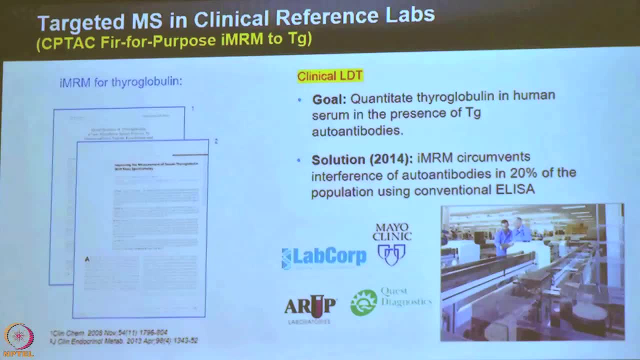 So we decided to do was to take the analytical techniques that we have developed and ask clinical laboratories: are there existing tests that are problematic? Yes, That might be alleviated if you were to bring this orthogonal measurement into your portfolio, and in this case they went after thyroglobulin. 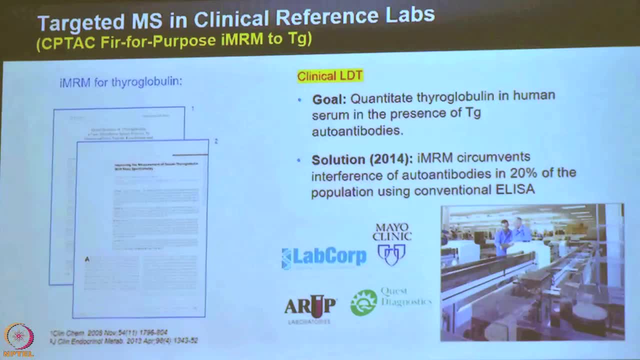 The reason they went after it is that you find out about 20 percent of the population individuals with thyroglobulin. they actually suffer from autoantibodies- The autoantibodies. the issue with that is that it is going to interfere with the secondary. 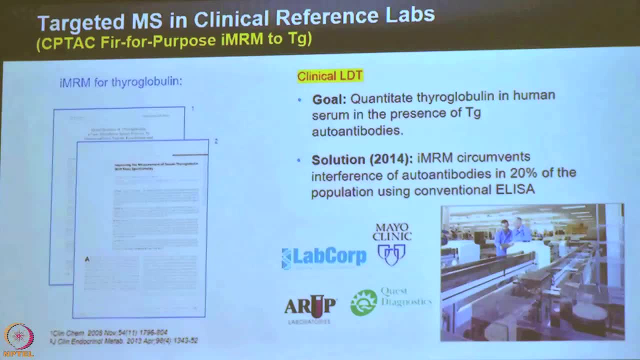 antibody of analyzer. So you get a lot of hook effects and basically you end up with false positives. So the circumvent the 20 percent of the population, 20 percent of the population. that is missing out on a very good test. we, actually, our investigators- 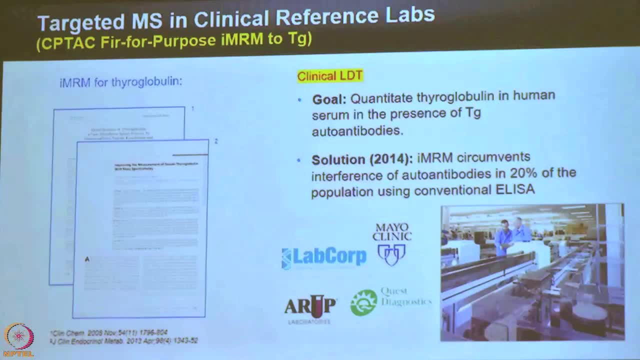 ended up developing a targeted mass spec assay dedicated against thyroglobulin itself. That test today now is being used by every major clinical reference laboratory in the United States. Now this is still being used as a laboratory developed test. What if you wanted to take it to the FDA and get something approved? that is a whole regulatory. 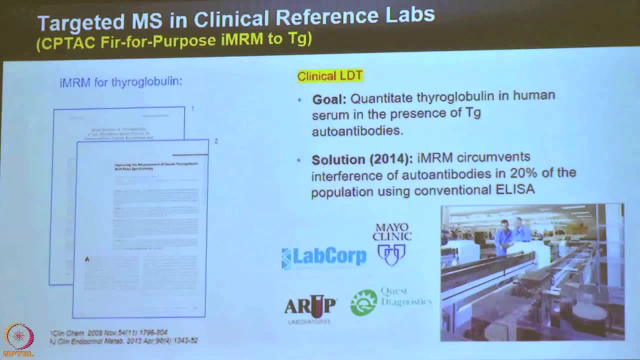 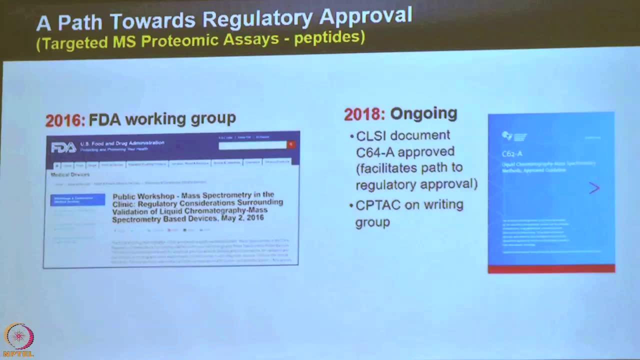 path. Well, that is an interesting space. So this is what our investigators are now doing within this environment. It turns out when you go directly back to the FDA they will say, well, mass spectrometry, we do not develop the standards or we do not tell people what to do. 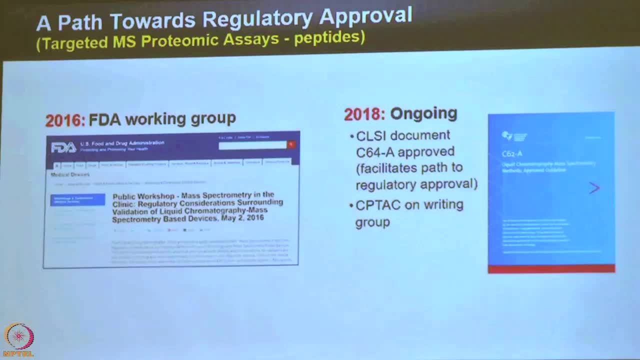 We look at the community to come up with a consensus document. once we understood the process, we said: So what is one of the communities you look at? it turns out there is an organization referred to as CLSI, which is the which is the clinical laboratory standards, institute aspects and 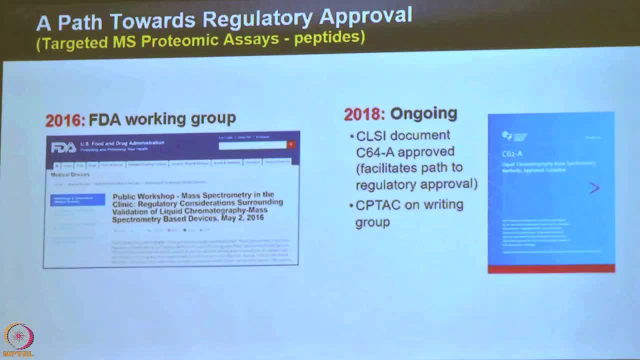 what we ended up doing was the following: In 2016, we worked with the FDA to put on a workshop dedicated toward mass spectrometry- not again, not mass spectrometry for metabolites, but to move it into the measurement of this. in this case, your measurant was going to be a peptide. 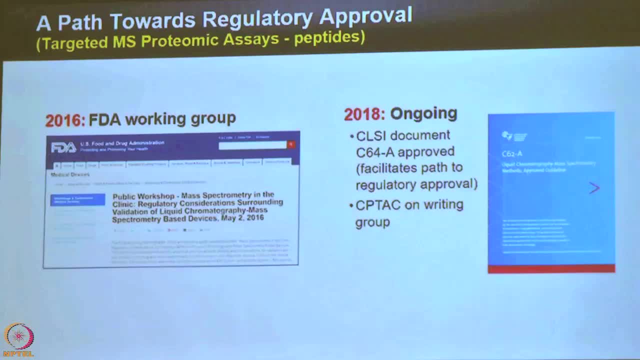 That that ultimately then led in early of 2018 to an existing governing body of CLSI. So they have always had, historically, a document referred to as C62A for using mass spectrometry in a clinical setting For the measurement of metabolites, but not for peptides. we are now working with them. 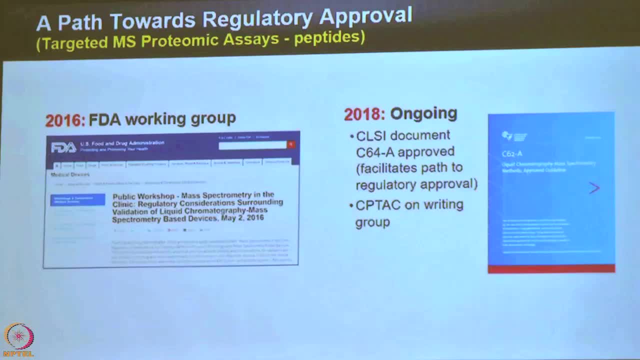 to develop one dedicated to the measurement of peptides, and the goal is, hopefully, within the year 2020. it takes a lot of time, apparently, but in 2020 they are going to be released a document that is dedicated for the measurement of peptides, which is a law, which is basically. 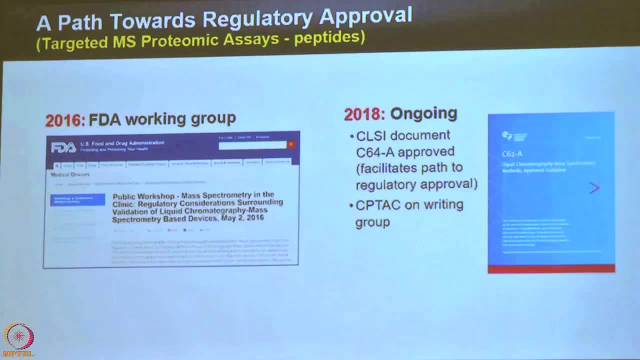 the targeted mass spec that a lot of people have been referring to. Now the other question I get is: well, are these technologies very specific to cancer? It turns out they are not. The methodology is ambivalent. that is the beauty of it. So here is a great example of it. 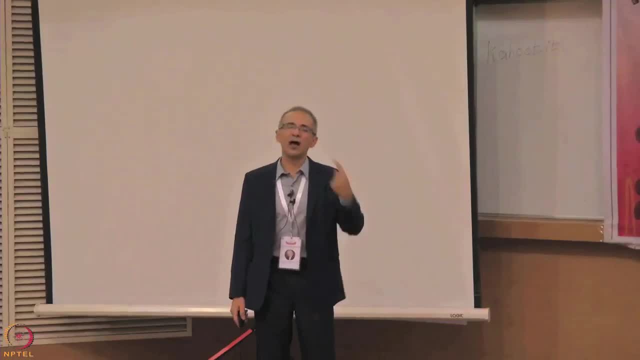 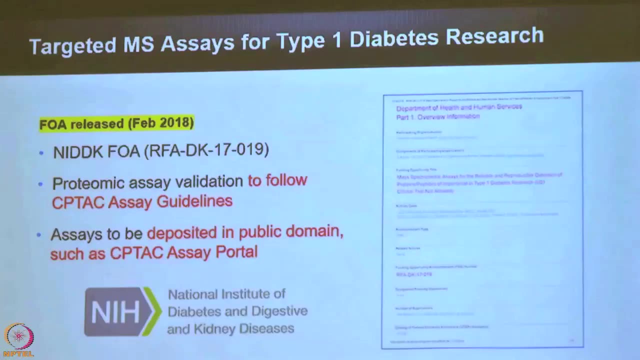 So at the National Institutes of Health- I belong to the National Cancer Institute, One of my sister institutes, the National Institute of Diabetes- they basically put out a funding solicitation early this calendar year. The reason I loved it was the following: when we found it they talked about is that they 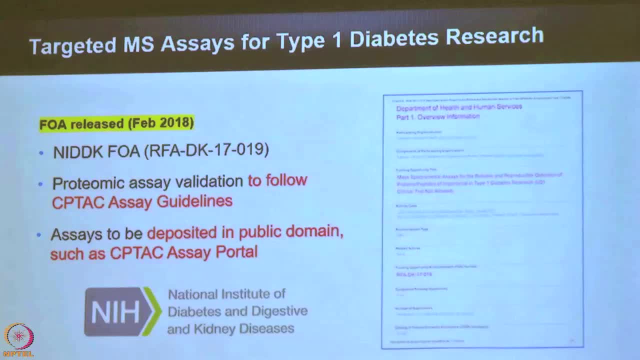 said they are going to be funding laboratories in the US to develop targeted based assays against, I believe, type 1 diabetes. Yes, but that is not the part that is interesting is taking proteomics into diabetes. The part that we like the most was- they basically said it- when you develop your targeted based 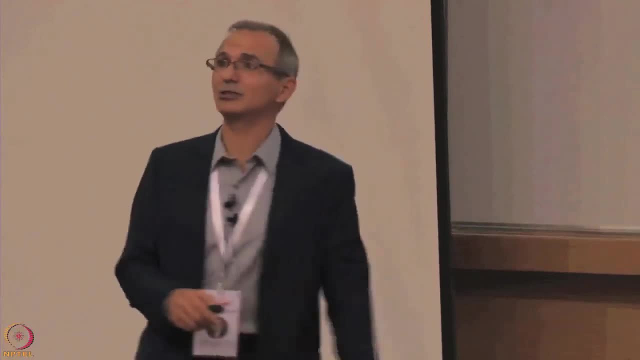 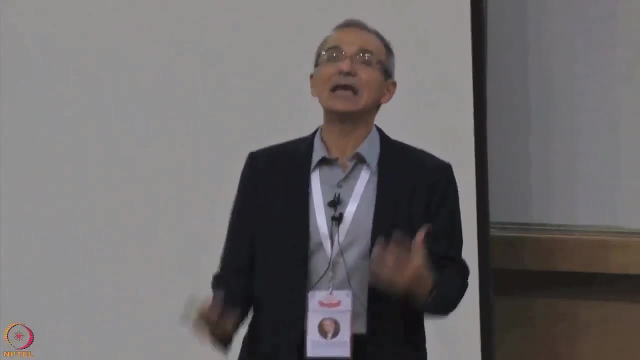 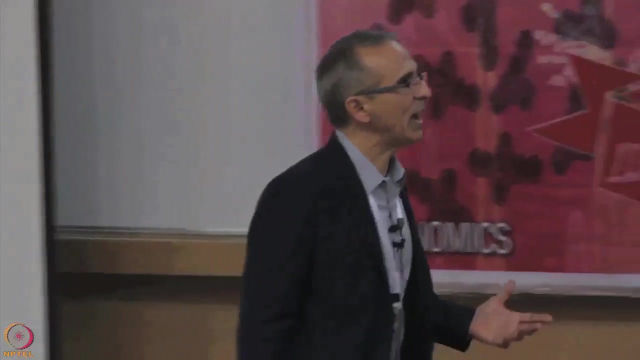 assays, you have to adhere to the guidelines developed by the National Cancer Institute CPTAC program and, more importantly, you have to deposit the analytical criterias of your assays in the public domain, So it sets a precedent for other people to be replicating that process. 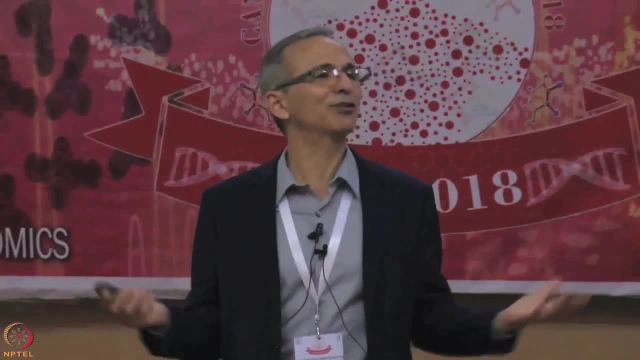 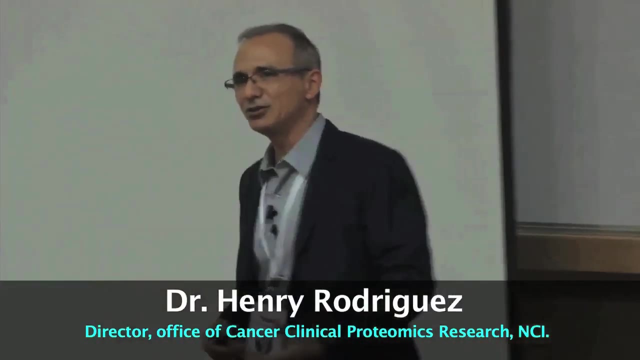 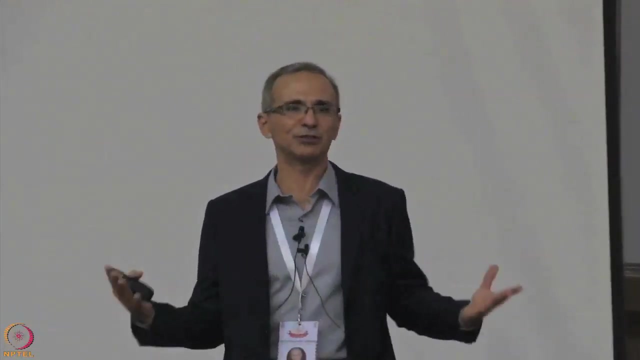 Now CPTAC. I pretty much do not do anything. I have to admit. I have the pleasure of being at the National Cancer Institute and overseeing this effort. This is really a team based program and this involves multiple institutions within the United States- Just a series of incredibly talented scientists. it has been one of the most privileges I have. 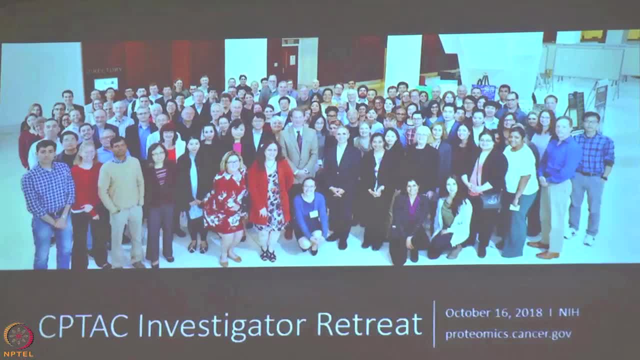 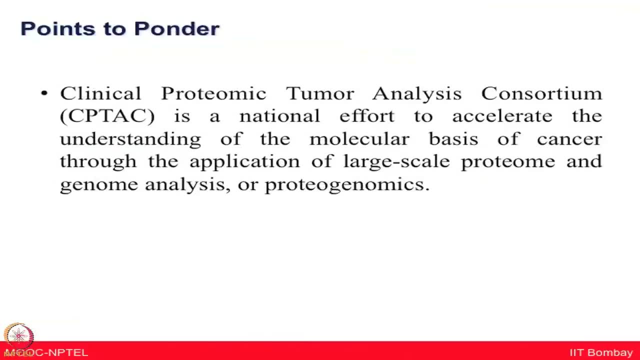 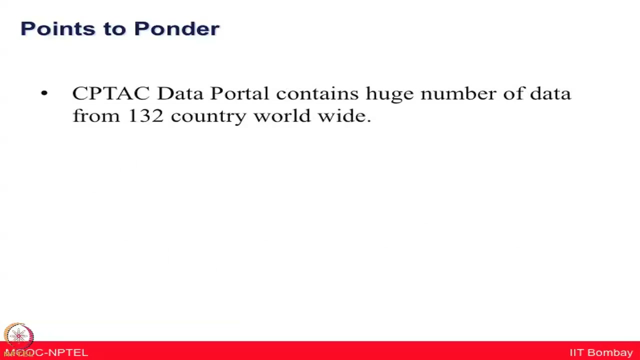 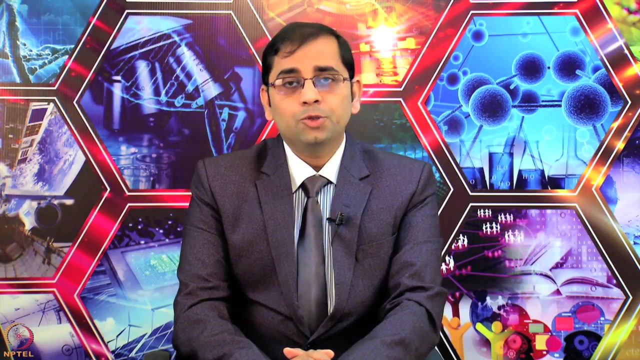 had over the past 12 years, But now this program actually has spawned this other sorts of initiatives of blending these two worlds together. I hope, after listening today's lecture, you are convinced that, whether to choose genomics or proteomics, which one is better? 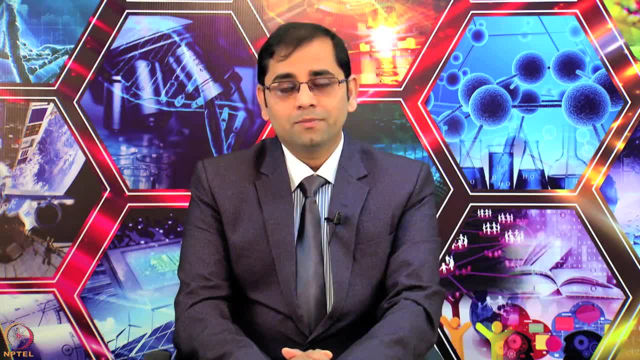 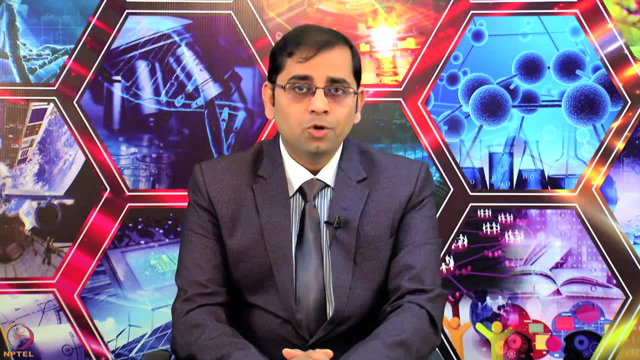 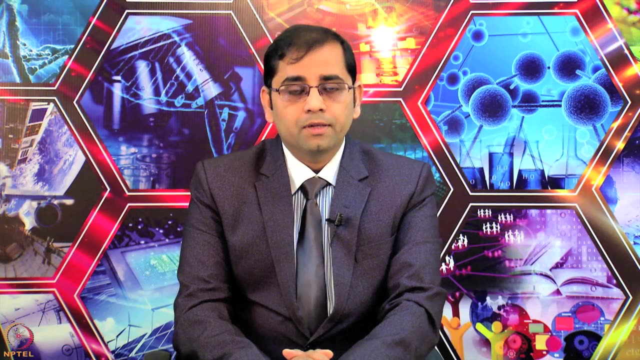 Probably genomics, Yes, Probably. you will not ask this question anymore and you will agree that both of these technologies are good, but probably a good integration of proteogenomics could provide us much more meaningful information. Dr Rodriguez provided very good example that if you open a biology book, what you find? 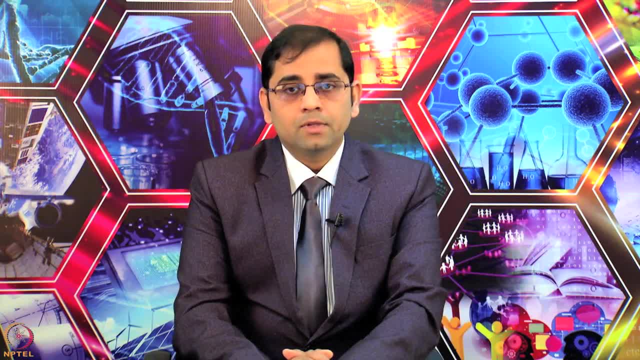 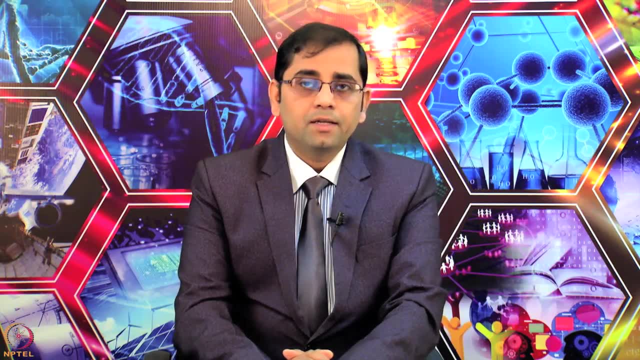 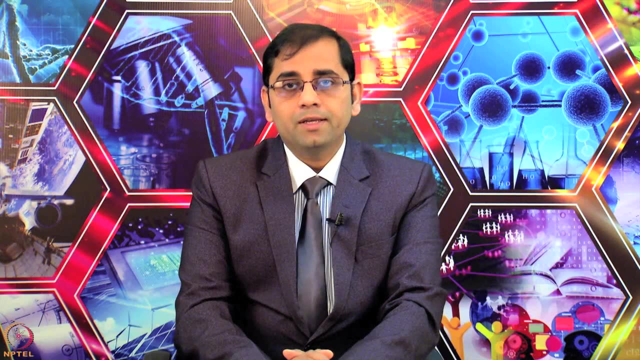 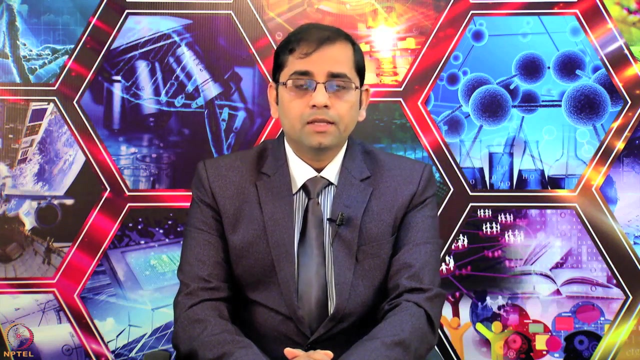 is the correlation which defines the complexity. So both genomics and proteomics need to be understand thoroughly so that we can understand important correlations. That means we all need to focus on the new area, which is proteogenomics. I hope you also heard various pathway networking correlation in the ovarian cancer project.